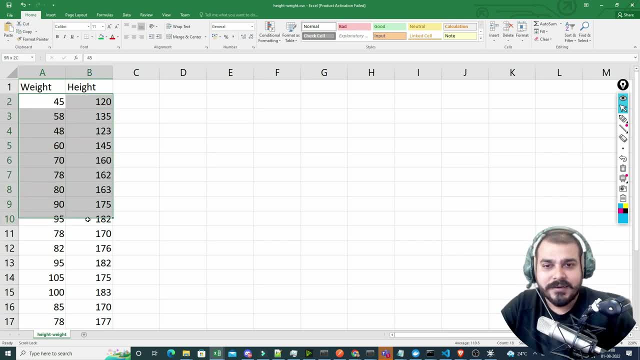 And here you can see, based on some weight, there is some different heights, right, And this is my entire data And I've just taken 24 records. In short, I've just created this data set by my own And what we are going to do is that, on top of this particular data set, we'll try to apply a simple linear regression. right, And why do I say simple linear regression? Because I just have one independent feature and one dependent feature. So here, weight is basically my independent feature And since I need to predict height, this is my dependent feature. 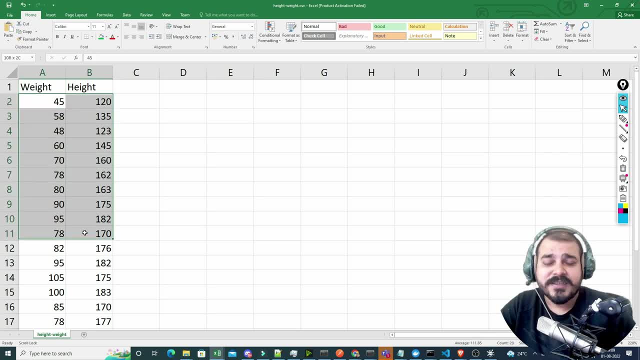 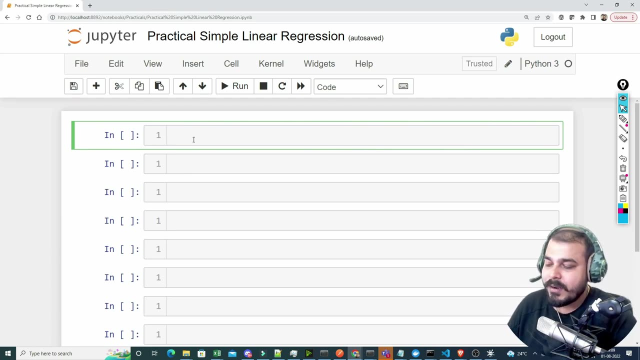 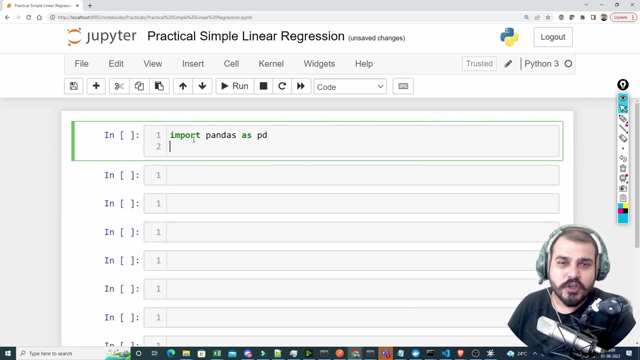 Now what I'm actually going to do over here is that I'm going to take up this specific data set and we will try to implement it with using a scalar. So let's go ahead without wasting any time. So here it is. I'll just open my file. So the first thing is that we will go and implement or import some of the libraries, right? So first of all, I'm going to import pandas as pd. Pandas is a library which will actually help you to read the data set from different data sources like Excel, CSV sheet or other. 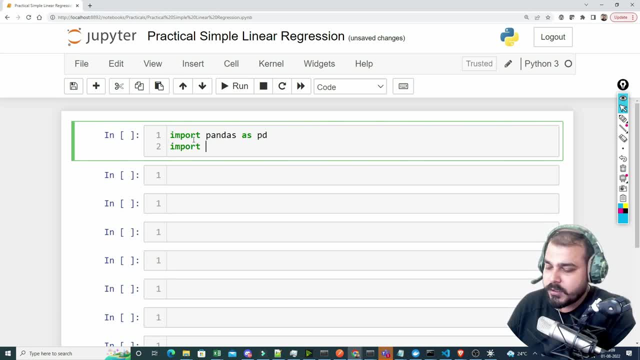 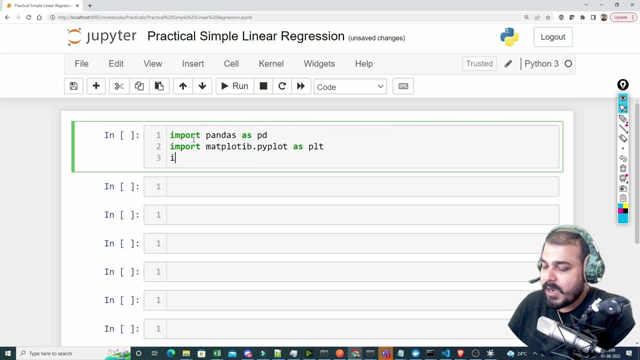 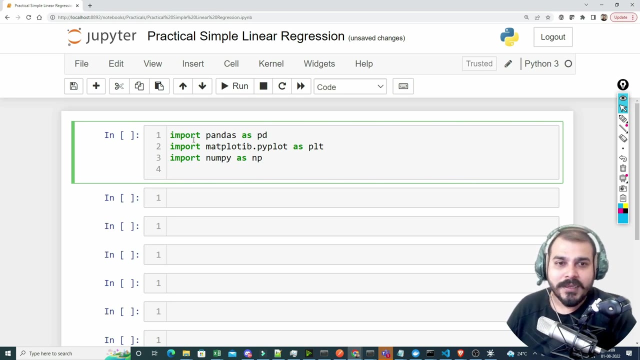 Right, And then I'm also going to import matplotlibpyplot as plt. This is for visualization purpose. Apart from this, I'm also going to import numpy as np. Okay, And guys, please remember one thing that if I probably make any mistakes, right, I will not, you know, remove that part of the video. The reason is that I really want to keep all the things in this particular video should look like raw, because 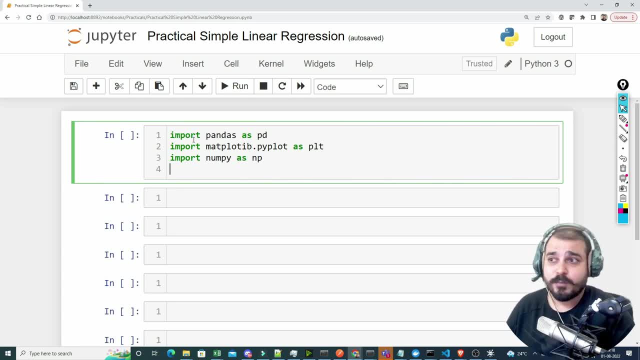 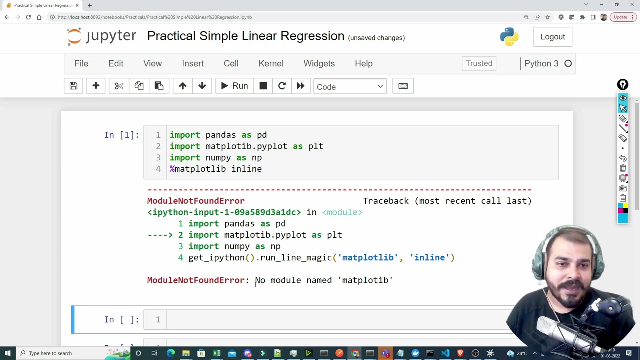 whatever issues you are going to face, it is better that we fix it in front of you, because tomorrow you may be also facing that particular issue. So just a reminder, Okay. So next thing, what I'll do? I'll do matplotlib, And then I will also say inline, so that I can display all my visualization graph within this Jupyter notebook. So let me just go ahead and execute. So here it says: first: error: no module named matplotlib, inline, Right. So here, if you see, what did I import? Import matplotlibpy. 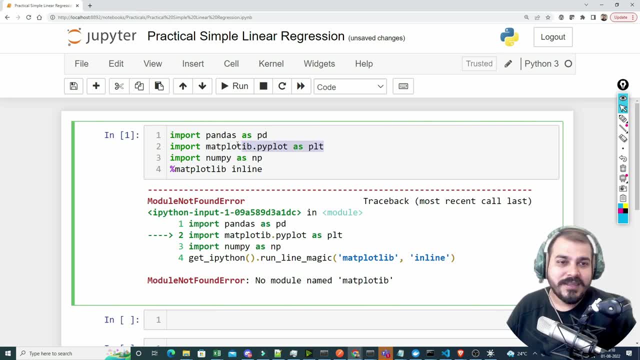 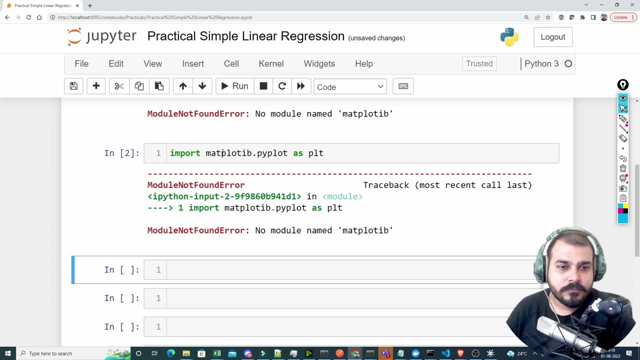 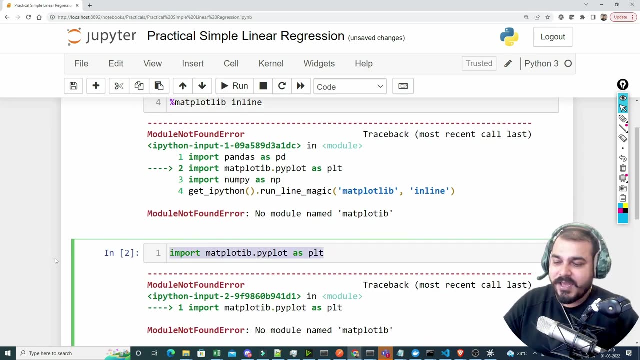 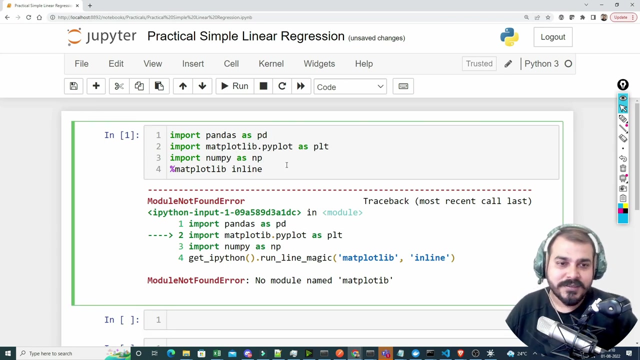 As plt, Right? So let's see why this thing is not executing. Okay, Import matplotlibpyplot as plt. Because here you can see clearly I have made one spelling mistake. So that is the reason why I'm saying you, even though I face any kind of issue, I'm not going to remove any part of that, So I'll make it matplotlib. So this is the. this is the spelling mistake was there in this library, So you may also face it. So I'm just going to execute. 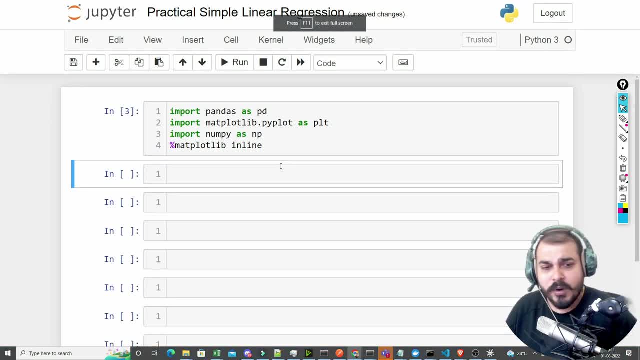 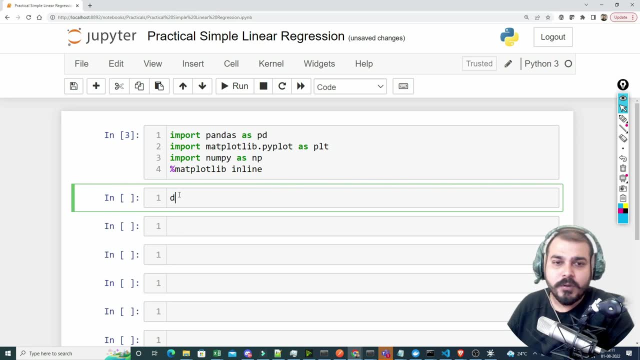 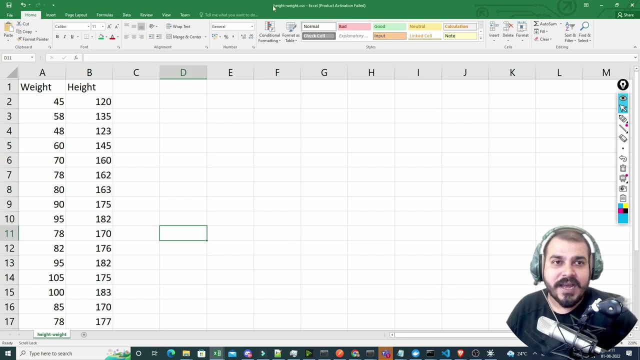 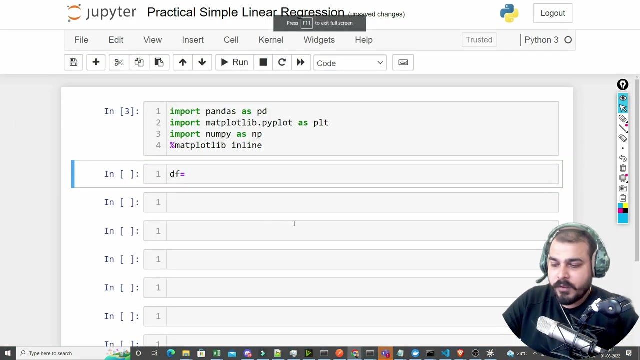 Execute it now. Now, the next thing is that what I'm actually going to do here is that I will be using- I will be reading the datasets Now to read the dataset. what I will do, I will write df And let me just open the dataset over here, And here you can see the dataset name is height-weightcsv, And this is present in the same folder location where I'm actually working. Okay, So let's go ahead and read this dataset. So I'm going to write pdread underscore csv. 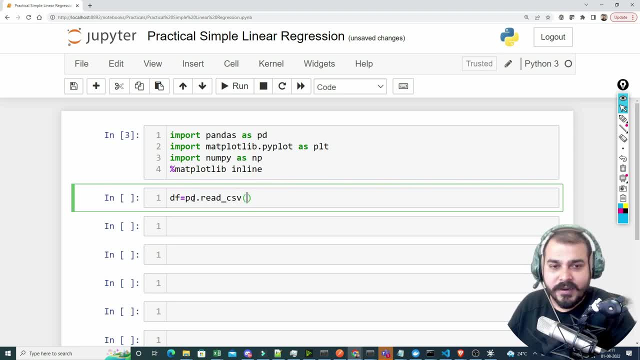 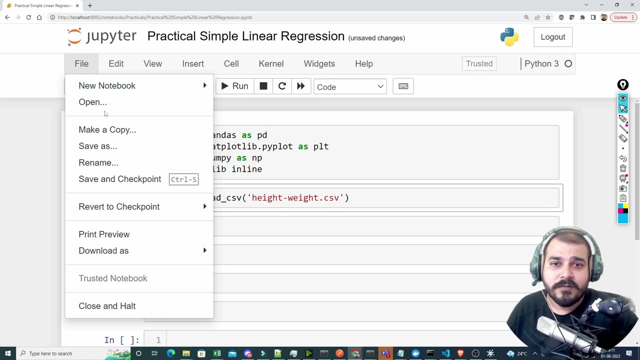 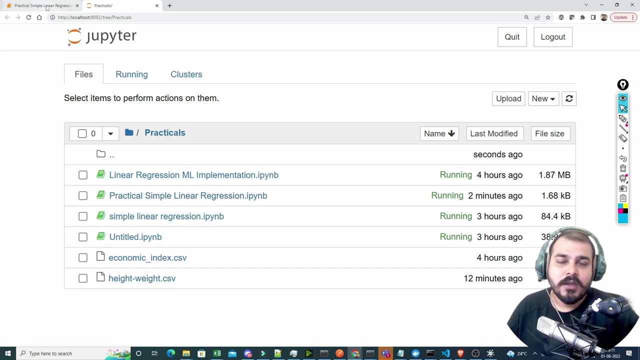 And here I will be reading my dataset, and my dataset is nothing but height-weightcsv. So if it is already present in this folder location, if I probably go and click on file and open it, right, you'll be able to see this particular file. Let me just show you So right now. this are all the files that are created inside this, And here you have height-weightcsv. Okay, So if you are starting this project, after you download the file, you know, please make sure that you keep that particular file. 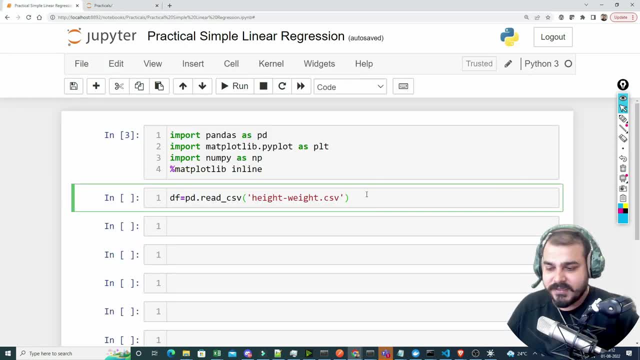 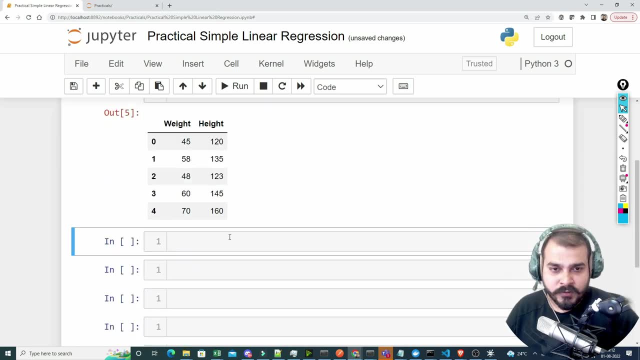 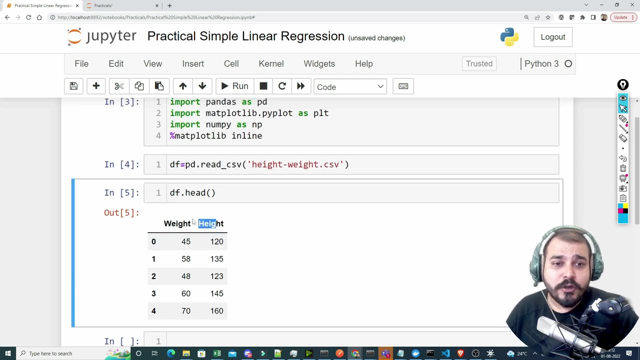 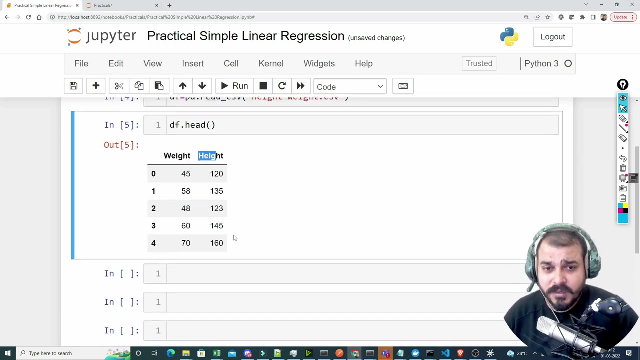 particular files on that same location. Okay, Now, once I execute this here now, I'm going to get something called as dfhead. If I see dfhead here, you'll be able to see here you'll be able to see two in one: inputs and one output, that is, weight and height. So these are my two features that I'm going to use And I'm going to probably create a simple linear regression. Now, first of all, one thing that you really need to understand: what is the relationship? 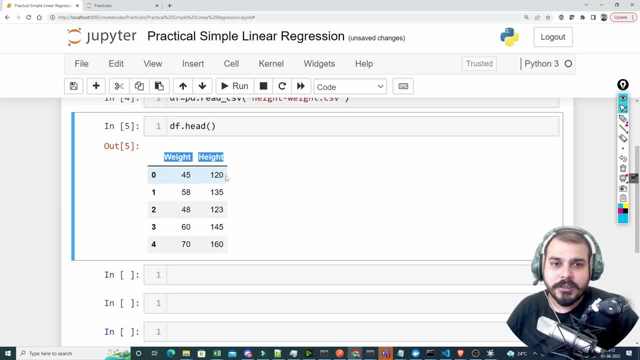 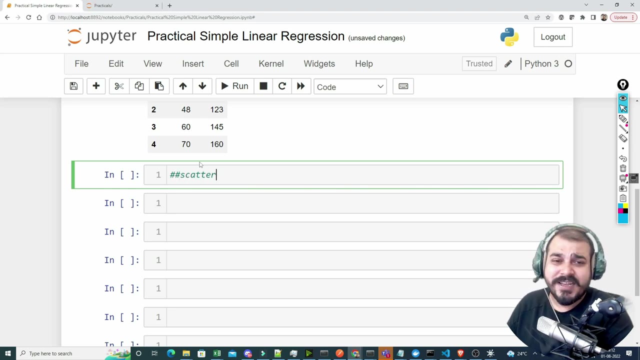 between weight and height. Whenever you are probably creating a simple linear regression, it is very much important to actually check how your independent and your dependent features are related, whether they are correlated properly or not. Okay, So one way is that I can use some scatter plots. Okay, And here I've taken a simple dataset. guys, You may be thinking, Krish, why you're not doing feature engineering. Is there any nan values you have to check or not? Yes, obviously you need to check, But I know in my dataset I don't have any other problem. And this is the first simple 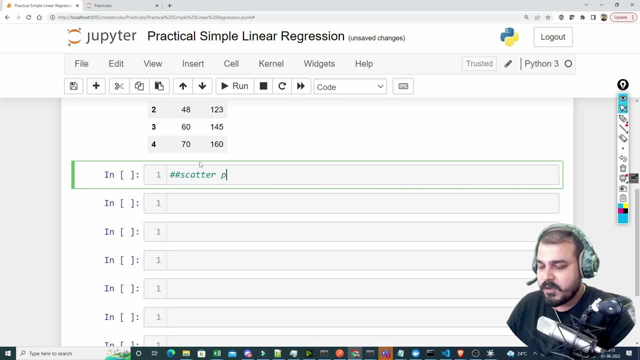 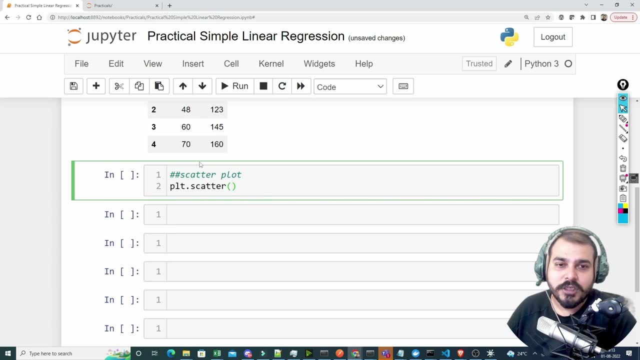 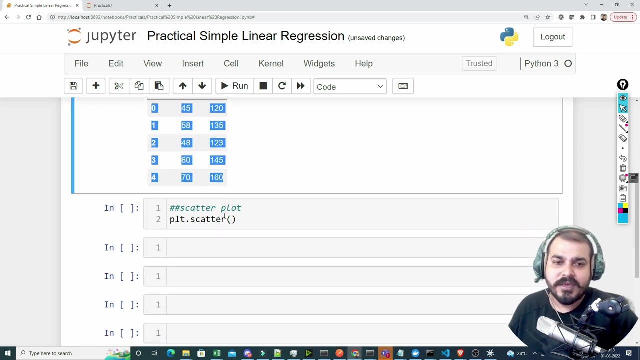 project. So I really want to go ahead and show you most of the important steps. So first of all, I will go ahead with scatter plot. In scatter plot I will be using pltc scatter. So scatter is a function which will actually help you to project your data points with respect to x and y axis, that is, your weight and height. So I just want to see how, what kind of relationship is there when we scatter the data points? So here I'm going to use df of weight And then I'm also going to use df of height. 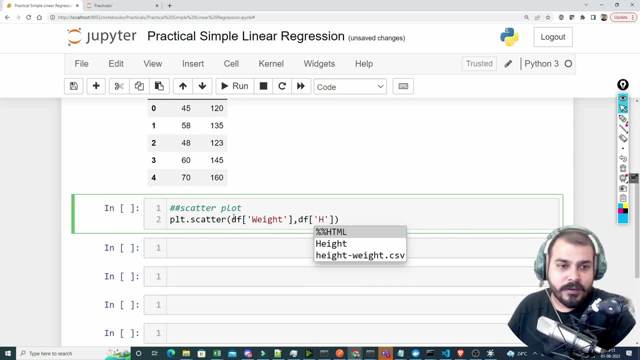 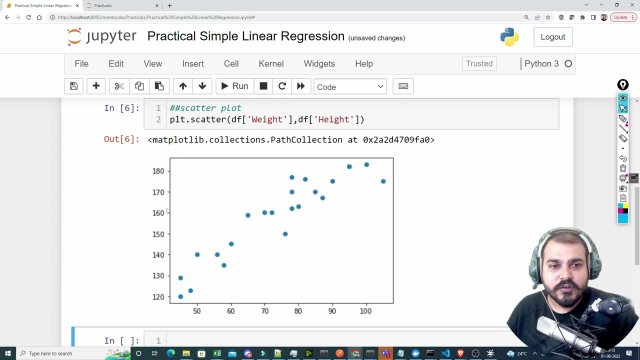 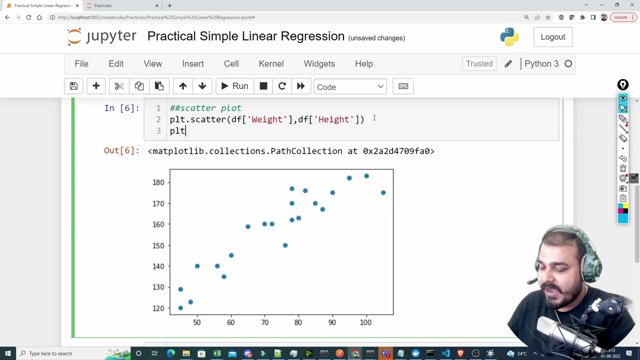 Right. So height, I think it is capital. So height. Now when I display this you can see that over here right In this. if you see the specific plot here, you can see on the x axis I've taken df of height right On the y axis I've taken df of- sorry. in the x axis I've actually taken df of weight. In the y axis I've actually taken df of height. Now let me just put some axes also. So I'll write pltx label, Okay, And I'll 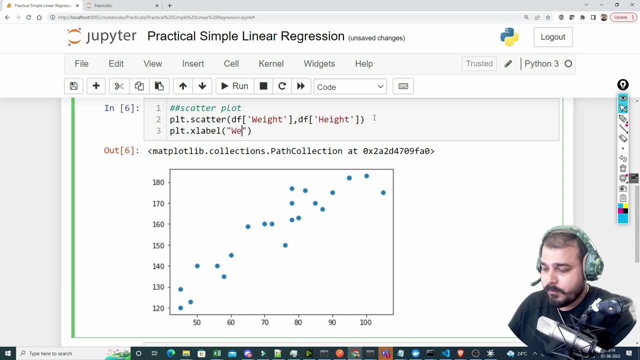 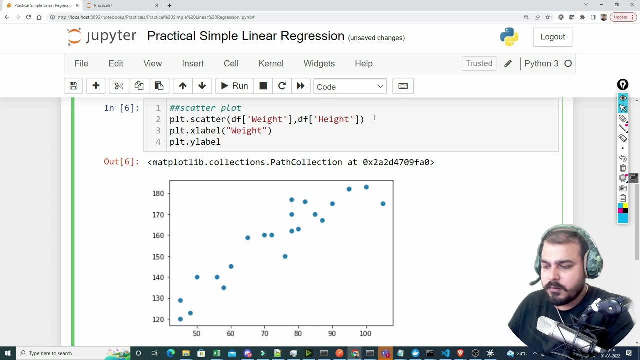 Here I'm basically going to put it as weight. Well, I'm just labeling the X and Y label so that it'll look better for you. PLT dot Y label. and here is specifically my height. okay, Let's go ahead and plot it now. here you can see that in the x-axis you are able to see height. 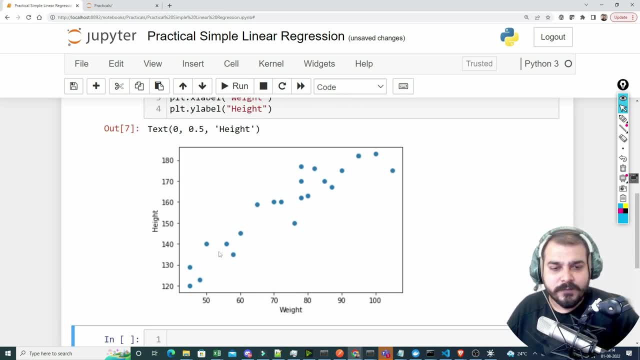 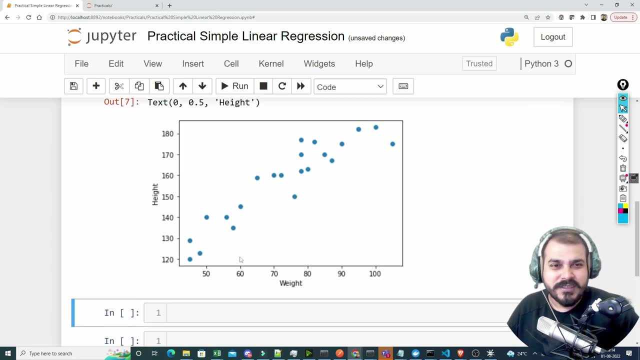 Weight, and here you are able to see height. Okay, Now, this is perfect. Now, from this particular data point, you can obviously see that as the weight is increasing, right, Your height is also increasing. So this is a kind of linear relationship, right? 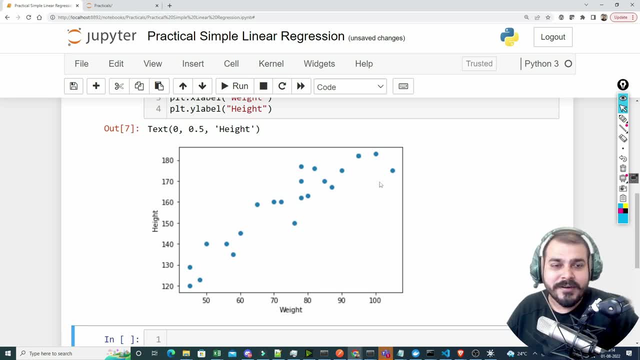 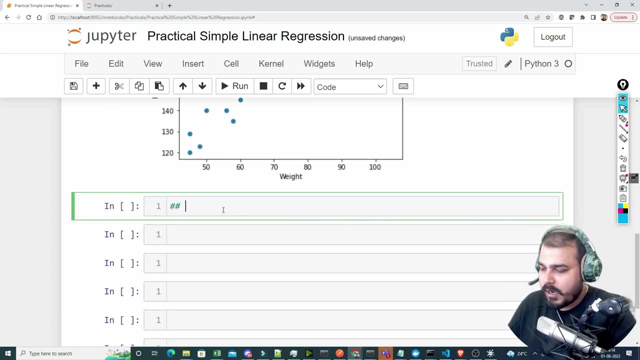 And if you really want to find out whether this really, whether this relationship, is positive or negative, you can also use Correlation right. So what I will do, I will just write over here of Finding correlation right. So if I write DF, dot C or RR, right? 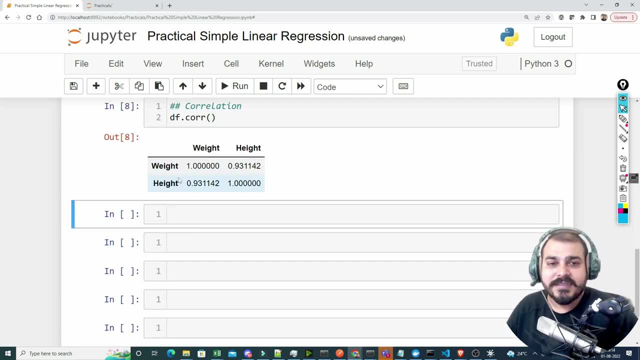 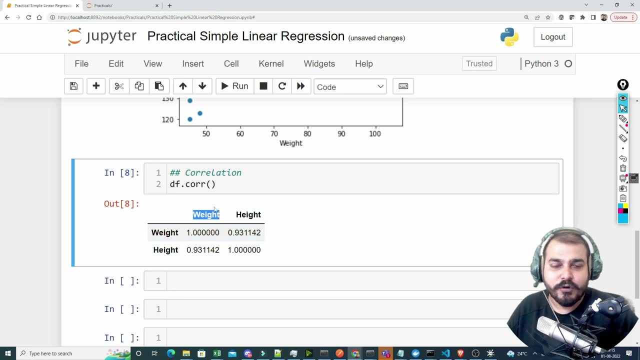 This basically means it will show you the correlation between your X and Y Coordinates, that is, your weight and height. now, here you can see within weight to weight, right, They will hardly be any variance, right, if you try to compare. so this is 1.0. 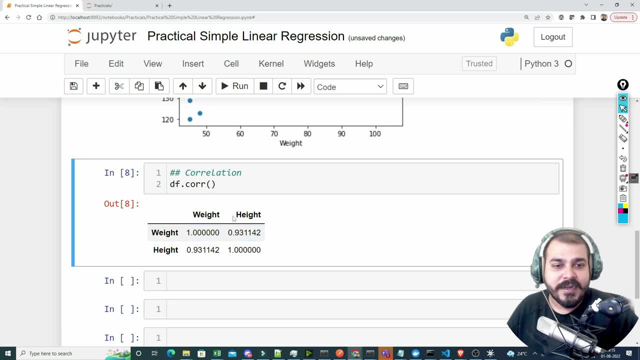 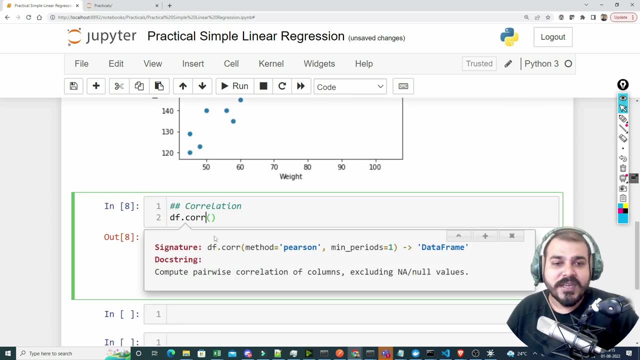 But if you see, with respect to the relationship between weight and height, It is 0.93. that basically means that it is highly positively correlated, because inside this correlation, If I go and press shift tab, the method that is used is something called as Pearson correlation. Okay, Pearson correlation and this Pearson correlation basically finds out the relationship between your X and Y coordinates. 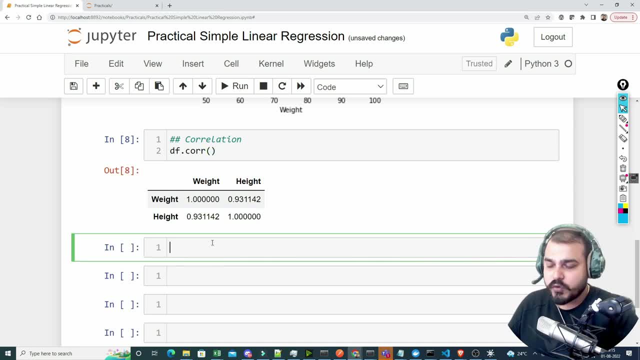 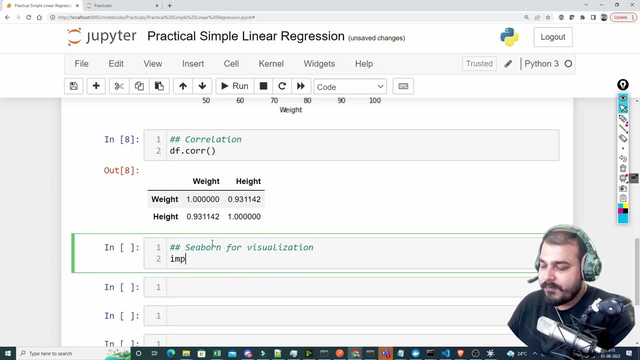 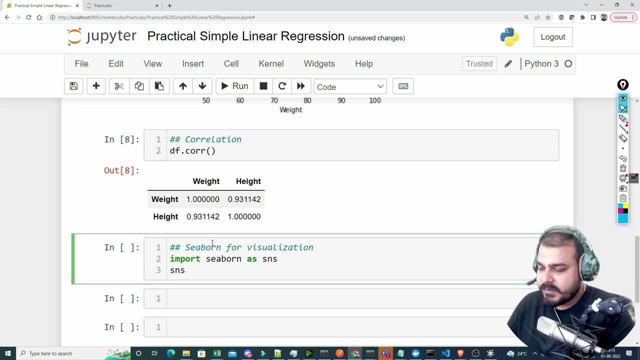 Okay, Now, this is perfectly fine. You can also use one library, which is called a seaborn, For visualization. So let me just show you that, first of all, what I'll do. I will import, see, but as SNS, right, and Here you can write: SNS dot pair plot. 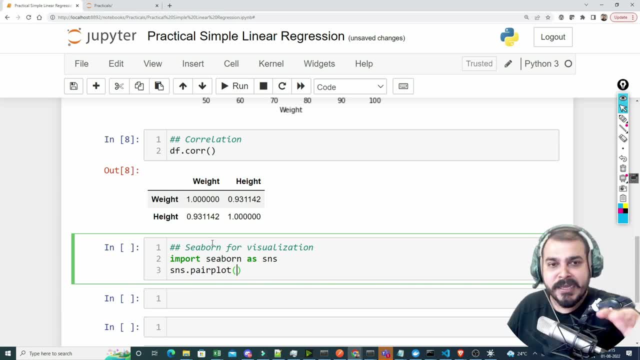 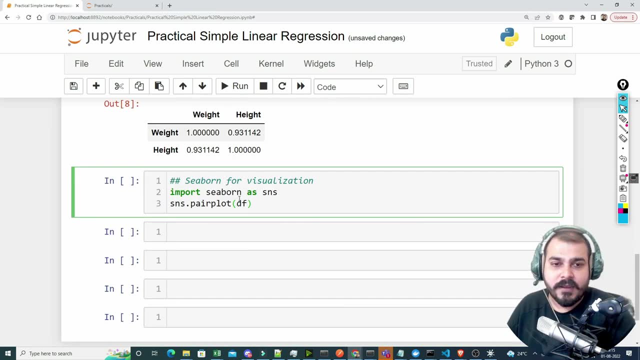 Okay, Now this pair plot. what it will do is that in a diagrammatically way it will try to show you, it will try to Display this specific coordinates. Okay, So here I'm just going to write DF And just execute it. So here you will be able to see. the same correlation is basically displayed over here. 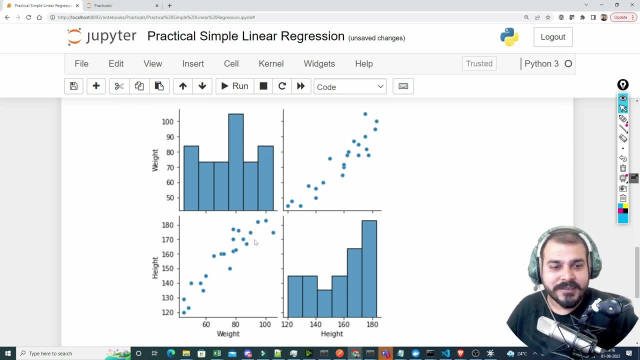 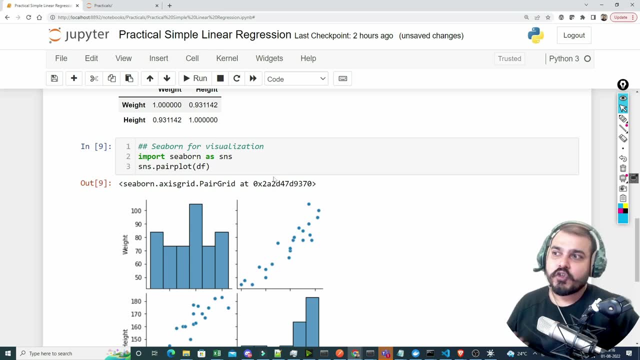 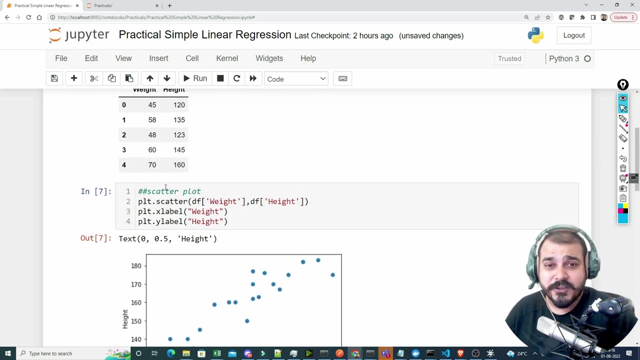 Right, and obviously height and weight is positively correlated. It is in a linear correlation and this is also in a linear correlation. Now suppose if you have something in linear correlation, you get a strong feeling that, yes, linear regression is going to work. Well, yes, there may be other problems with respect to the independent feature, Like usually when we do multiple linear regression. right, 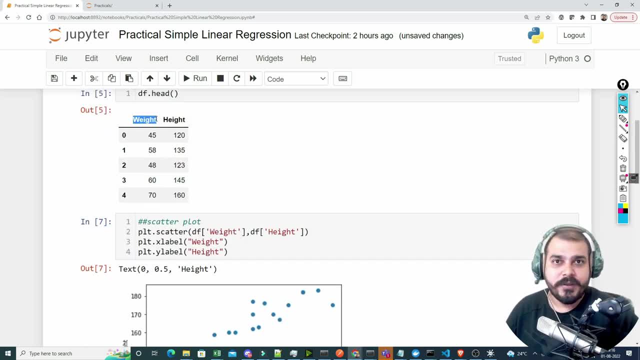 We also check this relationship between the independent feature. Right, but right now I just have one independent feature. We will. we'll get to know that how to check multicollinearity and all multicollinearity is a scenario Wherein if you have two to three independent feature and the correlation between those independent feature are high, then we can neglect. 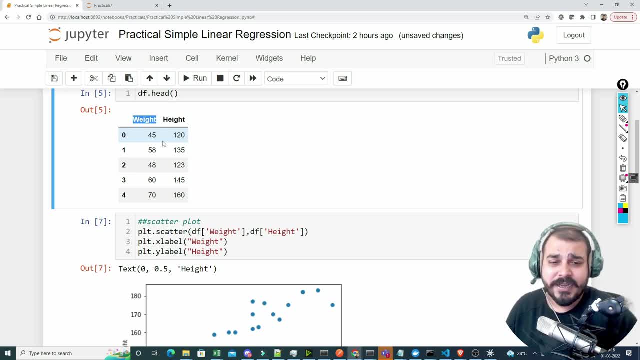 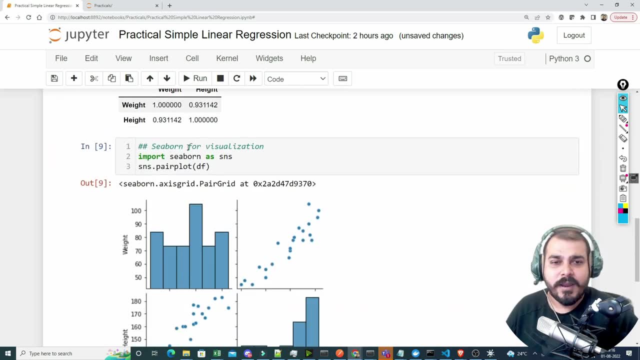 Those features which are highly correlated, either of the feature we can basically take. okay. So here let's go ahead with this one right now, because since in my independent feature I just have one, in the output feature I have one, so this is perfectly fine, and here you can see that. 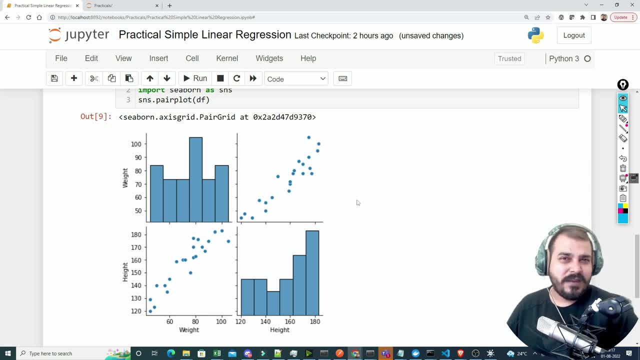 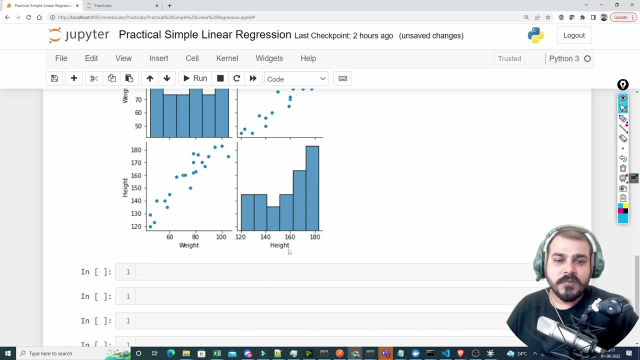 Okay, It is linearly correlated. So you get a good feeling that simple linear regression will work well, because at the end of the day I have to create a best fit line through it. Okay now The first step that we probably start in simple linear regression. here I am just going to divide my 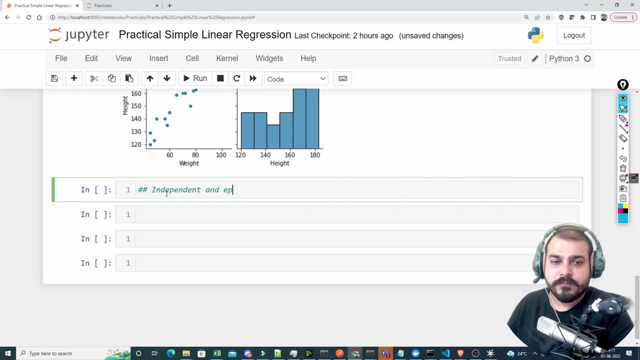 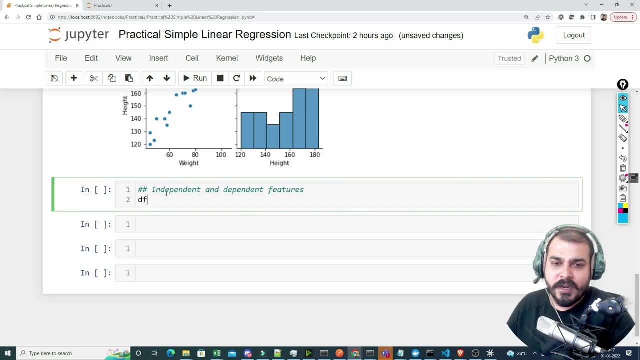 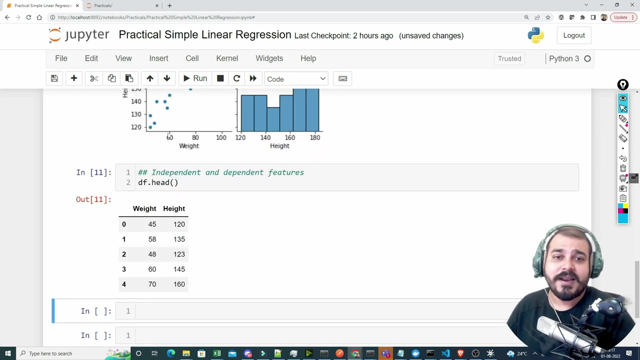 features into independent and dependent feature. super important Whenever we basically starts right Features. now, if I probably go and go ahead and display DF dot head here, you know that How many features I have now see. this error has come. so don't worry, because I know what is the error I made. 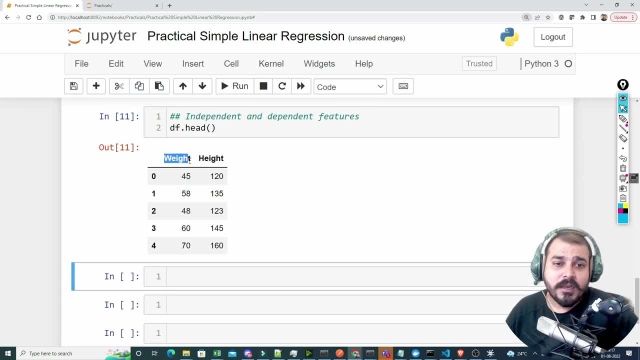 So here you have something like weight and height. Okay, now this weight is an independent feature and height is your dependent feature. So in order to create your independent feature, I will just name it as X. Just a naming convention. It is a good practice that we should use this kind of naming conventions. Okay, so X is equal to DF of. 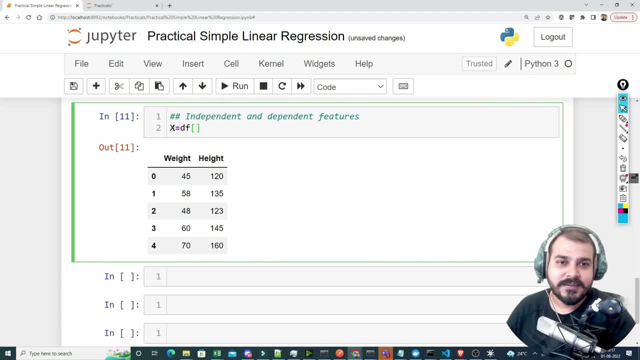 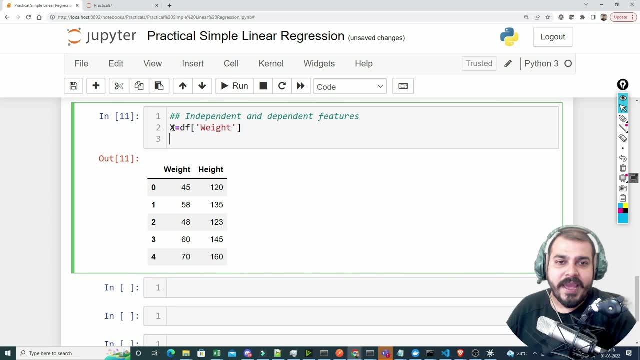 Now suppose if I want all my weight feature in the x-axis, So I can first of all write like this right? if I probably write like this right, Then the X that is basically getting created is a series right. So obviously I get my weight value over here, right? 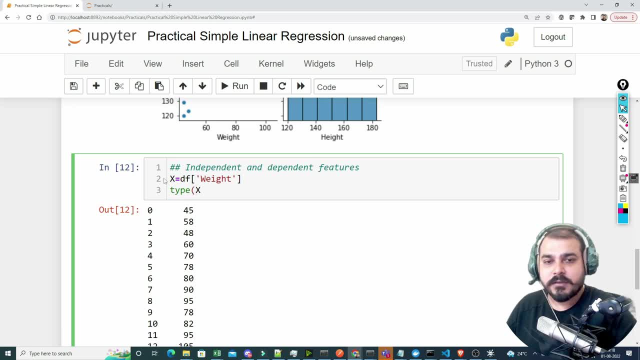 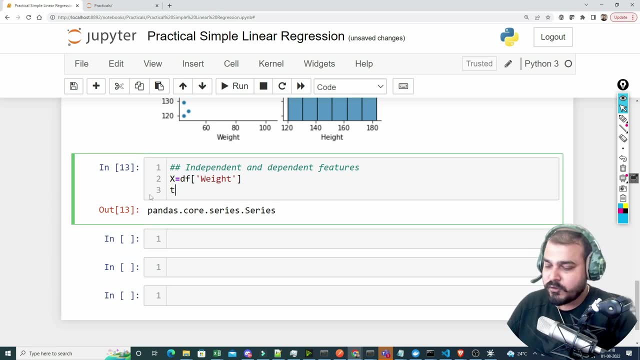 But understand, if I probably try to see the type of X here, You'll be able to see that it will be a series, not a data frames. right, data for a series now. But if I probably try to see type of DF, it basically shows me that it is data frame now. series basically means just a single. 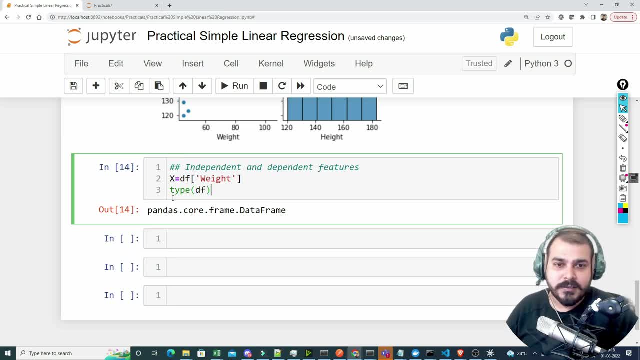 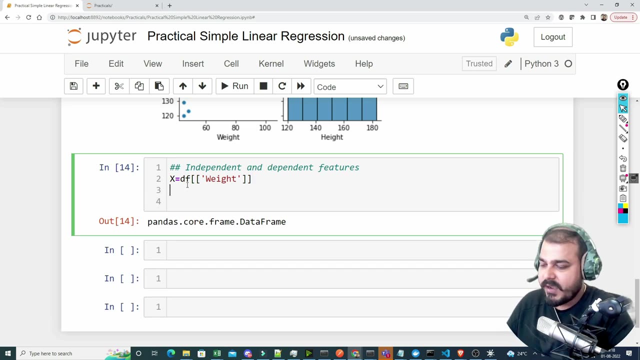 Record. you have to take care of one important thing, guys: whenever you probably try to Create independent feature, right, And if I use one additional bracket, then what will happen is that just see this: Okay, if I go and execute this like this and if I write type of X. 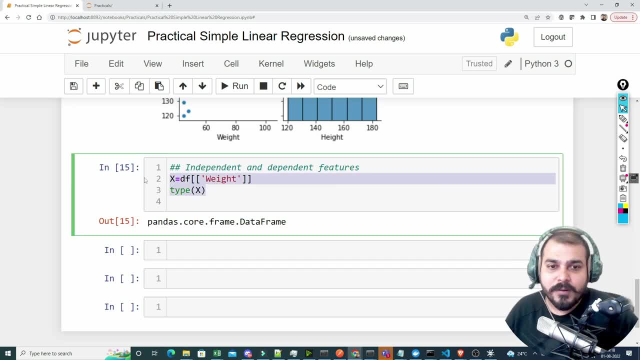 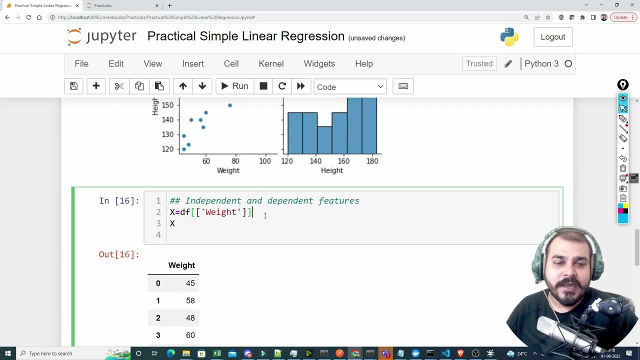 Now you know that we will try to get a data frame right and probably, if I try to Here, you'll be able to see that I'm getting a data frame with column name. always make sure That your independent feature right should be in the form of data frame or two dimensional array. Okay. 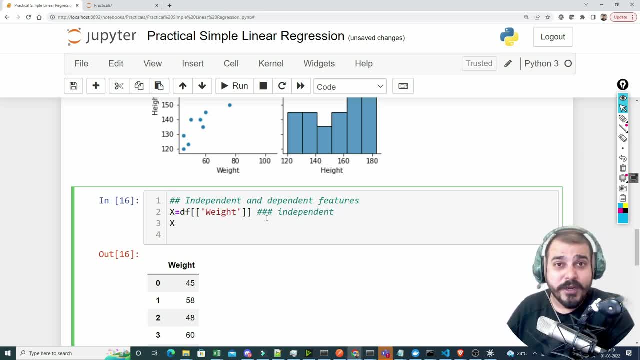 Independent. Yeah, I'm writing it over here because this will be super important when you're training your model. So your independent feature should be Data frame, or it can also be two dimensional array. when I say two dimensional array, What does this basically mean? this basically means I can have something like this see: 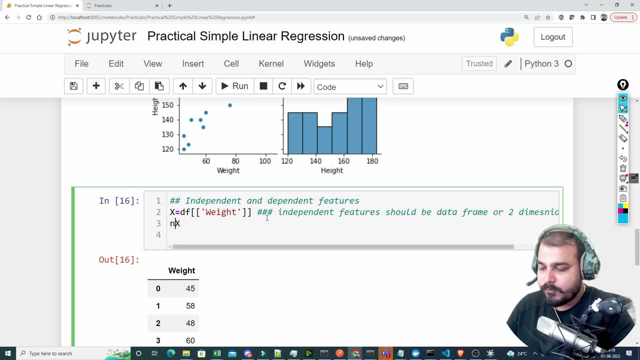 Suppose, if I write like this: okay, and now probably, let's say I'm going to write np dot array. Okay, and I'll probably write X: Okay. Now, if I write like this here, you can see that it is a two dimensional array. 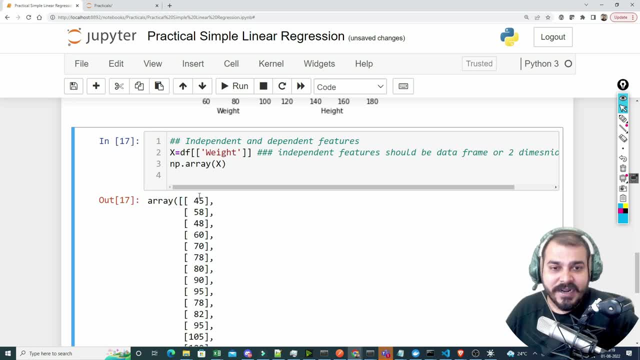 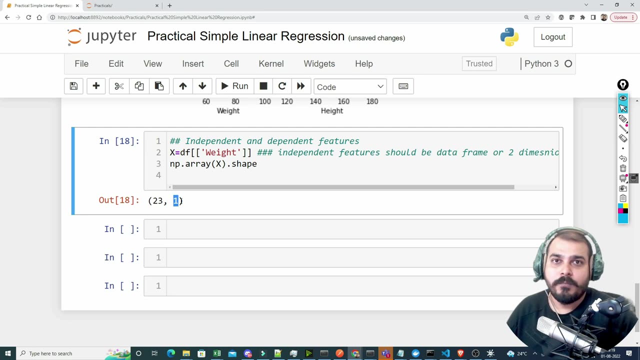 Okay, two dimensional array and this basically indicates that how many rows I have, I have one, two, three, Let's. let's just see how many rows I have for seeing how many rows I can basically go and execute shape. So if I write dot shape here, you can see that it basically has 23 rows and one column. 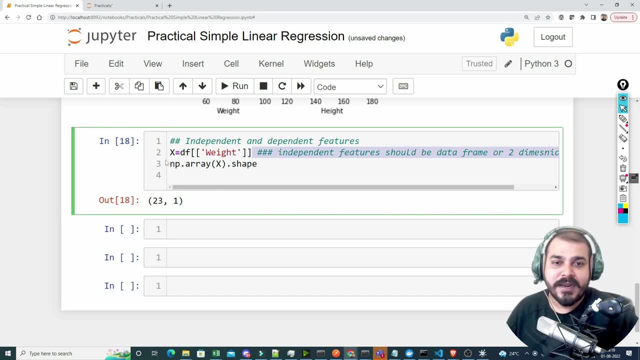 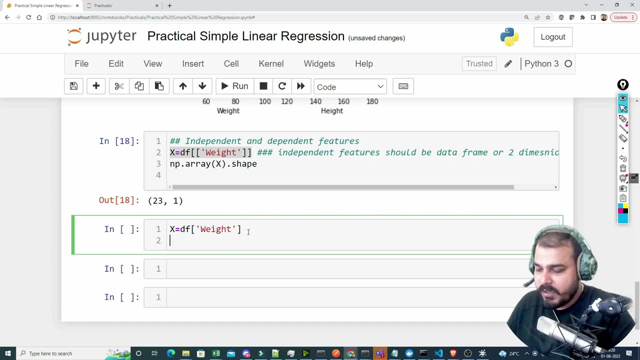 Okay, but in in data frame what was happening. Let's see in data frame What used to happen. suppose, if I go and execute like this and I remove this one bracket, Okay, and probably if I write NP dot array, right, I'm probably just go and see X and then write dot shape. 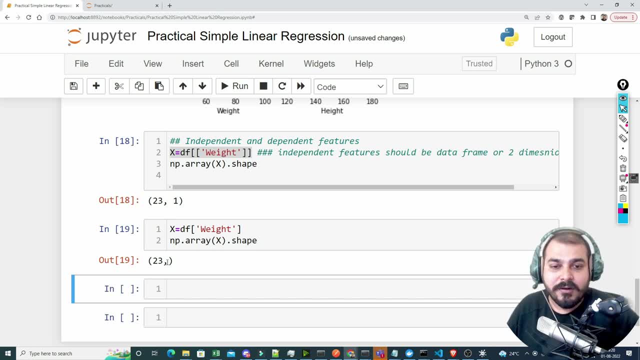 So here you will be, seeing that this will be a one-dimensional array. here No information regarding the column is given, but here importance should be given to the column right. So always make sure that at the end of the day, either it should be a data frame which has one column or it can. 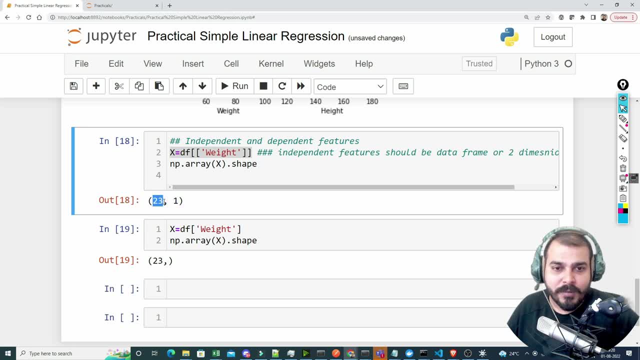 Be a two-dimensional array, also with with number of rows and some specific columns. right now, in multilinear regression, What will happen? this columns will increase. Okay, never keep in this particular format, because what will happen I'll tell you. Okay, let me just say that I am just writing this as X underscore series. 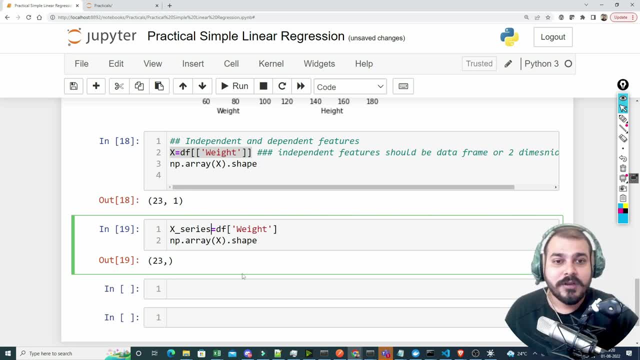 I will try to train with this and also, I will try to train with that also, and let's see where we'll get an error. Okay, So over here now. this is my X. Obviously, I've taken this as a two-dimensional Data frame which has one column. 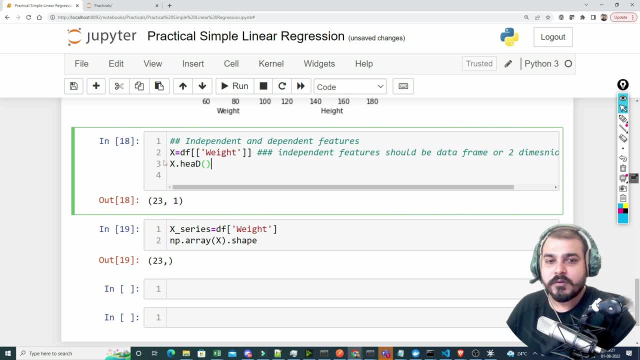 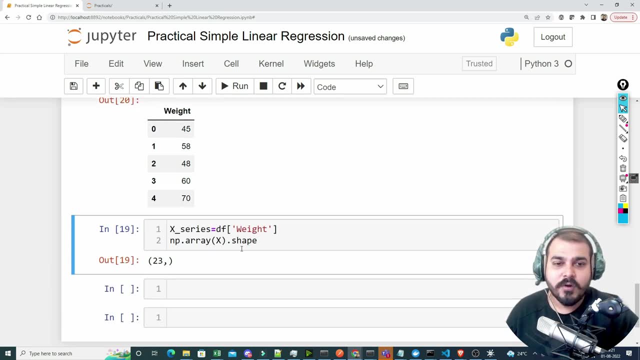 And then if I probably go and write X dot head, you will be able to see I will be getting this specific value. Okay, so this is my X. perfect. now, till here we have executed and let's go ahead and execute this also, And you know that probably if I also see the okay DF of weight. 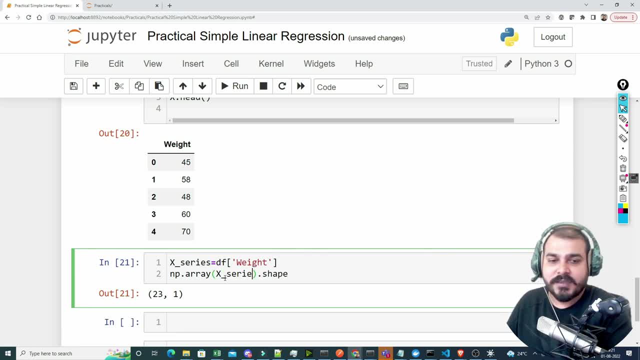 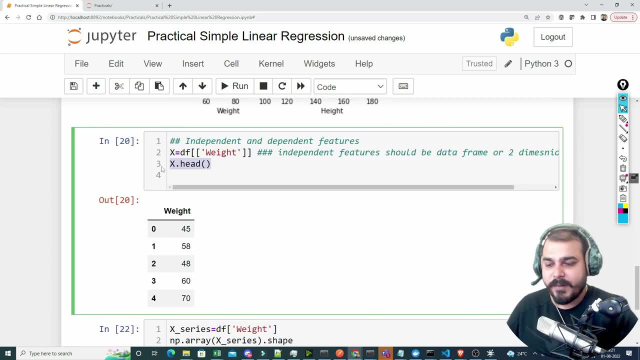 What happened? NP dot array- oh, I have to check it- and X underscore series. Okay, Now, here you can see. it is one dimension Perfect. This is done Now. the next thing is that, after creating an independent feature, I have to create dependent feature. now, in the case of dependent feature, 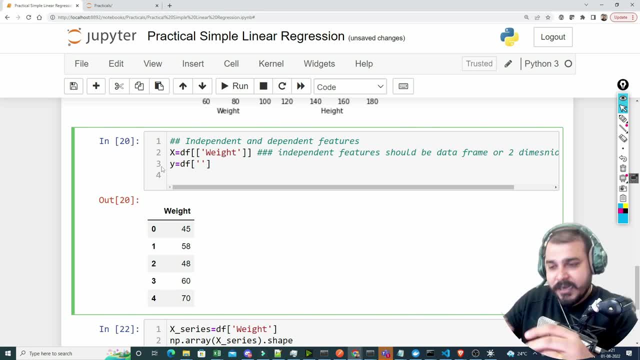 I can have it as a series: Okay, because dependent feature will only be one one column values, right, We don't have to worry much about that. But we do not have to make it two dimension. Okay, One dimension is properly fine in this, because we will have only one dependent feature in a specific problem statement. 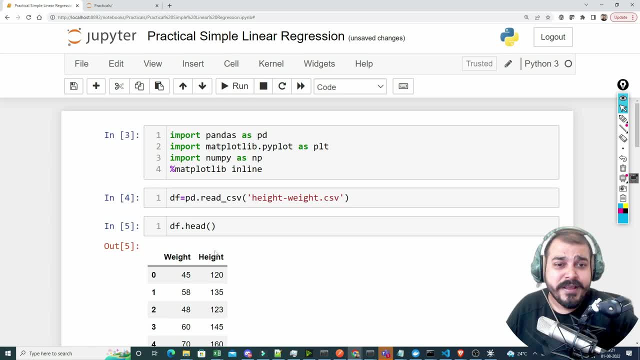 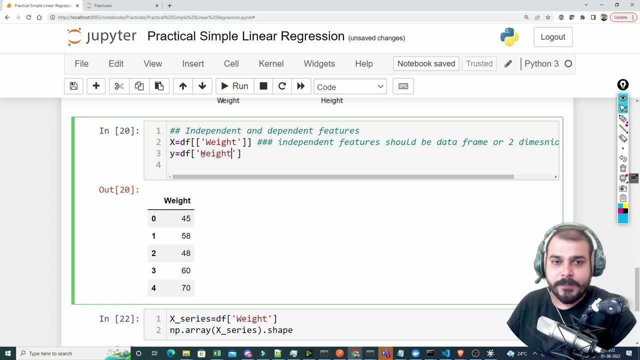 And this is a regression problem statement. Why do we say this has a regression problem statement? because here my output value is continuous. okay, super important point now. here i'm going to basically write df of height. now this is my y and this is my x. let's go and execute now. if you want to see your y, here is my. 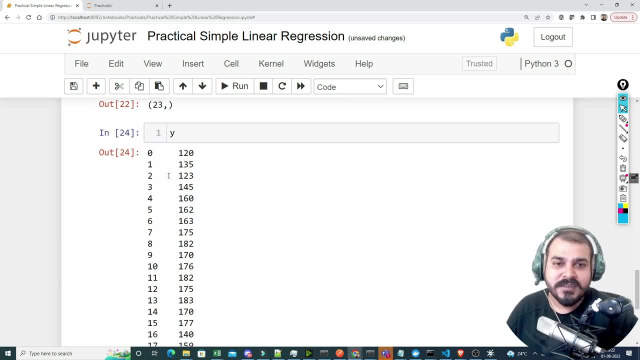 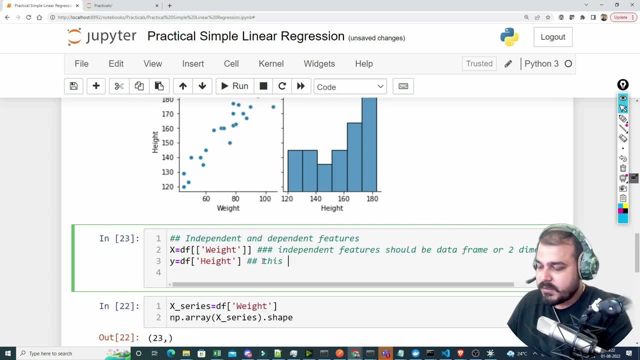 output feature. right with respect to this, and always remember this needs to be in series or it can be in one dimension. okay, so here i'm going to write it down over here: this variable can be in series form or 1d array. okay, 1d array basically means- if i probably write: 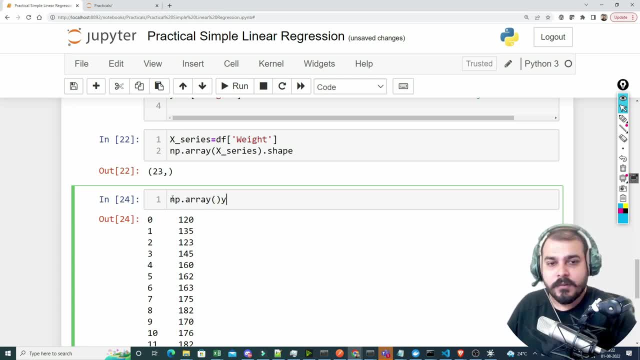 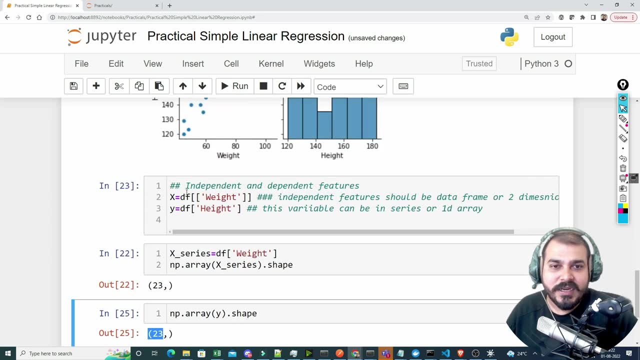 np dot array of y. okay, dot shape. here you'll be able to see only one array, so obviously 23. since you have 23 inputs, you have 23 outputs, right? so this is super important. so, and this is very much important, guys, otherwise at the last you'll face some issues, okay. 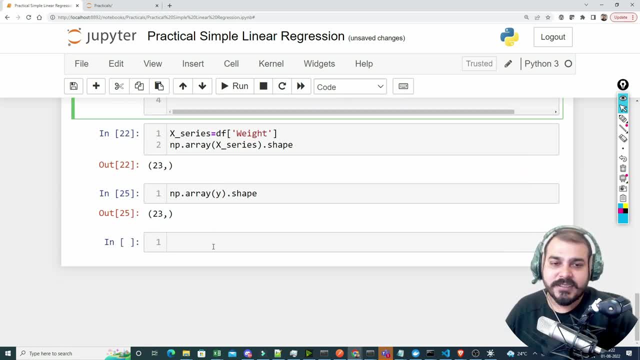 okay, So here I have actually done my independent and dependent feature. The next step: we specifically have to do something called as train test split, And I have already explained why you need to do train test split. This is for the overfitting- underfitting condition. 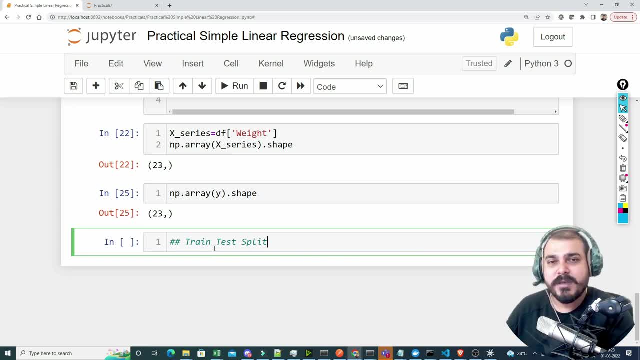 The train data only will be using for training purpose And the test data will just be used for checking how the model is predicting for the new data point. So for this we will be using a library from sklearntxt. So I'm going to import train test split. 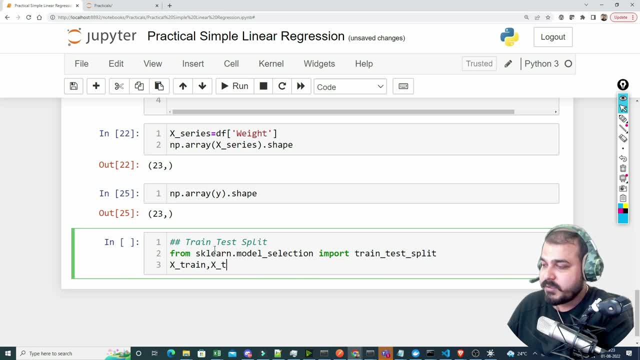 And here I'm going to use xtrain, xtest, ytrain, ytest. That basically means I'm creating a train data And with respect to that particular train data, see train and test. So training data will use the model for training that specific data. 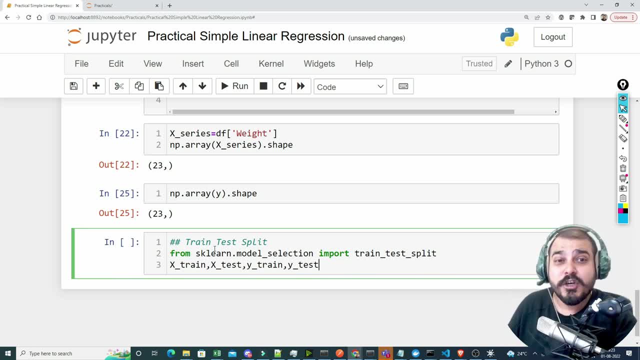 For testing that model or for seeing that how the model is performing. for the new data, we'll only use test data. So that is the reason we are creating these four components. Initially we just had two components. One is x and y. 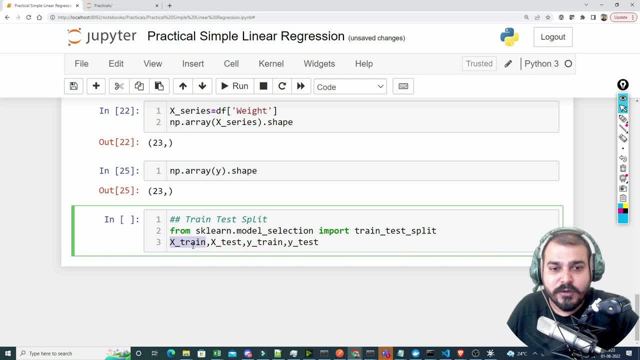 But obviously I need to create xtrain, xtest, ytrain, ytest. With respect to the output of xtrain, it will be present in ytrain. Okay, So these four parameters will get called when we use the train test split. 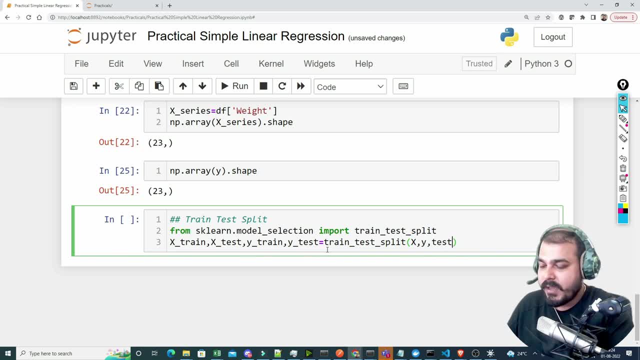 And internally we'll give x, y. Let's say, I'm giving my test size as 25%. Okay, So in order to give test size as 25%, I will write 0.25.. Now, how? How do you think I've got to know all these things? 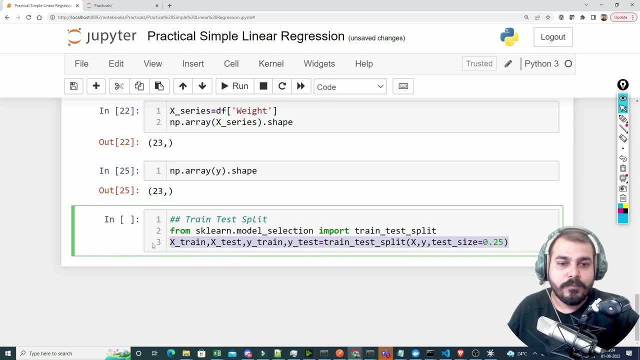 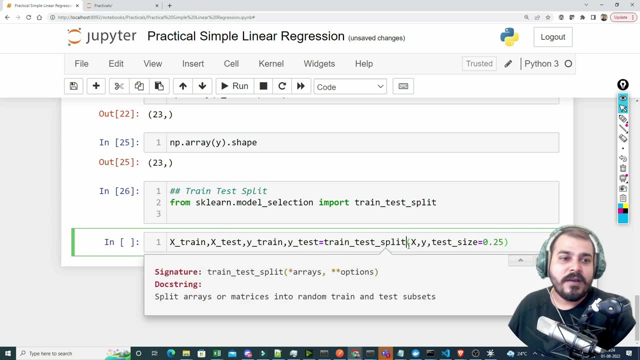 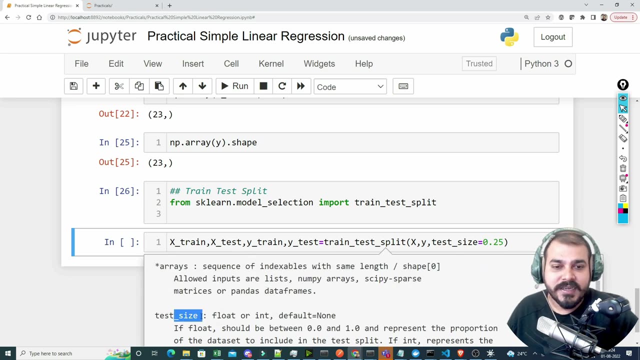 Just go and press shift tab. Okay, So, here this then only you'll be able to see it. Okay, So here you'll be able to see. I have just imported this And now, if I press shift tab, here you'll be able to see. or the arrays over here you can see test size I've given. 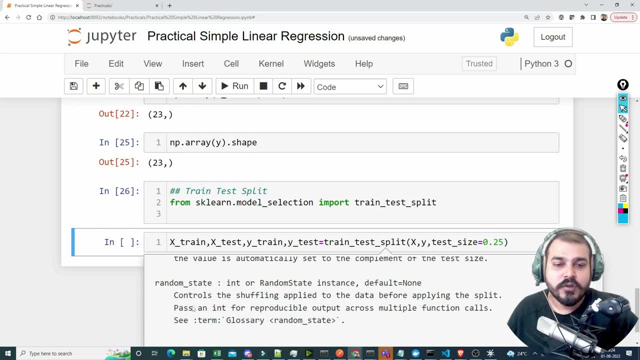 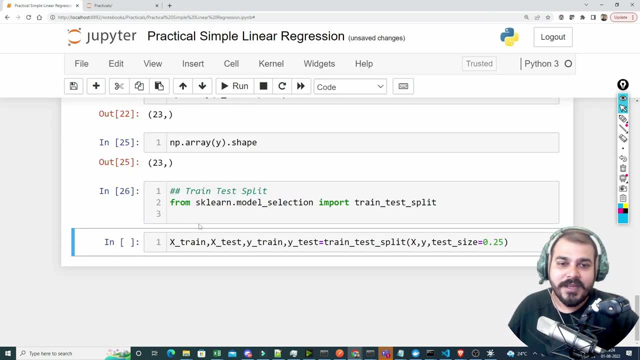 The arrays basically means x and y array, Train size also you can give, And there is also something called as random state. But before this let me make some cells. Just a second, I pressed F1.. That should not happen. Now let me just go and make more cells. 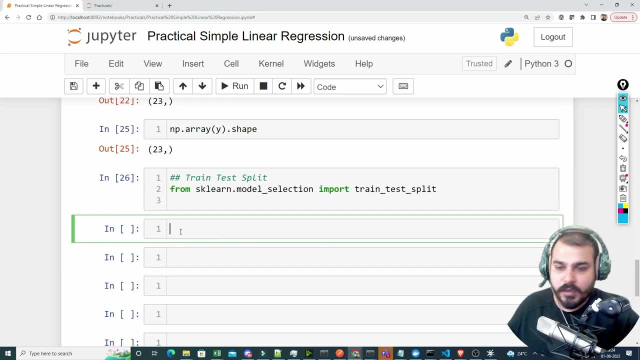 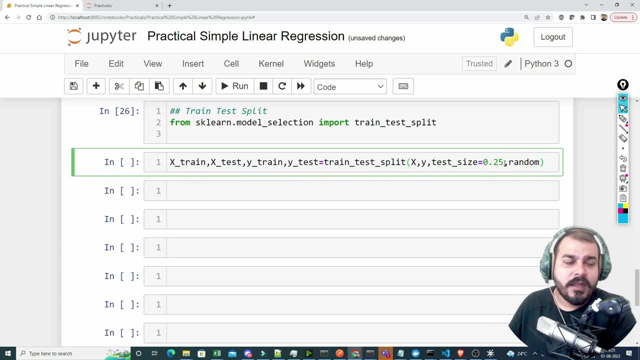 So I'll just copy this entire thing and I'll put it over here. Okay, Perfect. Now understand one thing over here, guys: There is something called as random state. Now see, usually when we basically take this random state- let's say I'm going to take 42.. 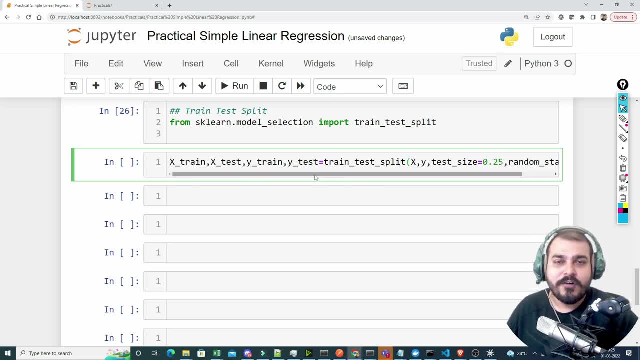 The type of train test split. if you don't put this random state right for everybody, it will be a different kind of train test. We can randomly pick up the record, 75% of the record, and put that in the training data set, and we can randomly pick up the 25% of the record and put in the test data set right. 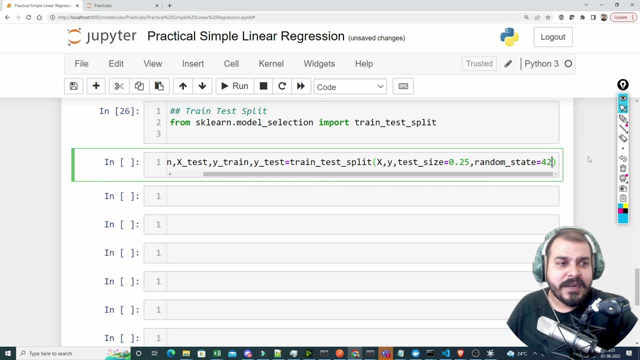 So that is what usually basically happens in this case. So if you write a random state as 42, so whatever way it is basically taking me, like taking my data and putting in the training data set, similarly for you also, that training data set will get selected. 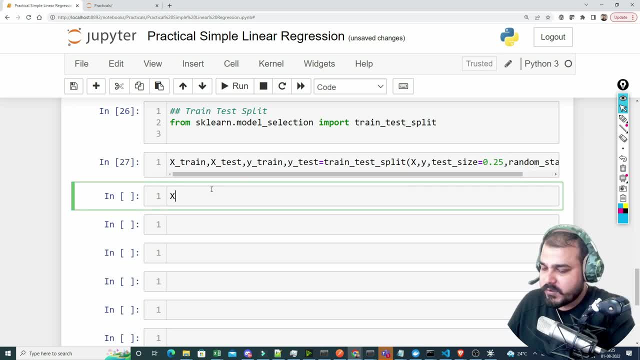 So once I execute it- so here you can see now- I will be able to see my x twin And I will just print the shape also And obviously, remember the shape should be two dimension Okay, Two dimension Okay. 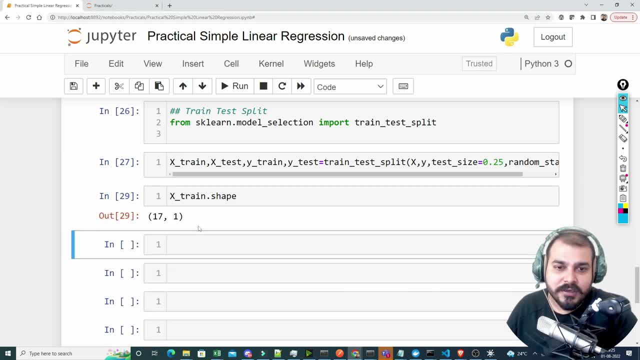 X twin dot shape. Sorry, I don't have to use this. And since here you can see, this is two dimension, right? That basically means this one is because of I have one feature and these are 17 rows, right? So 17 rows and one feature. 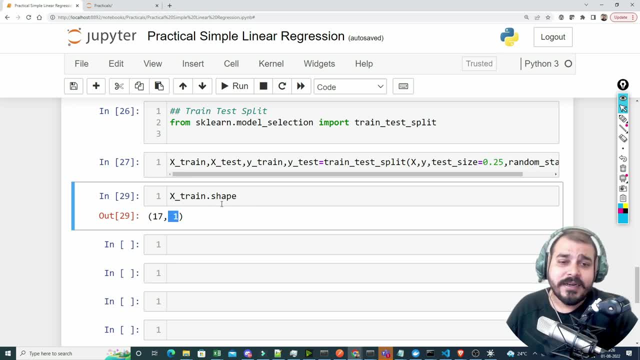 Similarly, if you have five features, then this will become five features. Okay, Like that it will happen. Okay, But at the end of the day, you will be getting Two dimension. Perfect. Now let's go ahead and let's discuss what we have to do after this. 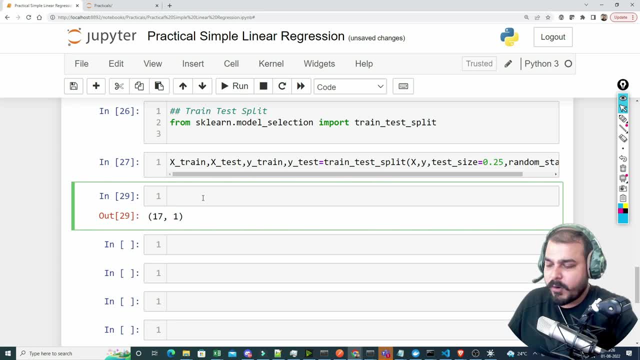 Okay, Now we have to perform a very important step, which is called a standardization- Standardization Why it is basically required. Now, just understand that I'm also going to write in front of you. Let's say I have two features: X and Y. 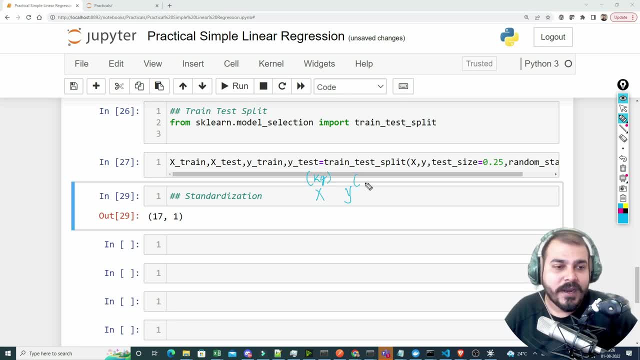 Let's say X is calculated based on kg units, Y is calculated based on some other units. Let's say over here. in this particular case, since this is height, I'm going to use centimeter. Okay, Now understand one thing: whatever values you get over here, right. 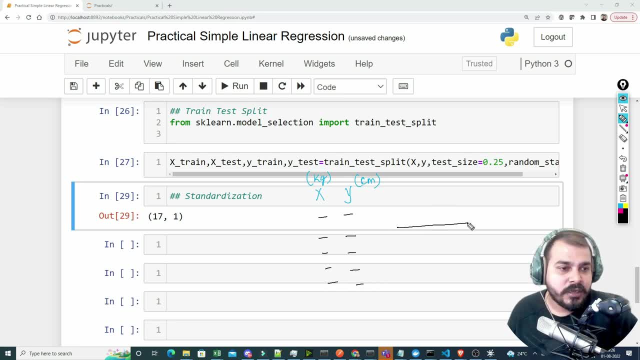 These are of different units And you know that in linear regression when we use a scalar we use something called as gradient descent. So obviously based on this unit, if this value is higher, to come to the global minima right. 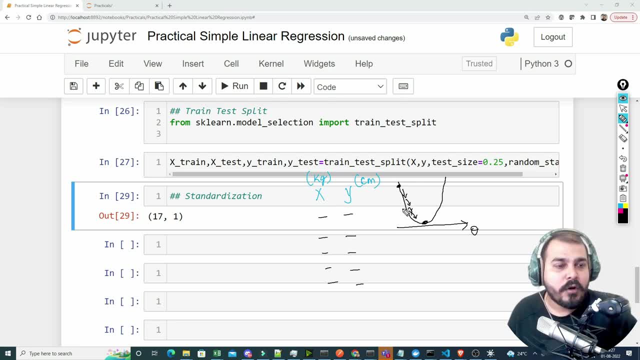 It is going to take time, right, Because I have a bigger value and all the maths equation that is getting applied. It will get applied to a big value Right, Which is again not a suitable solution. Okay, And obviously the optimization problem will take long time to reach the global minimum. 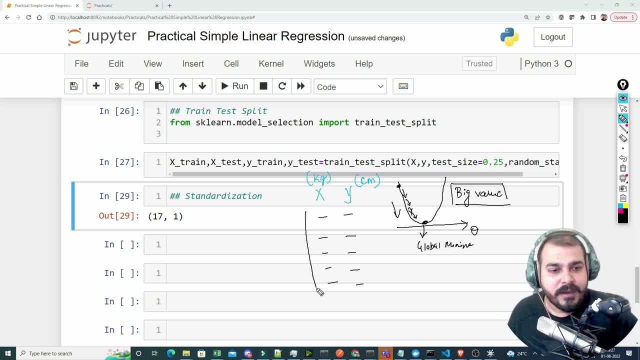 Okay, So what we do is that a very good approach is that we take up each feature, not the output feature. we take up each independent feature and we apply a simple formula which is called a Z-score, And this formula will basically be converting all your values. 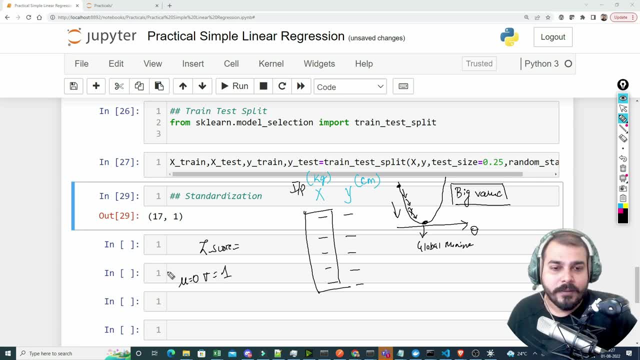 with mean is equal to zero And standard deviation equal to one. Okay, That basically means, if I take up all these data points, I will write X of I minus mu, divided by standard deviation Only. this formula gets applied to all data points. 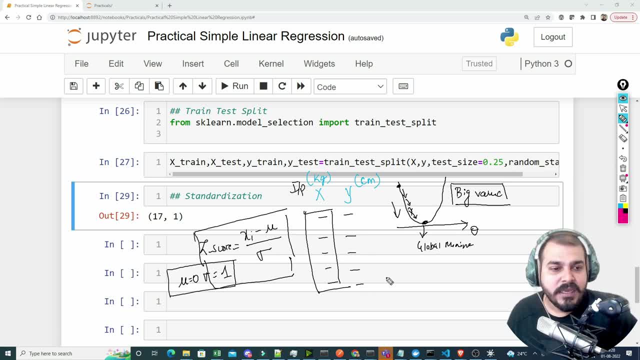 At the end of the day, what will happen is that my mean- all these data points will get converted with- mean is equal to zero and standard deviation equal to one. Super, super important, Okay, So please make sure that you remember this. 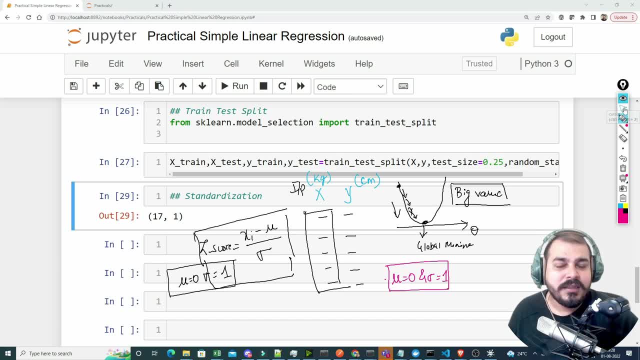 And this is a very good step. With respect to standardization, in the upcoming future, I will also talk about which all algorithm you not apply feature, You need not apply standardization. Okay, That part also I will try to discuss. Okay, Now, what I'm actually going to do and rub this and let's apply standardization. 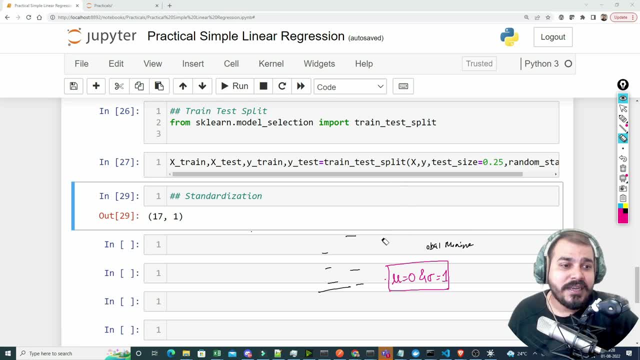 Now for standardization. again, we will be using an sklearn library. See, guys, every library that we are going to use, you will be able to get it in sklearn. Okay, So if I probably show you one case right, Let's say I have 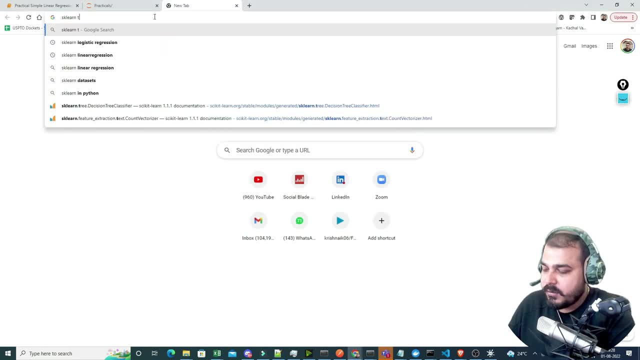 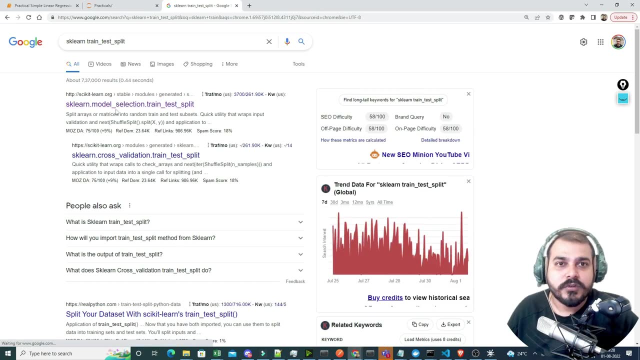 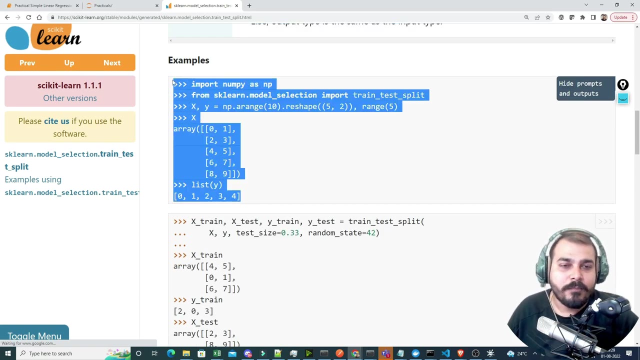 used train test split. So if you go and probably search for sklearn train test split here, you will be able to see that this is the algorithm that is specifically used. So here you can see all the parameters, what parameter, what it returns, and you can also see some of the examples. 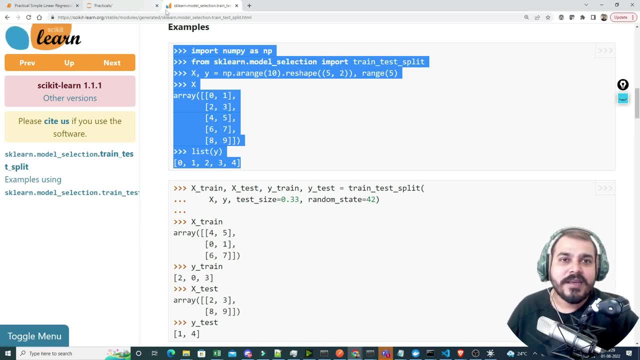 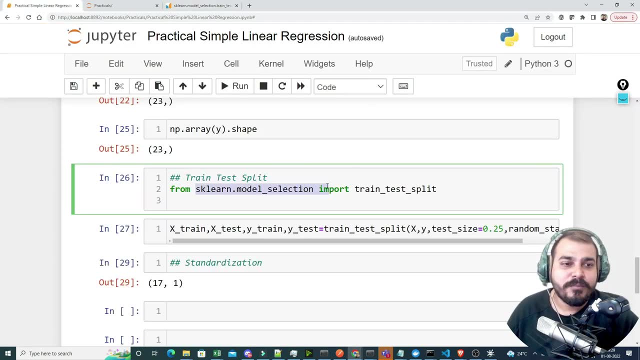 Right. So all the time, suppose, if you don't understand where this library exists, all you can do is that search the Google for that specific library. So that is the reason I'm able to write from sklearnmodel selection: import train test split. 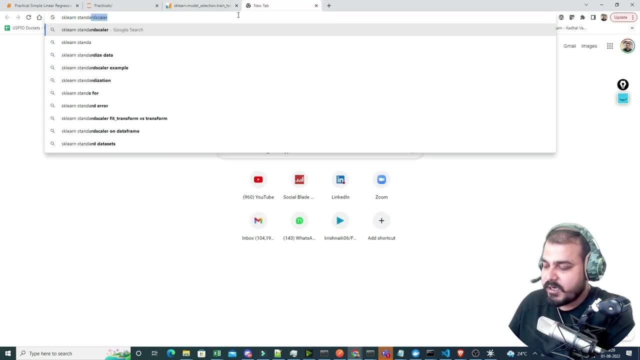 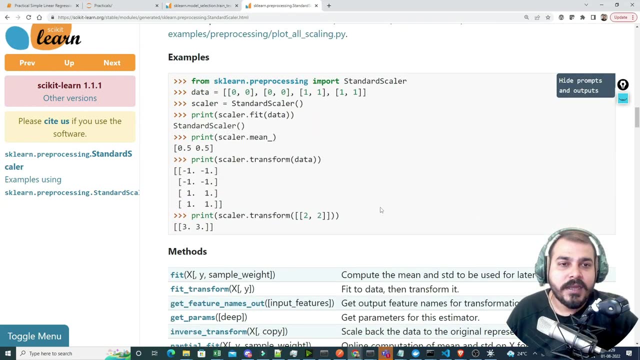 Similarly, here you will be able to see: sklearn standardization is there, which we call it as standard scalar. Okay, Now, if I probably search this and if I probably see this here, you'll be able to see that you are getting all the values over here. 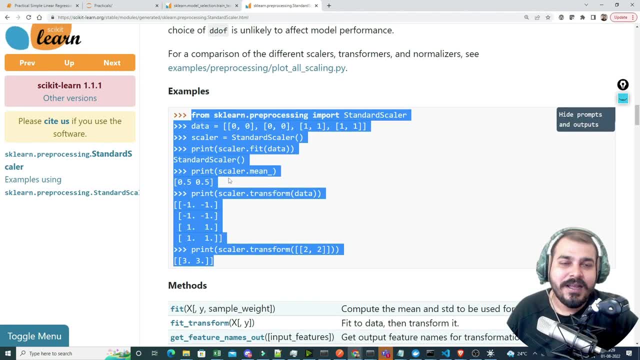 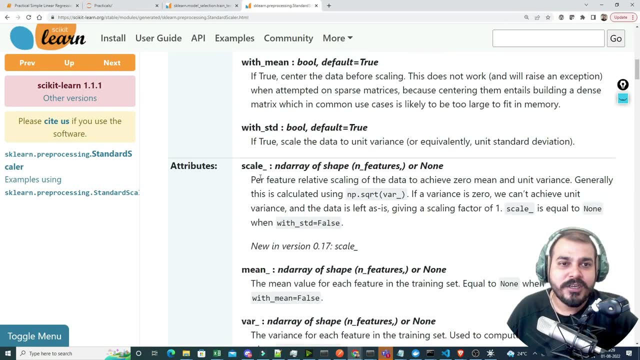 Right, So perfect. We are very much in sync and we are able to understand. Okay, Now the next thing that we are going to do over here is perform standardization. So, from standardization, what is the library from sklearnpreprocessing? 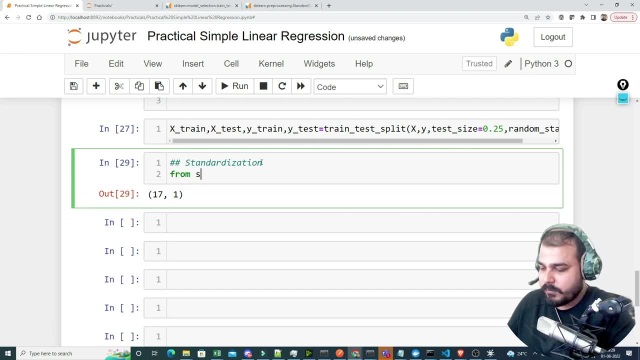 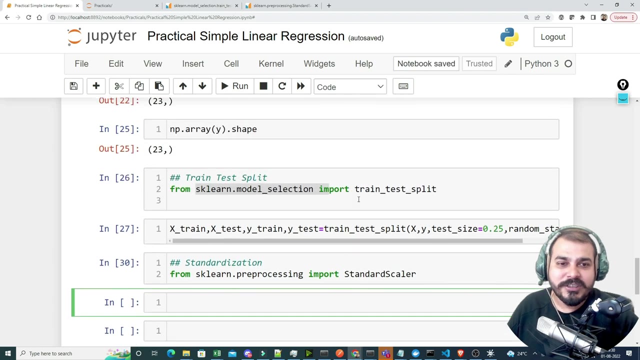 Okay. So here I'm basically going to write from sklearnpreprocessing: Okay, Import standard scalar. Okay. So once we do this, let me just execute it. And here now we are going to standardize my input feature, not the output feature. 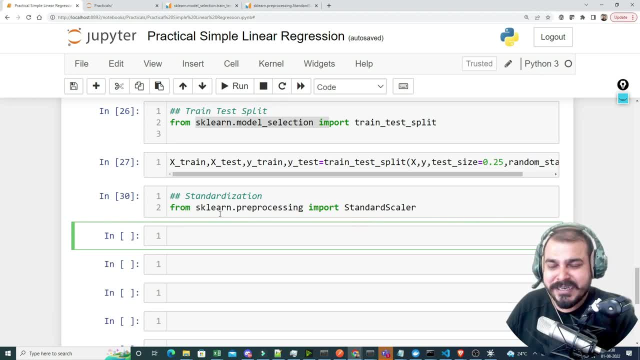 We do not have to standardize the output feature, because our gradient descent gets applied into the independent features, Right? So what I'm going to do over here is that I'll just say I'll initialize, Standardize. So let's say I'm using standard scalar. 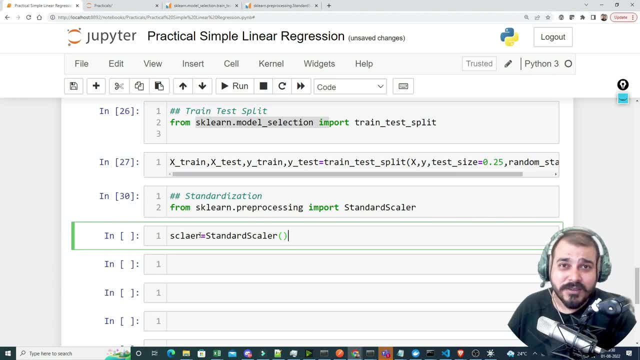 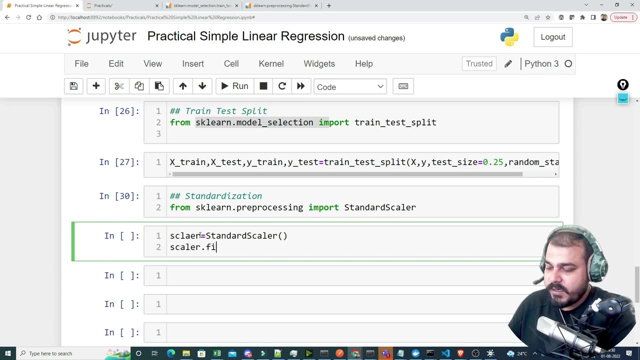 So this will initialize with that formula that I've written: Z is equal to X of I minus mu divided by standard deviation. Okay, Then after this it is just going to write: scalar dot fit underscore transform. So let me give this formula again: scalar dot fit underscore transform. 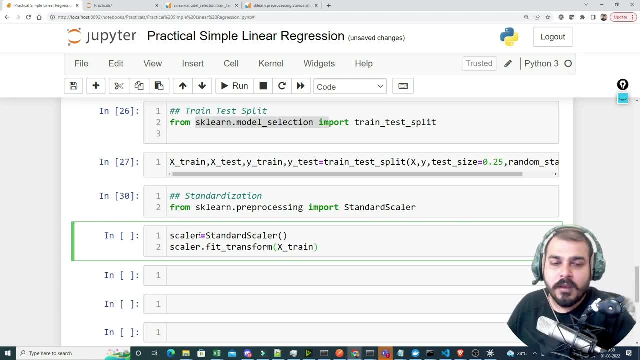 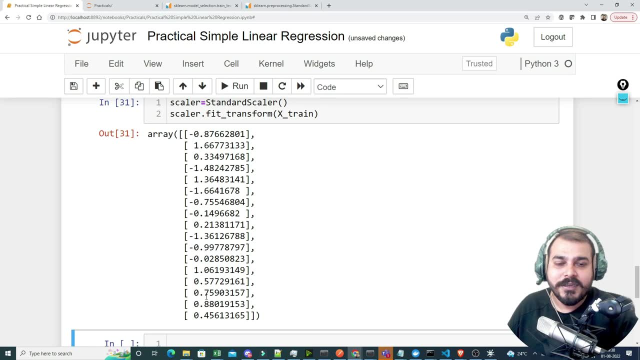 And here I'm just going to give my x-train. Okay, What will happen for all my x-train data? this transformation will get applied Now. here you can see all the data points over here. Mean will be zero and standard deviation will equal to one. 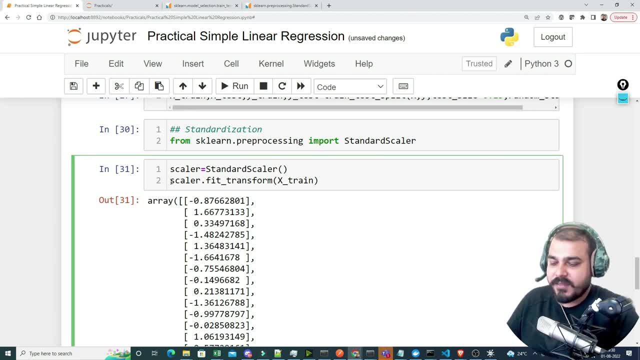 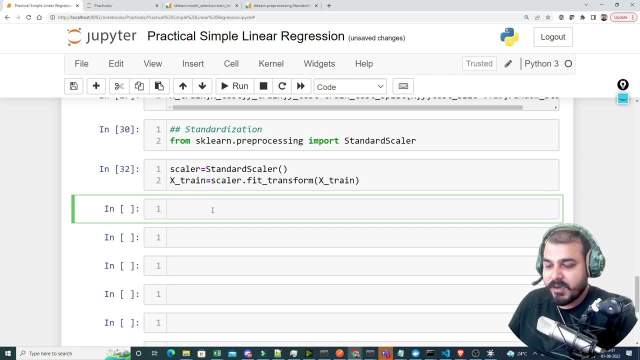 Then that basically means all your data points will be transformed in this scale And this I will assign it to x-train. Now, the same thing I need to do for test data also. Right, But always remember, in test data we do not apply fit underscore transform. 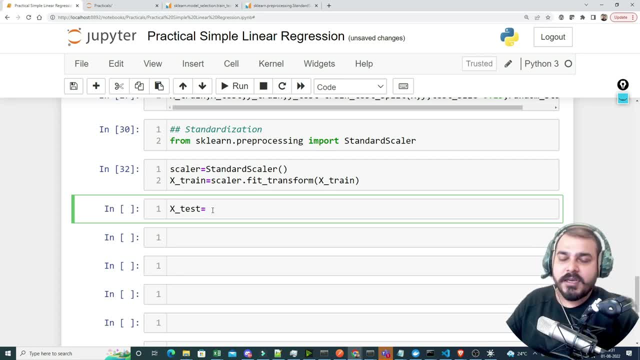 See the difference between fit, underscore, transform and transform is that initially, whatever data that I have, let's say whatever data I have in train, I'm going to use the same mean. Let's say the formula is like this: X of I minus mu divided by standard deviation. 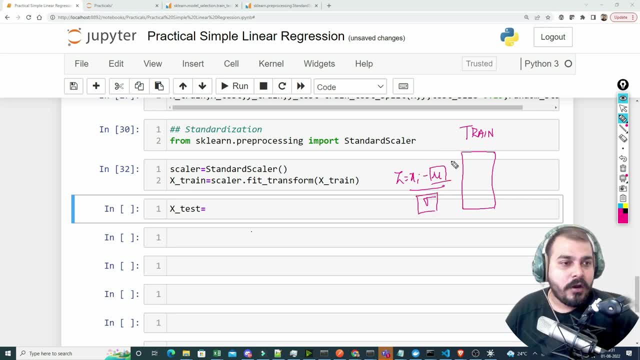 I'm going to use this mean and standard deviation only of this training data set And I'll apply the same formula in the test data set, Right In the test data set. So for this particular case, what I do in training, I say fit underscore transform. 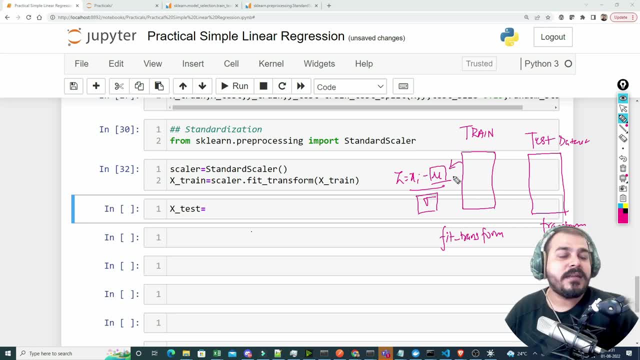 And in the test I just say transform. When I say transform, that basically means I'm going to use the training data set mean and standard deviation and use it over here, OK, And apply the same formula like X of I minus mu divided by standard deviation. 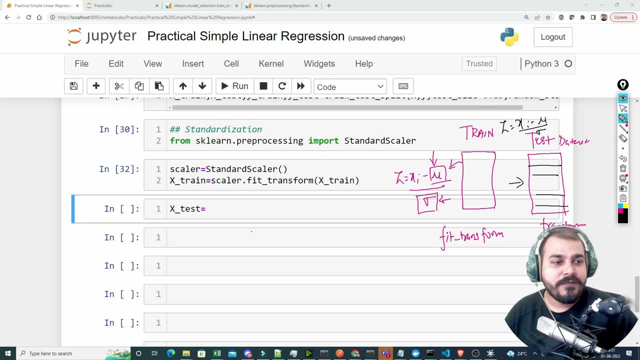 For all these data points. I'll be using this mean and standard deviation only if I use transform. If I use fit transform, then again mean or standard deviation will get calculated for this data. I don't want that, And why do we do this? 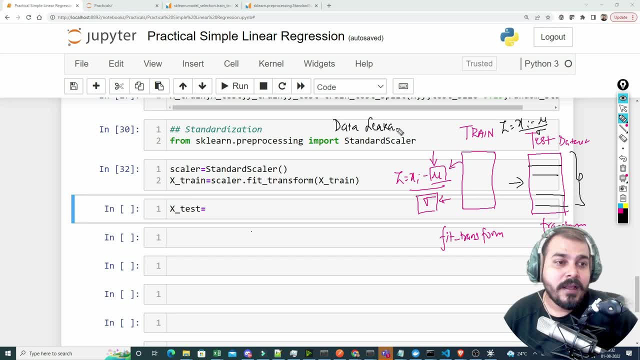 Because there is an important concept which is called as data leakage. I don't want my training data to know any info about test data. OK, I don't want that thing to happen. You know my, my model that is created. this should be the truth value. 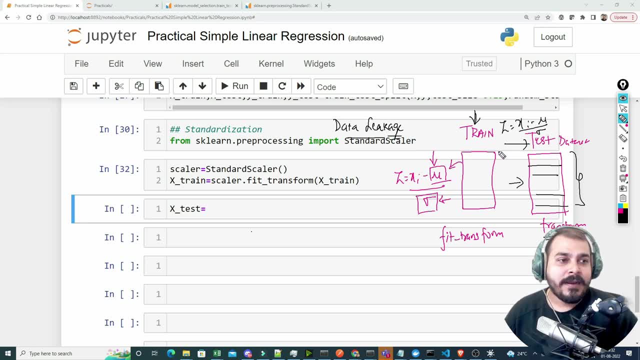 OK, This should be the information that should only be known Right, And when my model sees this, it should always see this as a new data, So that then only we'll be able to understand whether our model is performing well or not. 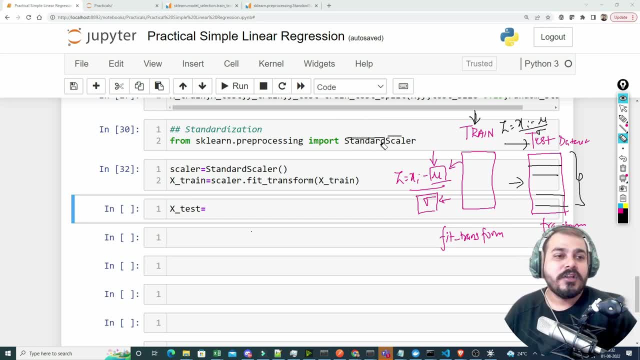 OK, Super important data leakage: fit underscore transform and transform. So this is a very important interview question. OK, Why do we use fit underscore transform? And this we will also be doing in PCA. that is principal component analysis. OK, Now let's go ahead and let's continue. 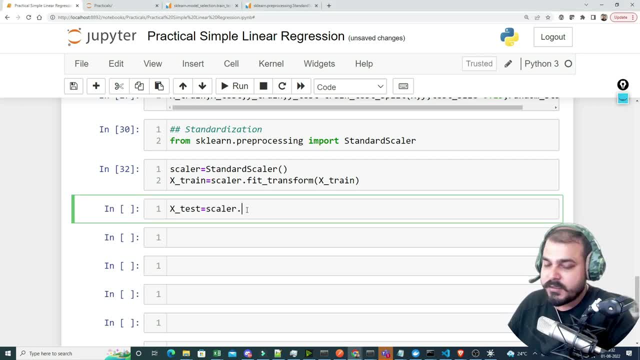 So here what I'm actually going to do here for the test data and writing: scalar dot transform- OK. Scalar dot transform- OK. And then I will basically write this on my X test data. Let's see whether we'll get any error. 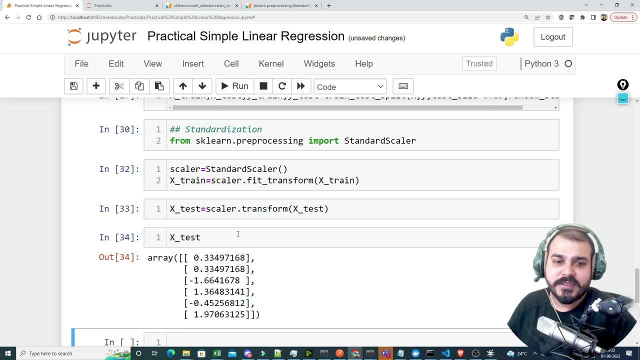 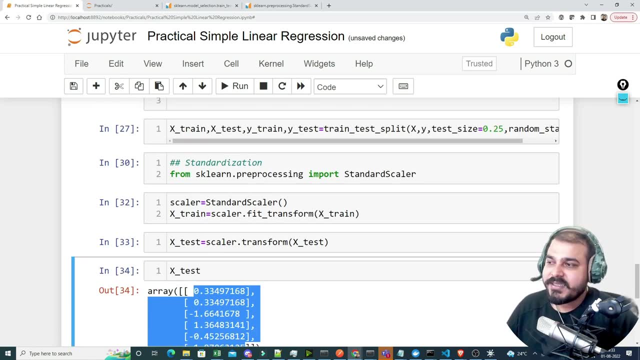 So, here again, this is perfectly done. Now, if you probably go and see your X test, you are going to get this. So this is my test data and this is how it has got transformed. This is perfect till here Now. the next step that we are probably going to do is that apply machine learning algorithm, that is, linear regression. 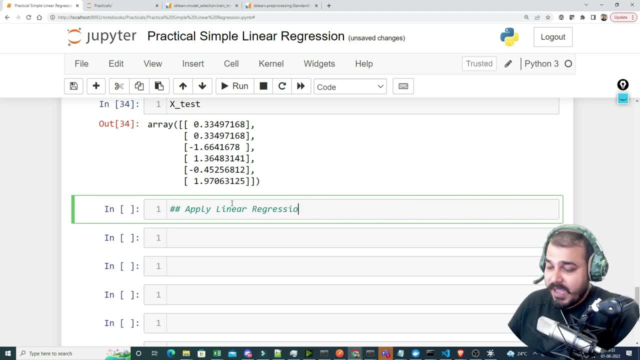 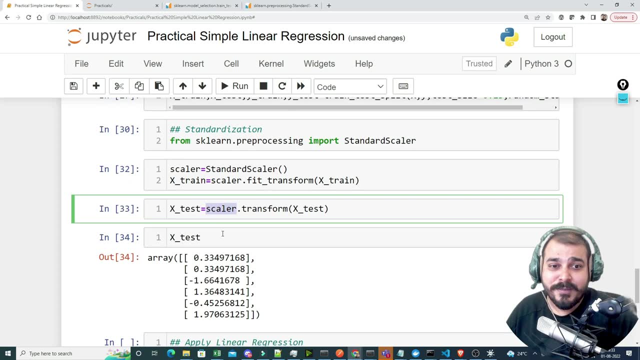 Apply linear regression. OK, And this is super important, I will again be using this, this particular scalar value. OK, This will be again used for the new data also. Any specific new data that has come will again transform them. OK. 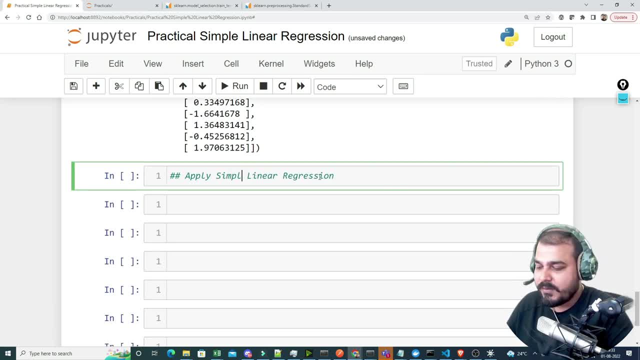 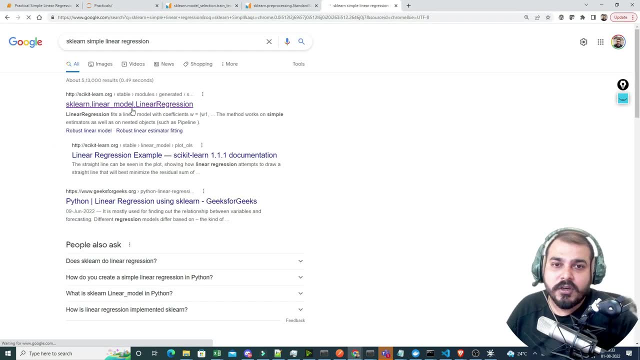 Now I will apply simple linear regression. Now, in order to apply, we'll again use scalar, And in this scalar I will search for simple linear regression. So here you'll be able to see something called as linear regression. So this is the model that we are going to apply. 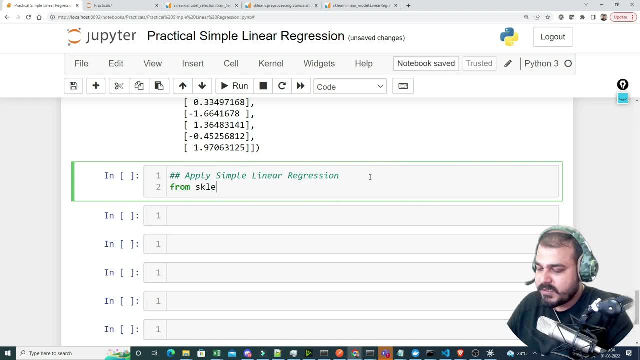 So let's go ahead and let's write form: scalar dot, linear model, import, linear regression. OK, Now, here you'll be able to see the first thing that I will do again. So I will initialize the object whenever we are using any any libraries for my scalar. 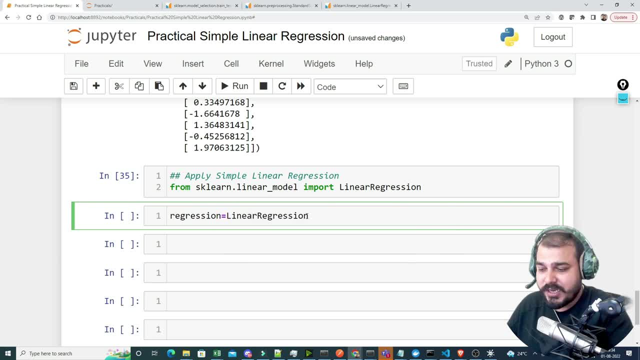 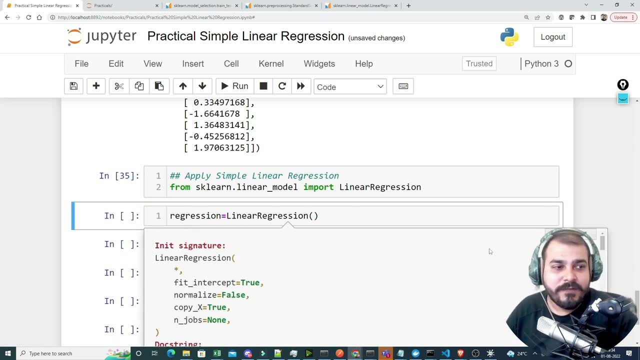 First of all, we need to initialize that object. OK, So here I'm going to initialize linear regression By default. the parameters, what all things are there? So there is a first parameter which is called as fit underscore intercept. Now, this fit underscore intercept is nothing, but it will say that, whether 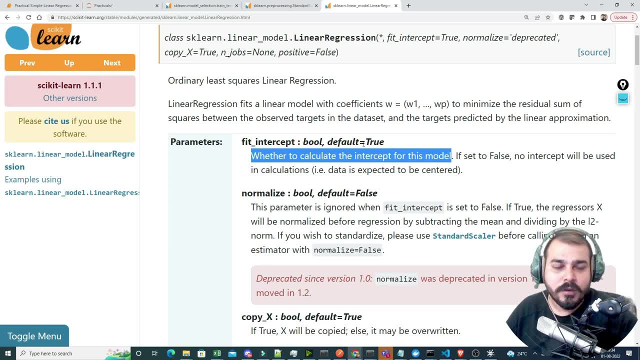 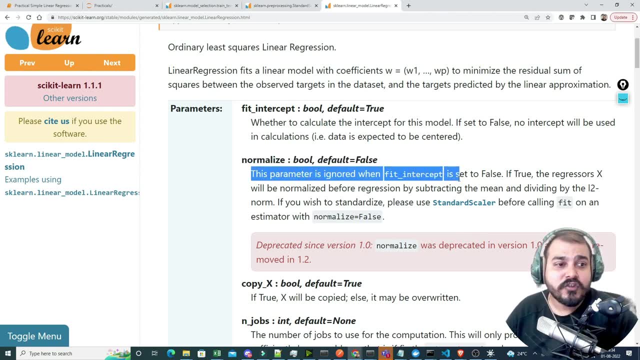 to calculate the intercept for this model or not. Obviously, I want to calculate this, So by default, whatever true it is, I'm going to keep it as true. Now, this normalized function is there. This parameter is ignored when fit underscore intercept is set to false. 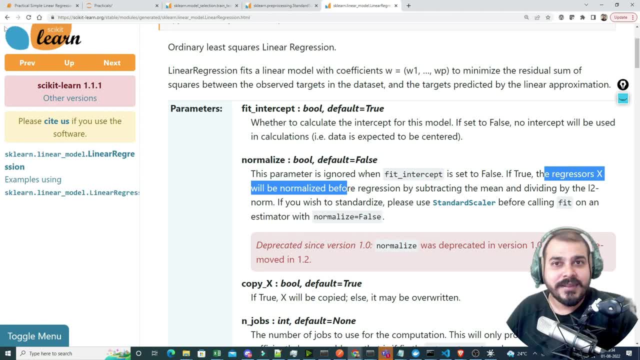 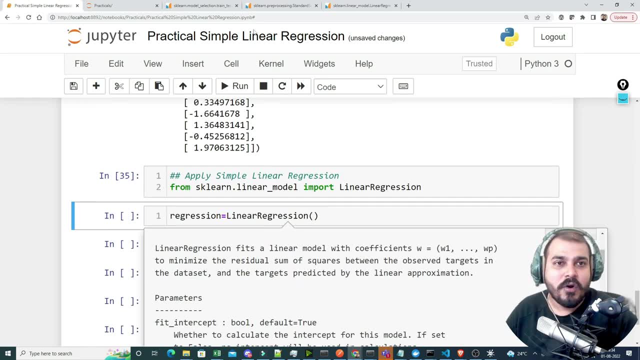 If true, the regressor S will be normalized. And this process- we have already done this Right. We have normalized here. We have standardized this by using standard scalar. We have already done that. So whatever will be the default value will keep. 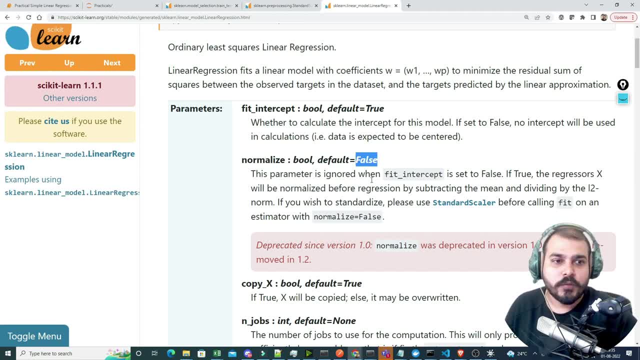 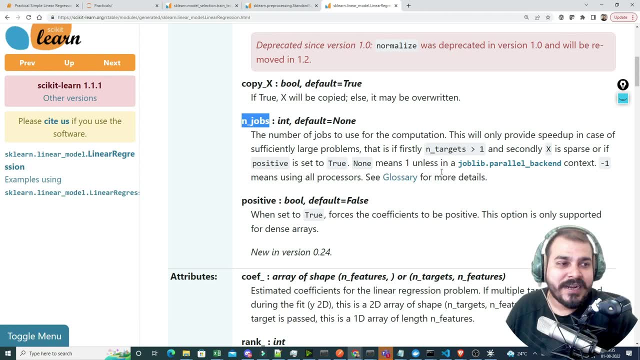 If you are not done that step, normally you could have kept this as true. OK, Then you have N underscore jobs. This N underscore jobs is a very important parameter, because if you set this as minus one, it is going to use all the processors that are there in your system with that. 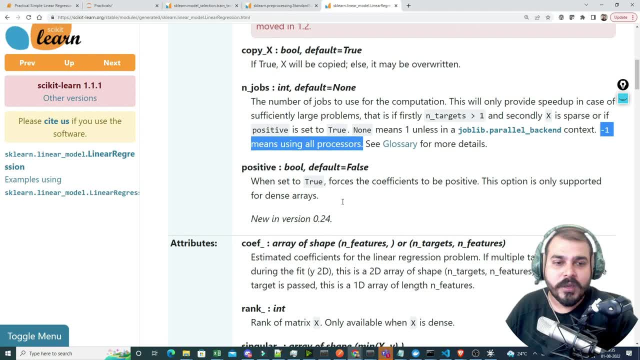 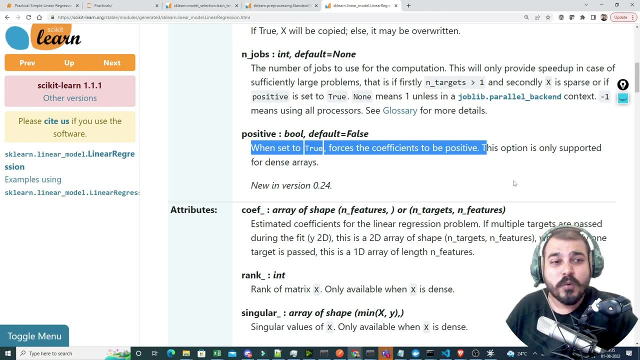 With the help of them it will try to converge and it will try to do the training OK And positive basically says that when set to true forces the coefficient to be positive. So I don't want this specific thing to happen because some of my coefficients can be negative. 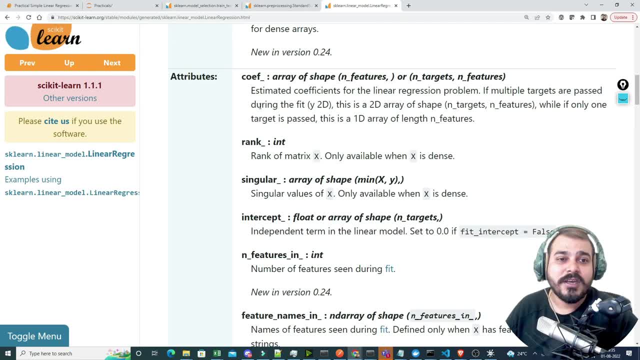 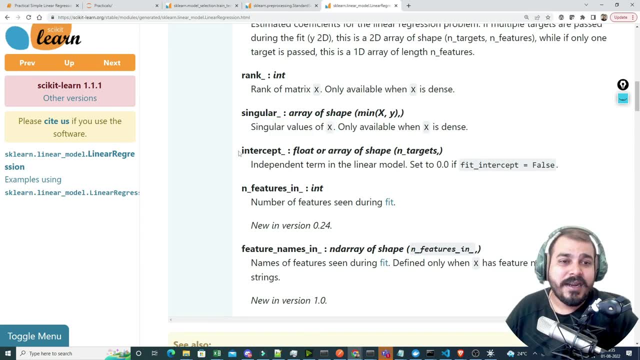 Then in return, what all things you'll be getting if you apply this algorithm Here. you'll be getting coefficients, rank, rank of matrix, singular, singular value of X, intercept. But out of all these things, right, the most important thing is coefficient and intercept. 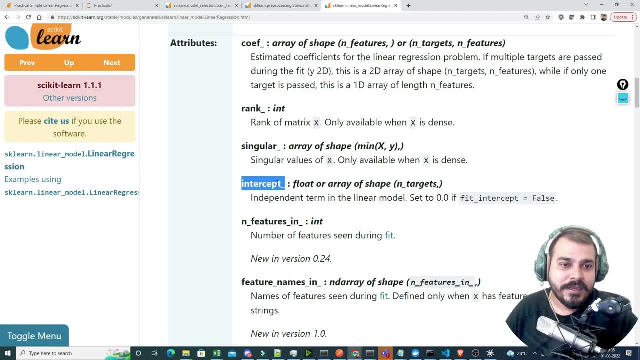 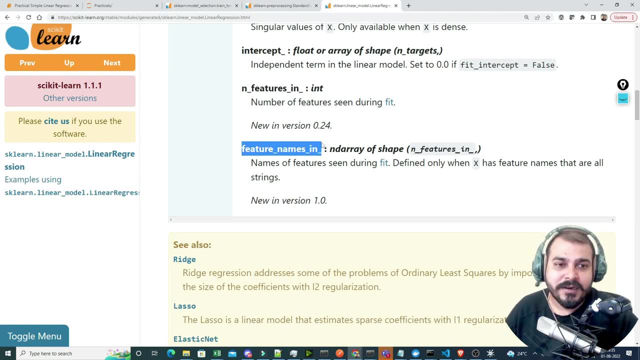 And we'll try to see that. how many, how many, what is the coefficient intercept and what is the relationship with respect to the final output. We'll see that there is also a feature that will get returned. That is called a feature. underscore names. underscore in name of feature seen during fit. that also it will show. 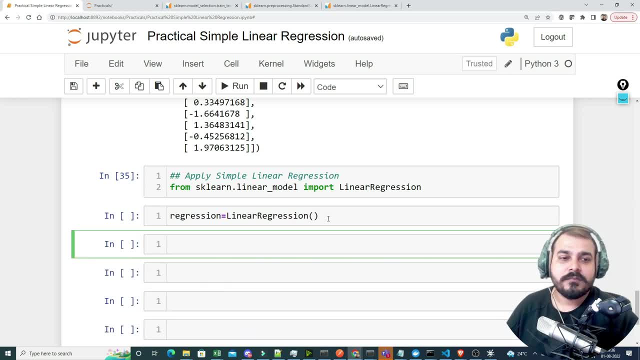 We'll try to see this, OK. So here I have applied linear regression. Let me just go and execute with all the default parameters And I'll say: regression dot fit. Now I want to fit this regression model to our training data, Right? So all we will do is that we will go ahead. 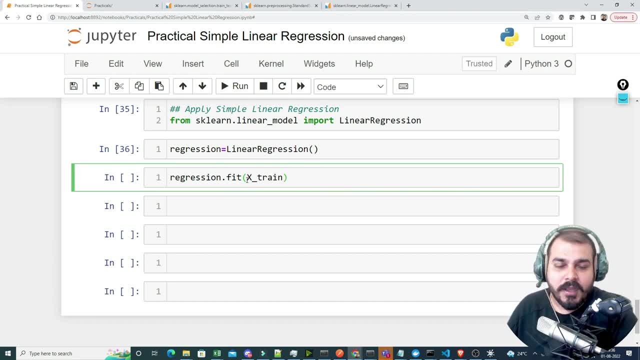 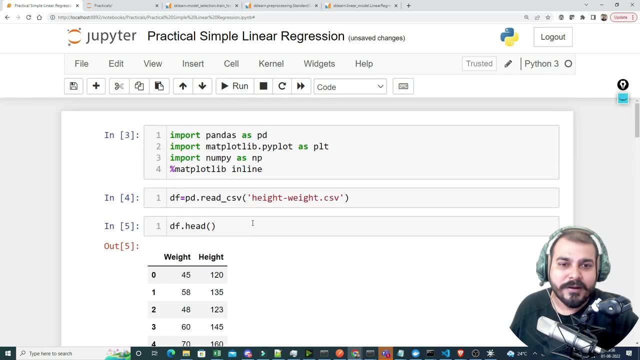 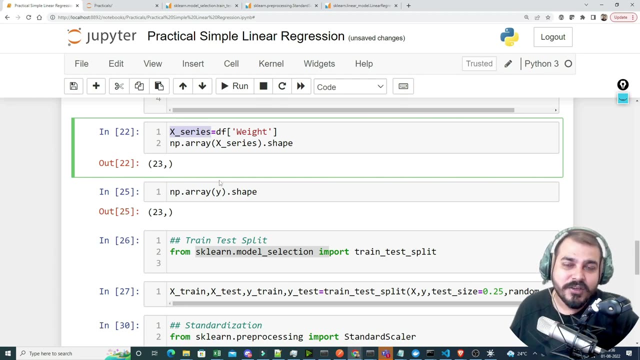 and assign this, and we'll assign it to X underscore train. Now, understand this. Let's say, before giving this X underscore train, let's say I created one more variable, right, and that specific variable was called as X underscore series, Right, And you know that this is one dimension. 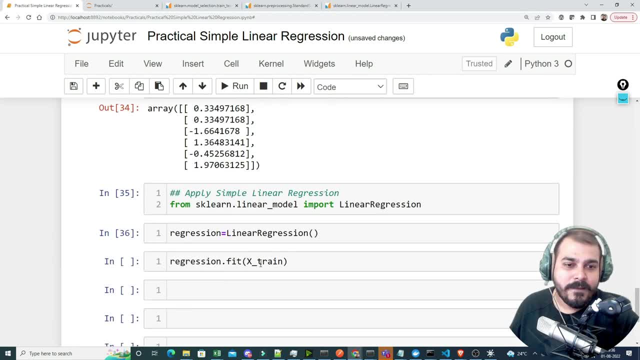 Now, instead of X underscore train, if I give this, what will happen? See, let's say, if I'm giving this and I'm giving Y because this had all the data, Now see what will happen. It will give us an error. 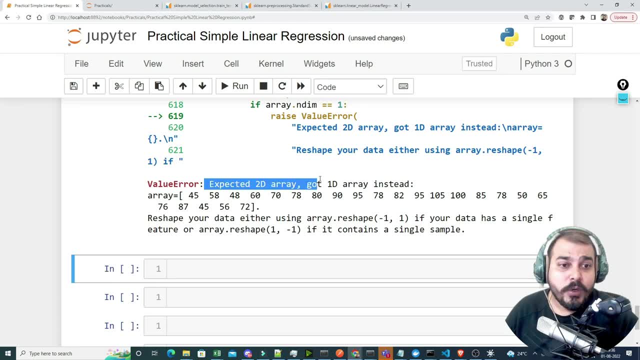 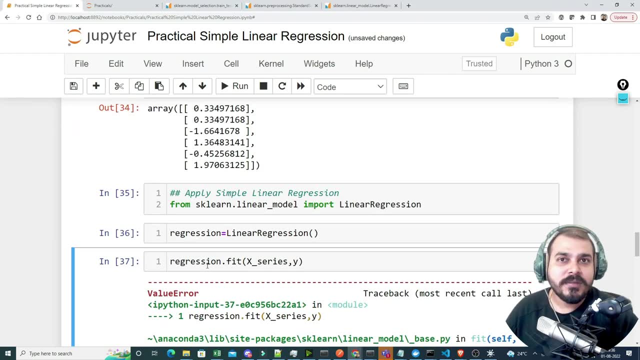 Why? Because it is saying that, except a 2D array, right, got 1D array instead, Right, And this was a 1D array, Right. So always remember any algorithm that you'll be seeing in the fit and whatever. 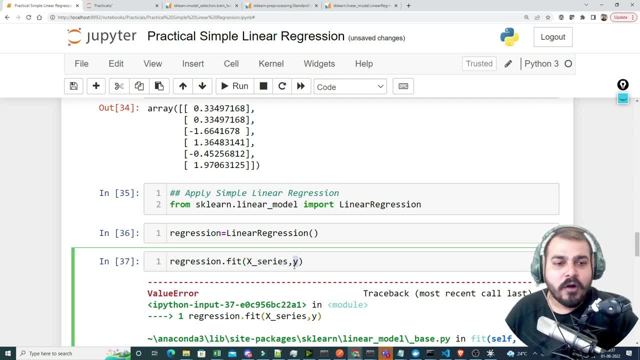 training data I am giving. it should always have a 2D array In the output. if you have 1D array, that is fine, Not a problem. But here you need to give it as a 2D array, OK, so here what I'm going to give now. 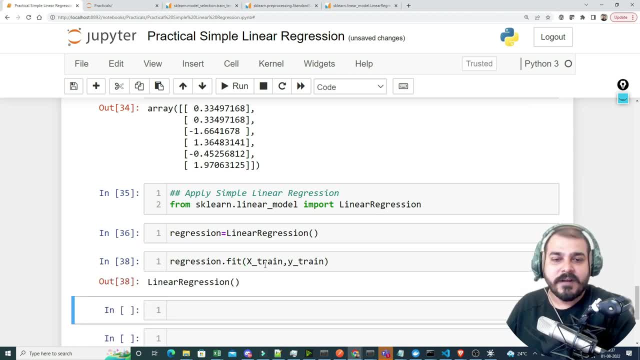 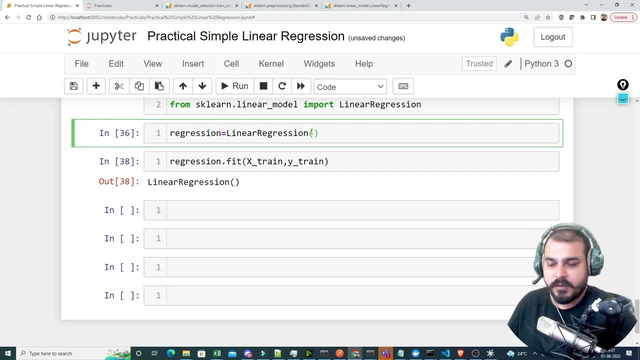 is the fit train, comma Y train. Now we will go and do the fit Now. once we go and do the fit now, let's see over here If I press shift tab. Sorry, over here if I press shift tab. 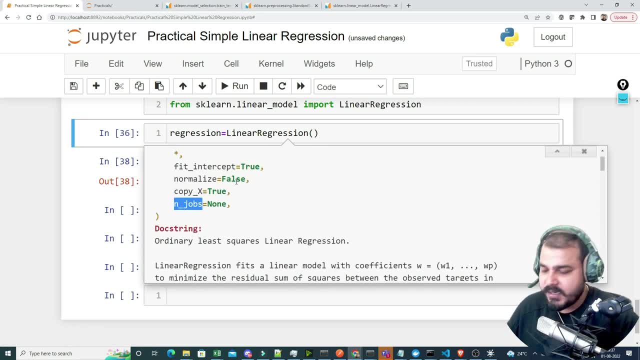 here you'll be able to see one parameter, which is called as N underscore jobs. Let's say it is none right now. Right, I'm just going to keep it as minus one, So what it will do. how many processors are there in my 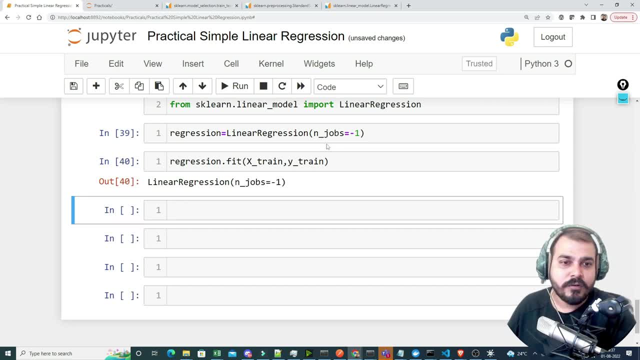 So how many processors are there? It will try to run it on them. So once I execute here, you can see that N underscore jobs is equal to minus one. Yes, you cannot see that because it is happening within the system Right now. if I probably go and see my regression now, 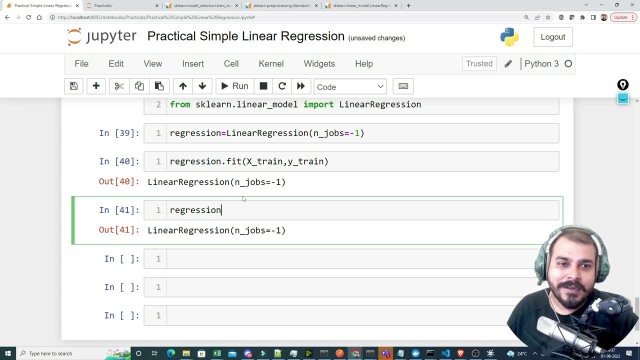 it is basically showing linear regression. Now all I have to do is that, in order to predict, or in order to predict my test data, how do I do it? So there will be a function which is called as predict, But before this, I already told you that how many different types of parameter it. 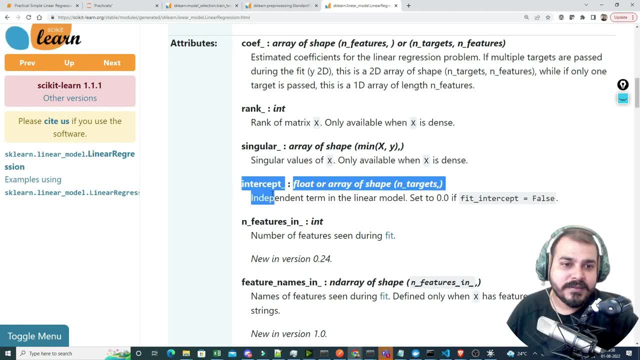 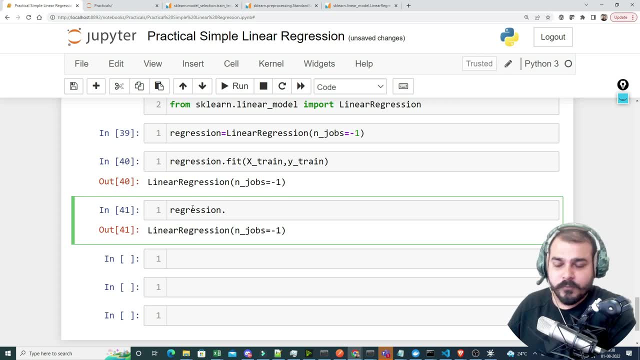 is running coefficient. coefficient basically means slope intercept and N underscore features rank and singular will not focus much into it. So let's go ahead and write the regression dot Here I will say coefficient. Now, if I go and execute this here, I'm going to get the coefficient. 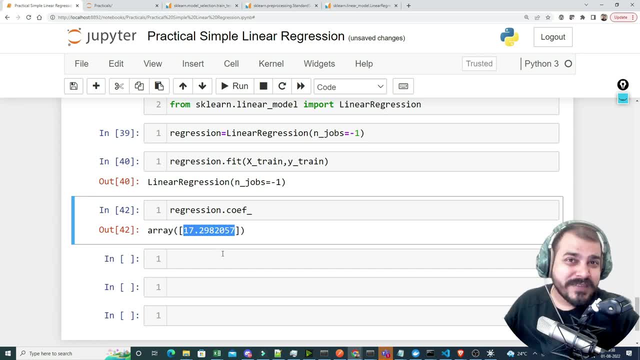 Now, this coefficient is the slope. And why only one? Because I just have one independent feature. Now, if you remember the entire equation, if I have one independent feature, so my equation will become: Y is equal to, or Y hat is equal to beta, zero plus beta. 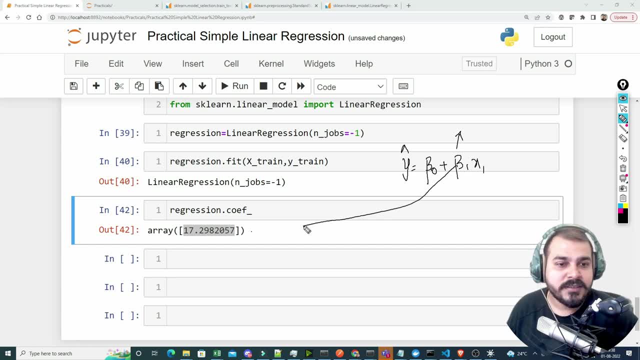 one to X, one Right, This beta one is nothing but this specific value. OK, And now I can actually also get this value, because I have already calculated the intercept and these are my data points In this particular case. this data points are nothing but weight. 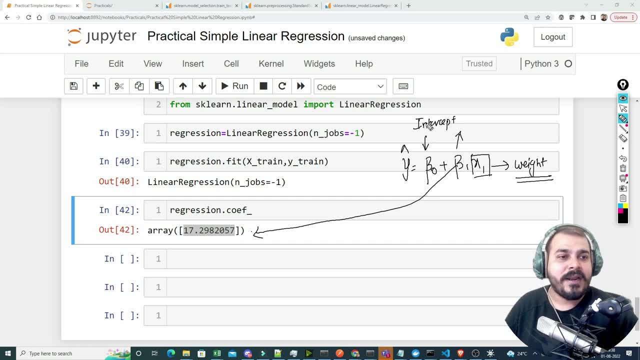 Right, So this data points are weight. This we have calculated. beta one intercept We will be able to get when we are writing the regression dot intercept underscore. OK, so here let me remove this quickly and let me show you to you, The reason why I'm using this, so that I 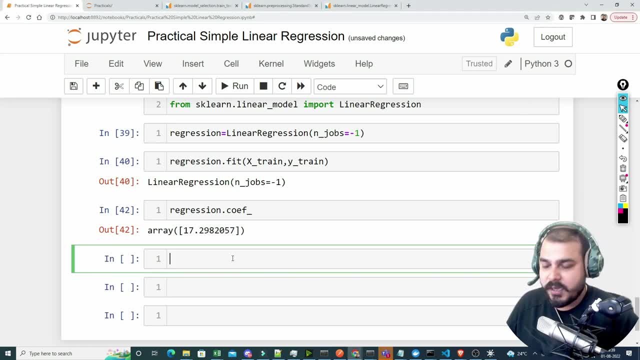 write anything in front of you, you'll be able to understand, OK. so here Now, this is my coefficient, So let me print my coefficient. So here I'm just going to say: Coefficients or slope is nothing, but is this specific value? 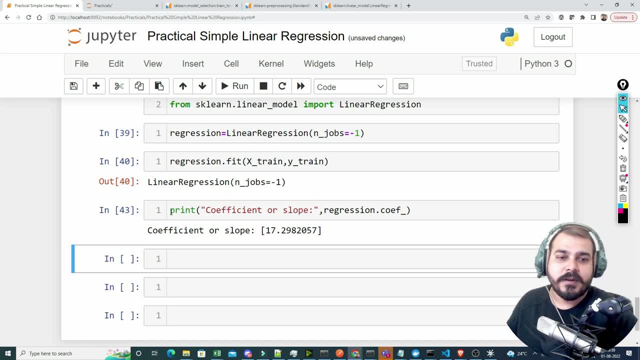 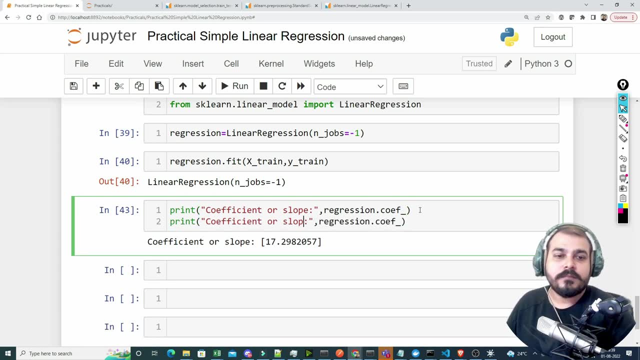 comma regression coefficient. OK, so here I have just printed it. Similarly, I can also print intercept. So I'm just going to copy this and write: print over here, Intercept, And I'll talk about this. what is the meaning of this? 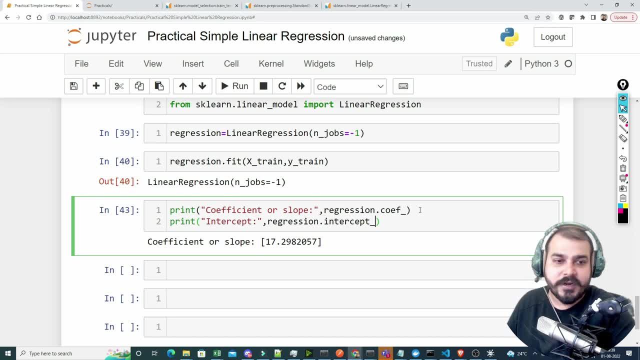 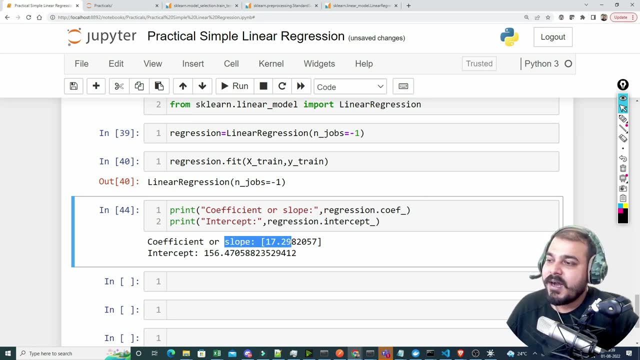 So intercept is equal to this will nothing be. I will just write intercept underscore. So this is my intercept and this is my slope. Now, what does this be With respect to this? OK, now, super, super important. That basically means one unit movement in the weight value. 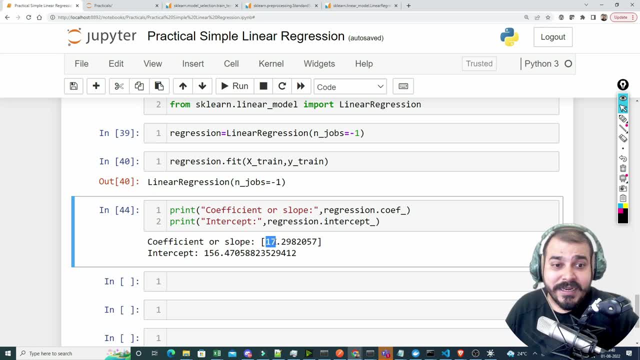 Let's say, one unit movement in the weight value. that leads to seventeen point two, nine unit movements in the height value. That is what it basically says, This coefficient. I can understand this one unit movement. OK, let me just draw it again in front of you. 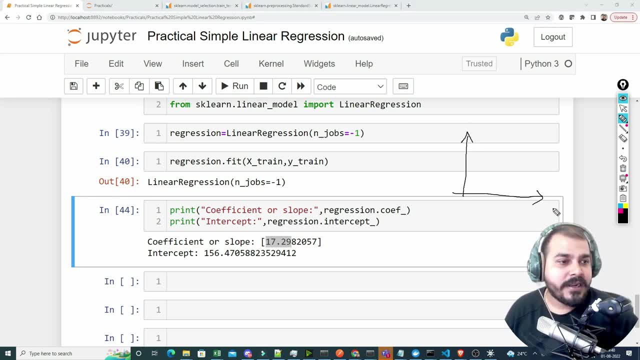 Suppose this is my X and Y, This is my weight and this is my height. Right, This is my height. It basically says that one unit movement with respect to the Y axis it leads to seventeen point two, nine unit movement. So from here to here, basically, this is seventeen point two, nine unit movement. 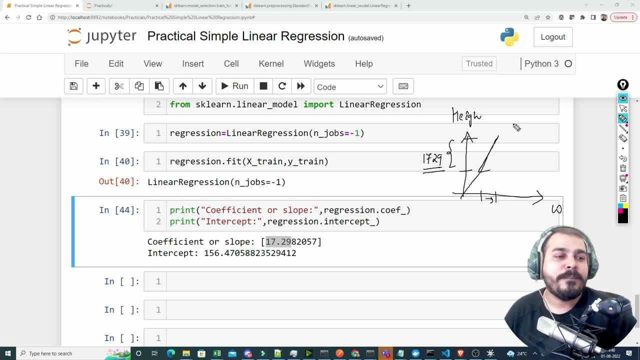 OK, with respect to the Y axis. So this is what this probably will look like- my slope, OK. so this is what we are doing. And the next point is that: what is this? one fifty six. One fifty six says that when your weight value is zero, 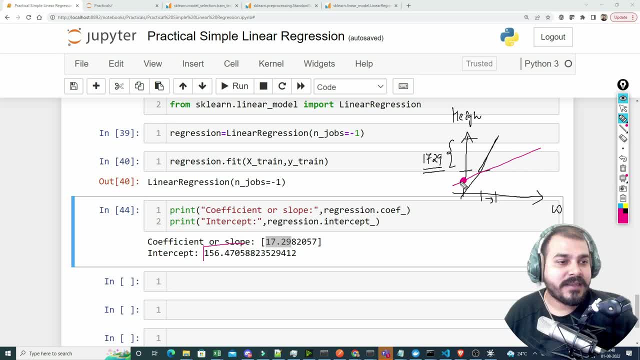 when, at what point your line is meeting in the Y axis. So this particular point is nothing but one. fifty six point four, seven. So I hope you have got an idea about it. OK, the importance of coefficient and slope. OK, and let me do one thing apart from this. 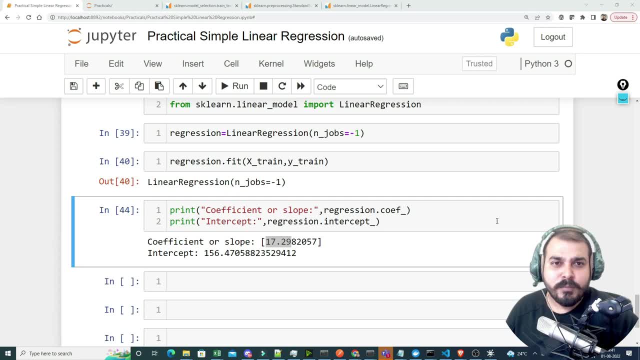 Now you have got your coefficient and intercept. Now you may be thinking, Krish, OK, fine, you have created this. Can we see some kind of line? So suppose, if these are my data points, can we see some kind of line which I can see it as a best fit. 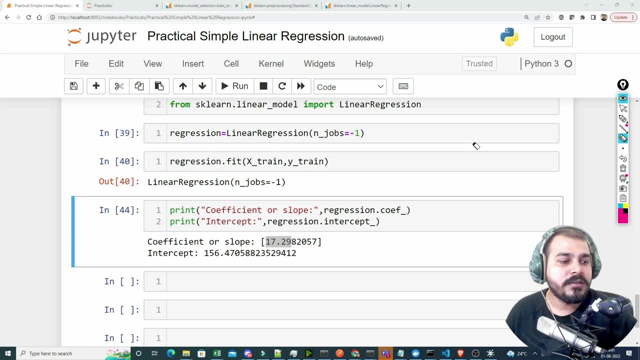 The answer is yes, and I'll show you that. So let's go ahead and plot this particular point Right? So here I'm going to plot the training with respect to training data. I'm going to plot Plot best fit line. 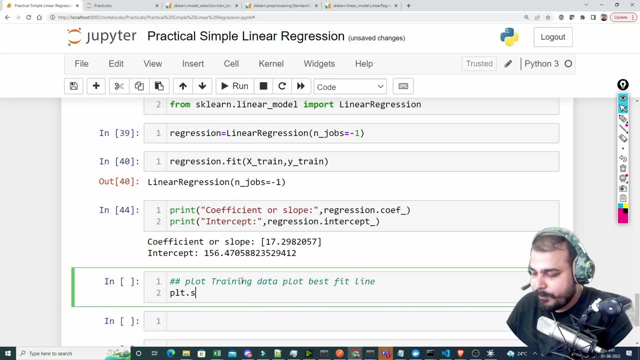 OK, So here let's go ahead and plot it. So first of all I will say PLT, dot scatter, And here I'm going to scatter my X train and Y train data. OK, so what will happen if I plot this? 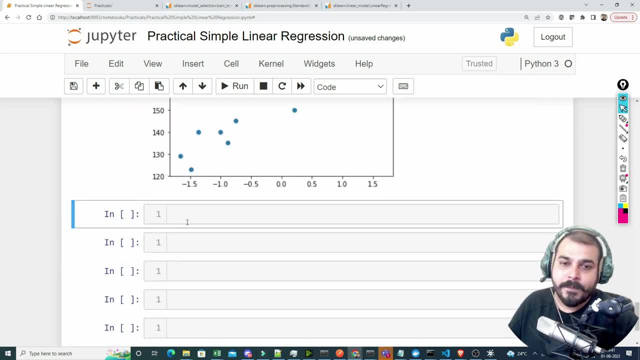 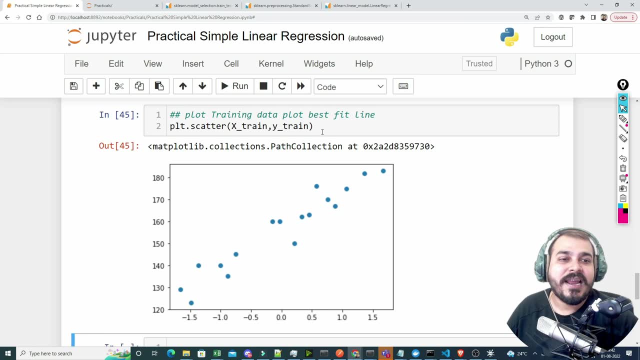 Here you'll be able to see this kind of plot. OK, let me make some more fields. OK, so here you can definitely see some plotting happen right on top of it. Now you want to see how our best fit line is created. 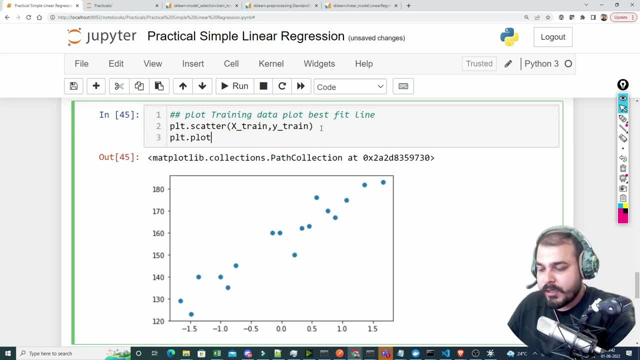 Then what do I do? I will go and write PLT, dot, ERO, T plot. This plot is also used, So here I will be taking X train, and we know that how to find out a predicted value Right now, in order to find out the predicted value. 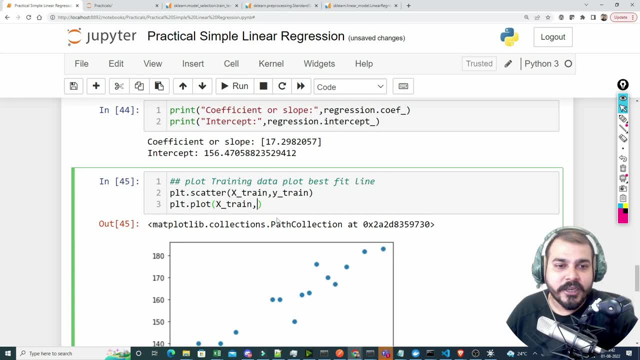 all I will be doing is that I'll take this model. OK, this model is regression. So here I'll write regression dot predict. OK, and here I'm specifically giving what value over here. See, if I write regression dot predict, here I'm going to predict for X train. 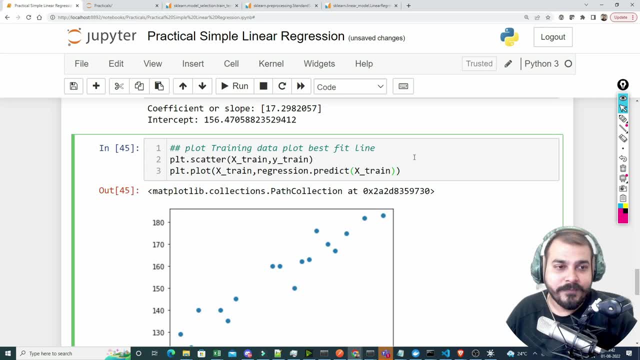 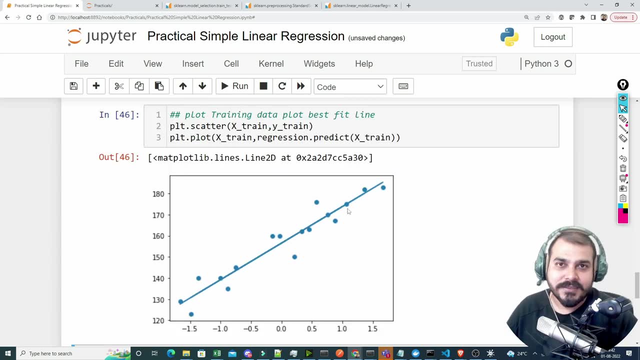 So this will basically give my predicted value, along with the straight line. Now, if I go ahead and execute this now, see, this is the best fit line that has got created in the specific data set Right, And this best fit line will have. 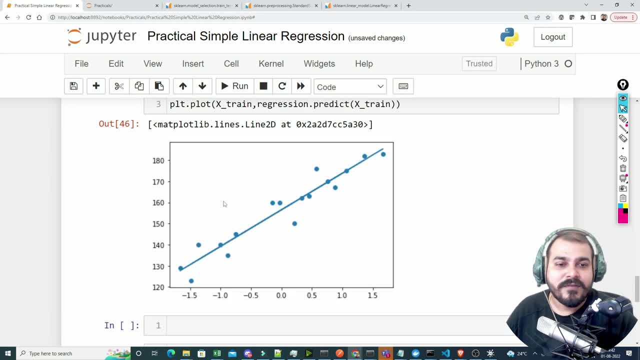 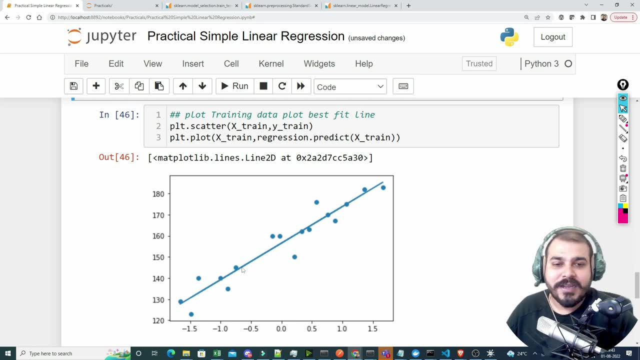 an coefficient of seventeen point two, nine and intercept of one fifty six. Because see if I probably, if I probably try to, you know, make sure that I extend this when my value is zero, then we are actually going to get an intercept of one fifty six. 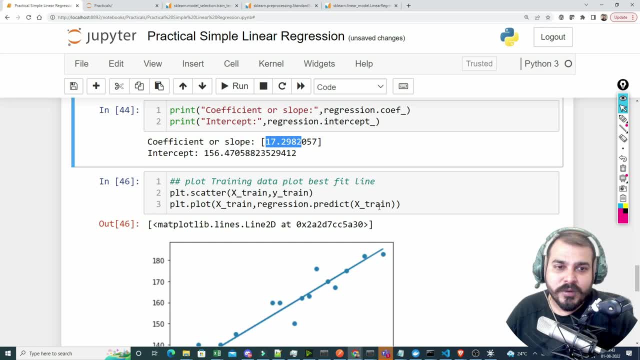 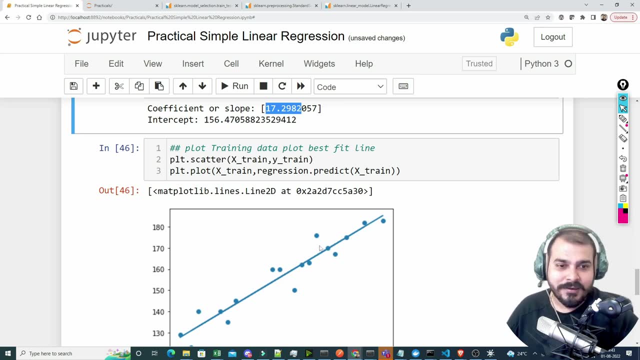 OK, so this is what it basically says with respect to this. OK, so now here You can see I've got my best fit line. And with respect to this particular best fit line, we are able to see that. OK, the the error also looks very less right here. 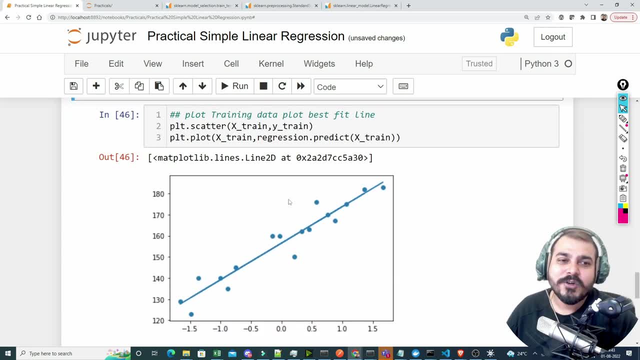 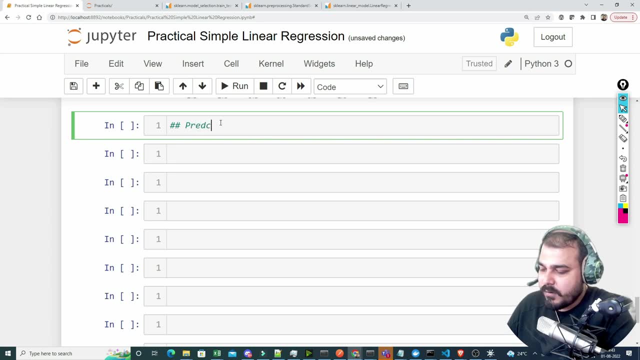 You can definitely see. the error is also very, very less. Now let's go ahead and let's go to the next step. Now we need to do the prediction for the test data Now in order to do the prediction for the test data prediction. 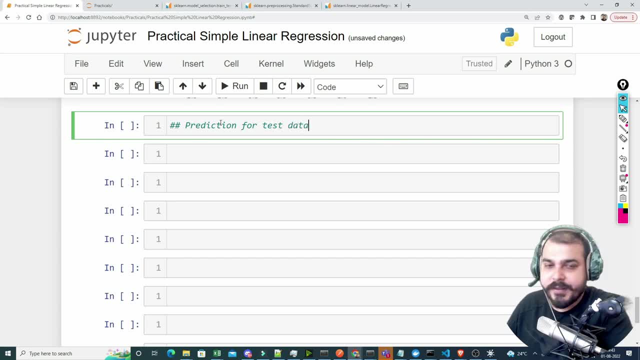 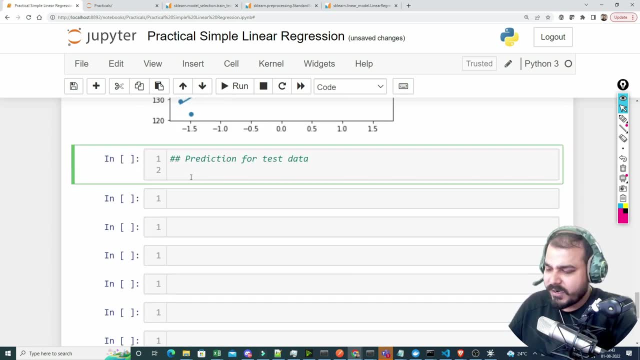 for test data. how do I do for the prediction for test data? So here you'll be able to see I will be using plot dot scatter or no need to use plot dot scatter also. So my model is something called as a regression dot predict on my X test. 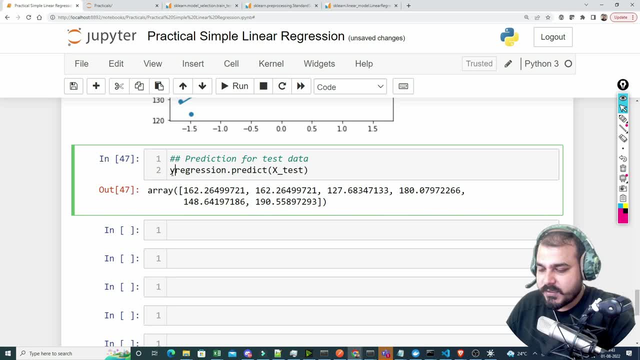 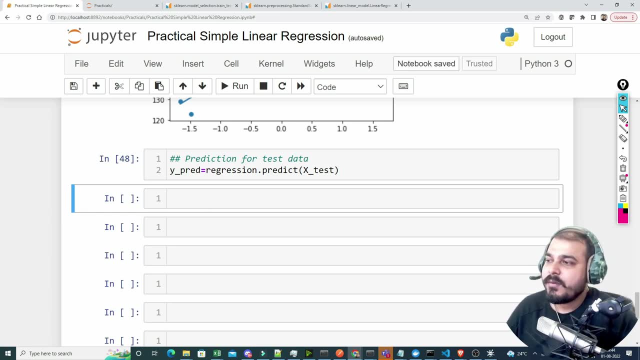 Now here, when I do the prediction, this is my predicted value, So this will basically become my Y underscore print. OK, so let me just execute it Perfect Now in order to see how the result is. you know how the result is. we will try to now check with some of the performance metrics. 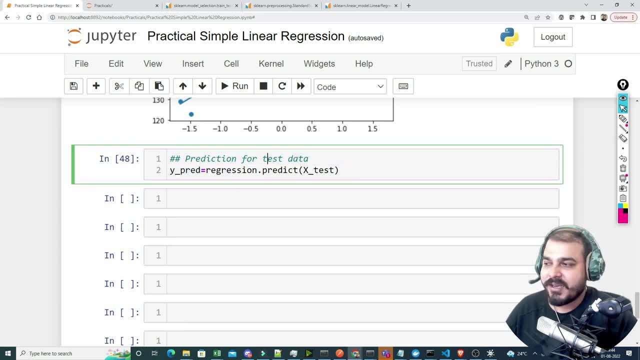 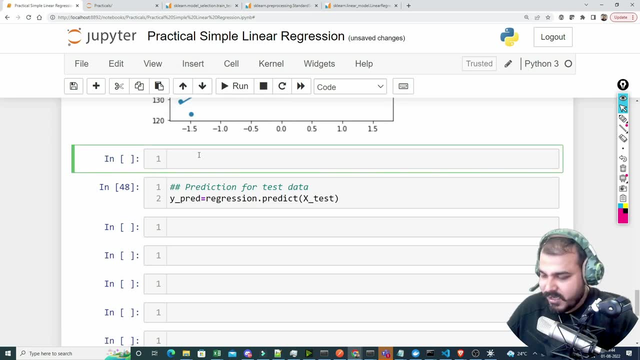 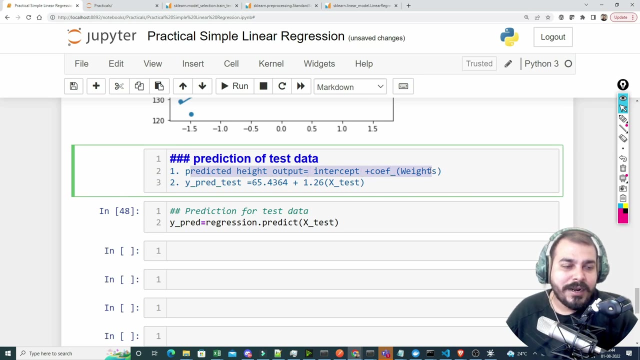 But before that, if whenever I do prediction for test data, right, I will just go and copy this thing. OK, just let's see. I hope everybody will understand it. Let's say I'm keeping a mark down over here. Here you can see the predicted height. output will be intercept plus coefficient multiplied by weights. 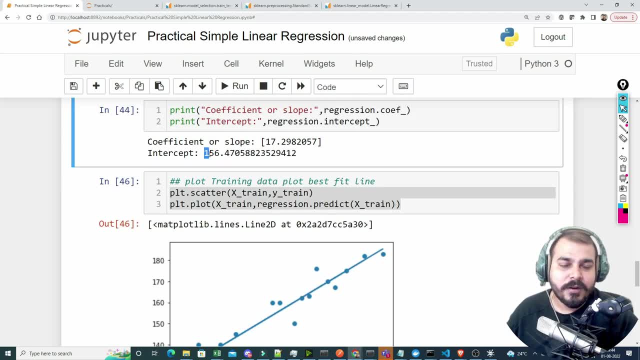 Right. So right now, what is my intercept? My intercept is nothing but 156.. OK, let's say this is my value. OK, so I'm just going to copy it over here, And my coefficient is nothing but 17.29.. 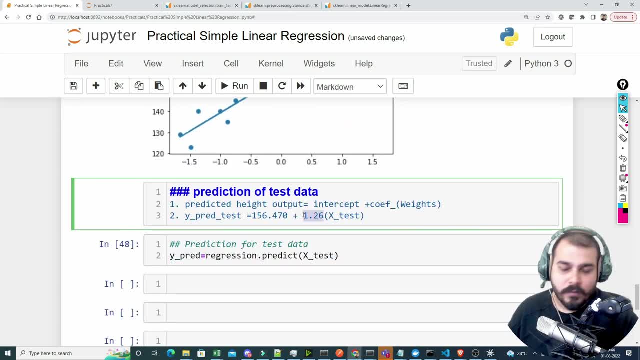 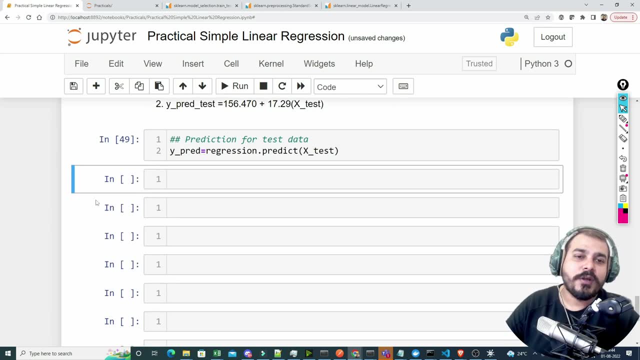 So I'm just going to copy this and paste it over here. OK, so this is what is basically happening in order to find out all my Y print. OK, so here I'm just going to execute it, So that will give you an idea. 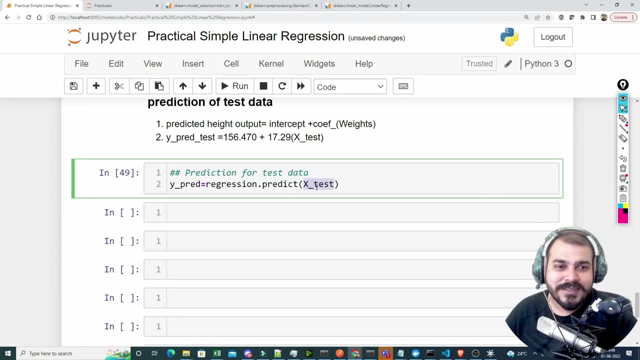 OK, so I hope everybody is able to understand this already. This understand X test data is already transformed also. OK, if you don't know now, let's go ahead and do some more things in this. Fine, We have done the prediction. 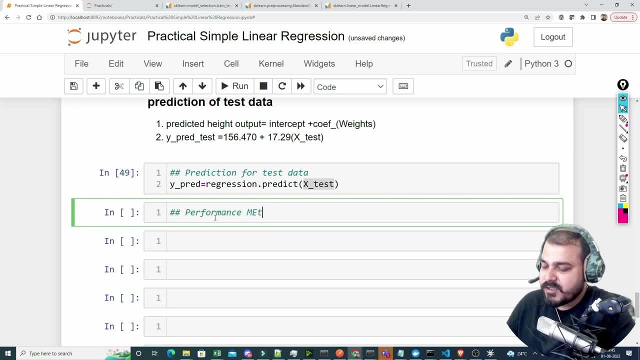 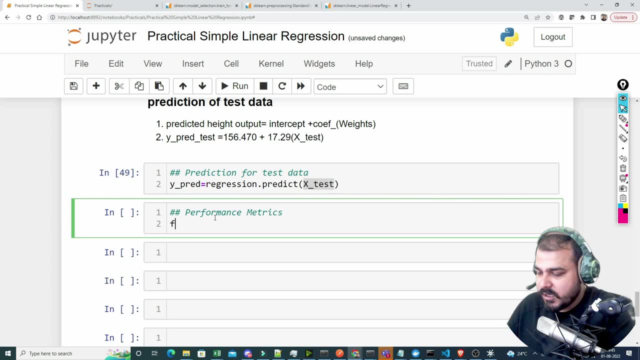 I will focus more on this. I will focus more on the performance Now, which all performance metrics we have already discussed that we are going to see. So in this I'm just going to write the performance metrics that I have actually discussed. 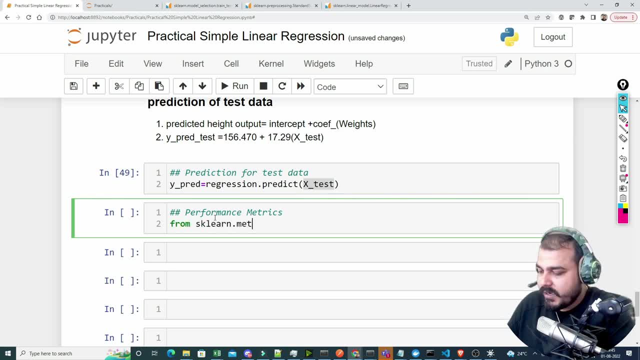 I'll write from sklearnmetrics I'm going to import. the library that I'm going to import is something called as mean squared error. So here you have: mean absolute error, mean mean squared error. OK, There are also many, many other performance metrics which you can also use. 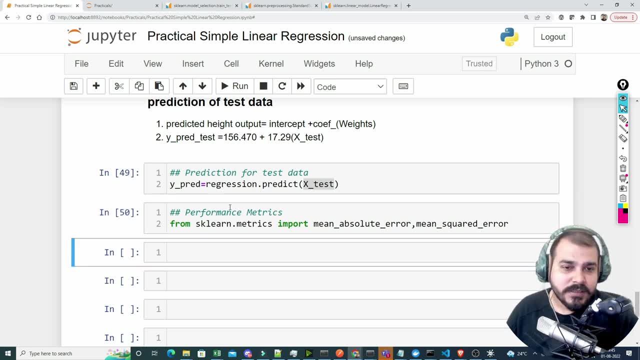 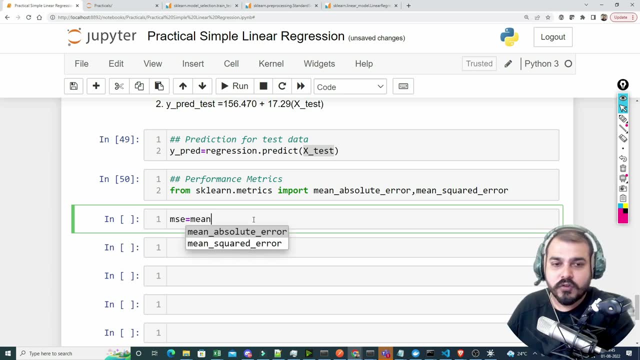 Right, For right now I'll just use this because we have learned about this. OK, And then what I'll do? I will basically calculate my MSE mean squared error. So here I'm going to write mean squared error And here I'm going to give my Y underscore test. Y underscore print. 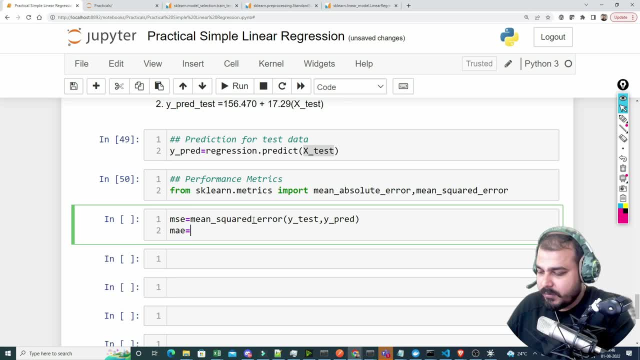 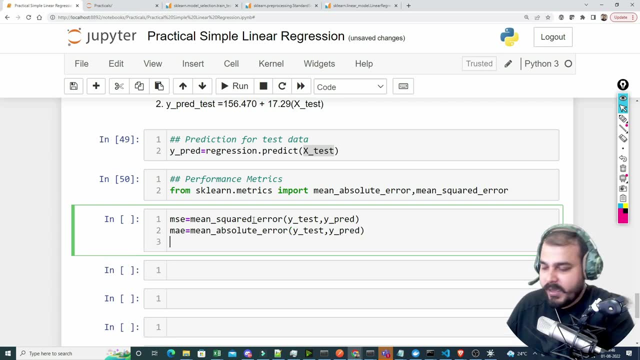 So this will basically give my MSE. Similarly, MAE is nothing but mean absolute error, And this will basically give my Y underscore test, Y underscore print And finally, root mean squared error, which is nothing but NP dot, square root right of MSE. 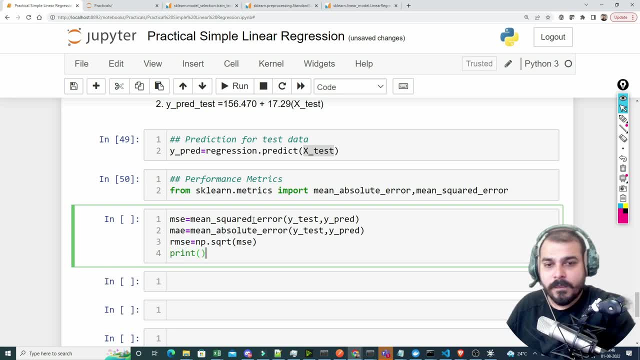 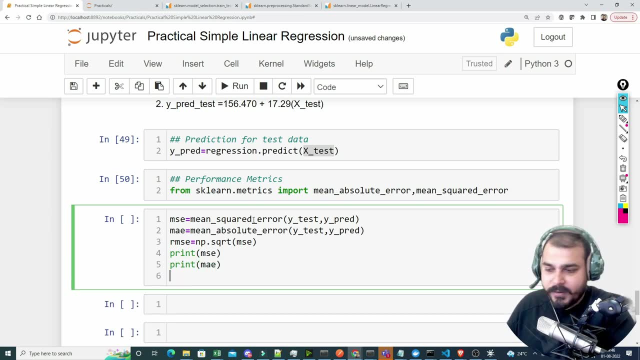 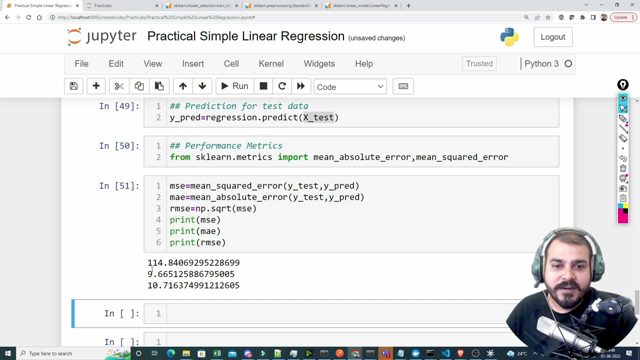 Then I'm just going to print MSE, print MAE and then print RMSE, As I said that we really need to check all the parameters over here Now, here you can definitely see that 114.84 is your mean squared error. 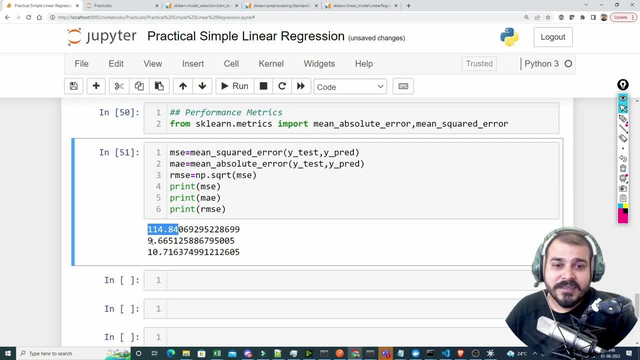 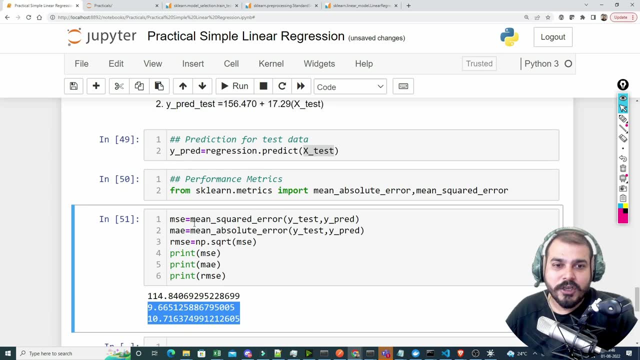 Definitely it has penalized a lot of outliers, you know, whereas in this case- here you can see it's almost nearby- by using mean absolute error and all OK. so here this is what we have actually got with respect to our performance: error metrics. 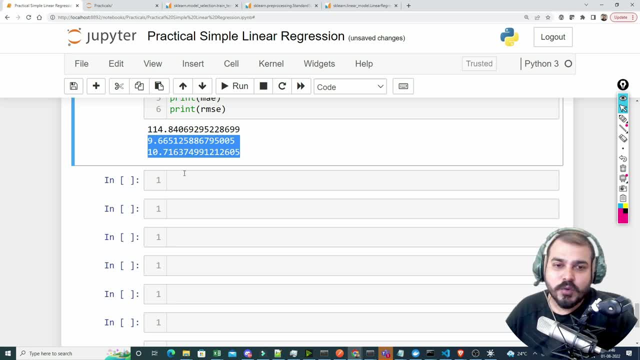 Now, the next thing that we are going to use is something called as R square also, So R square. if you remember the formula for R square, how we are going to use the R square, So here I'm just going to copy and paste the entire formula for you. 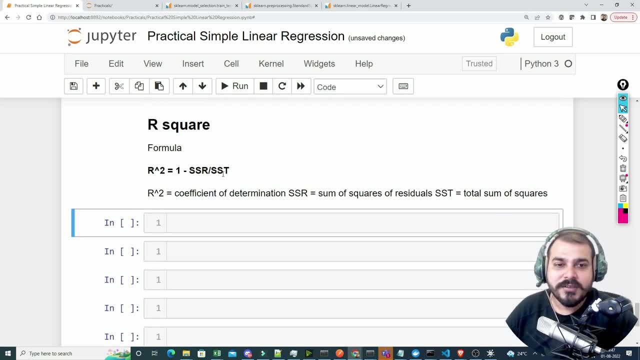 We have already discussed about this. There's nothing but one minus sum of square residual divided by sum of square total right? So here, this is the formula that we'll apply. in order to apply Also. we can also use this from my library. 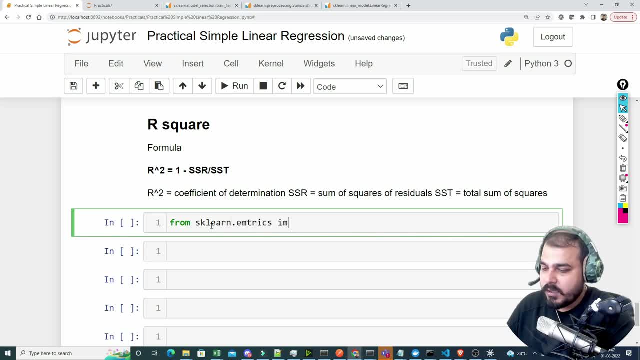 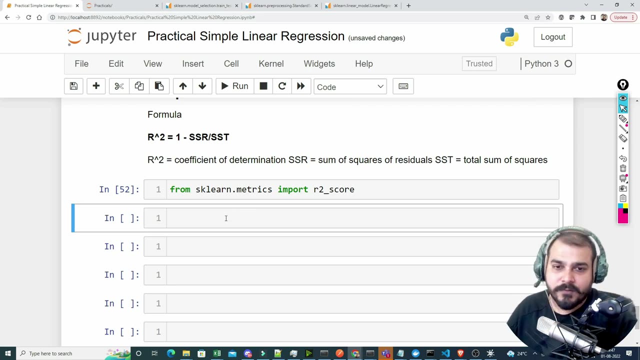 So I'll write from sklearn dot matrix: import R to score, R to score right, so it should be matrix OK. So this also will look good because now overall we'll be able to get how our model is performing. So finally, my score will be. 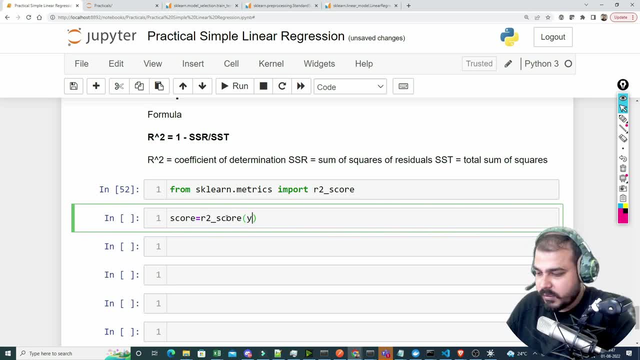 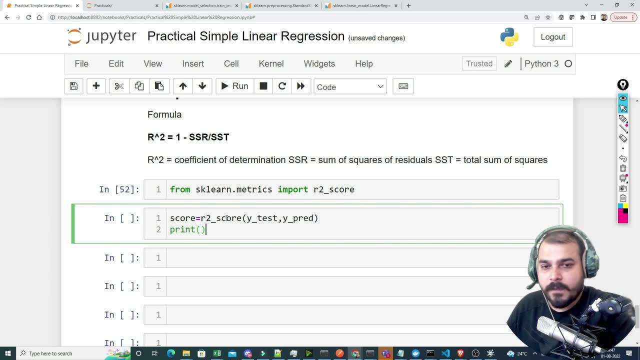 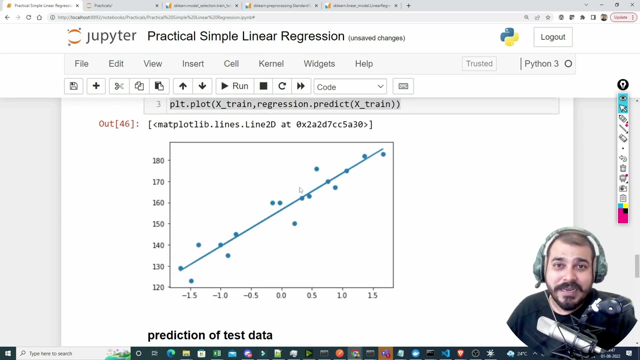 equal to R2. underscore score is nothing but Y underscore test, Y underscore pred Right And if I probably print my score, this will be my R2 score. and here I'm getting 73 percent. And obviously you cannot get a perfect just by linear line. 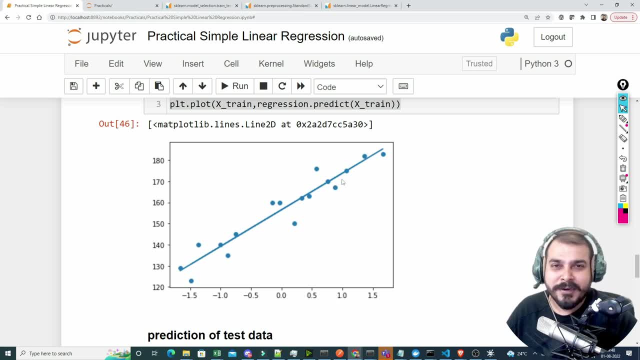 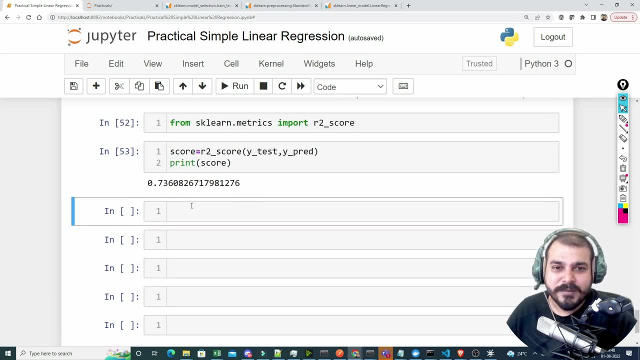 We'll be seeing how we can improve this by using some of the algorithms like polynomial linear regression, decision trees and all. Many algorithms are going to come up in the further stages which will try to improve this particular accuracy, But right now I'm getting 0.73.. 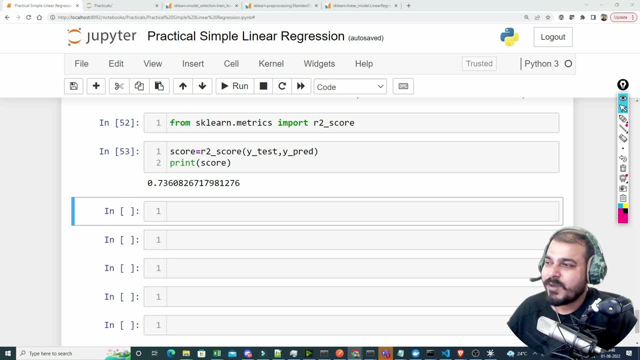 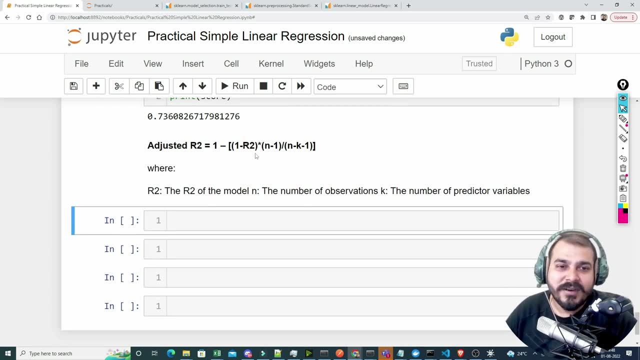 And obviously let's go and find out one more. that is called adjusted R-square And, as you know, adjusted R-square formula is this, which, again, I have discussed in my theory part right: it is nothing but 1 minus 1, minus R-square, multiplied by n minus 1. 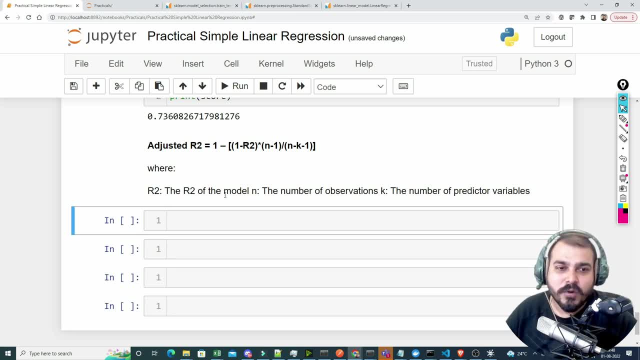 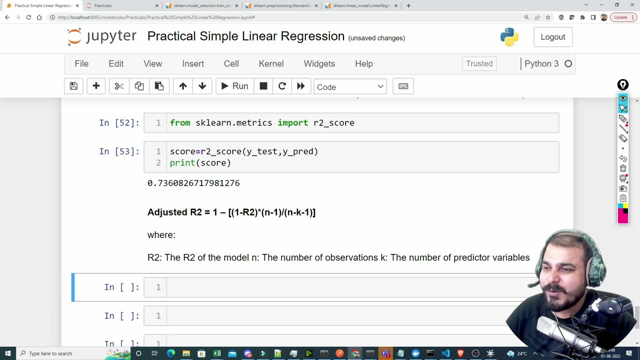 divided by n minus k minus 1, right, R2 is nothing but R2 score of the model, number of observation and number of predictor variables right. Right now I just have one predictor variable, so I don't think so it will be such a big issue. 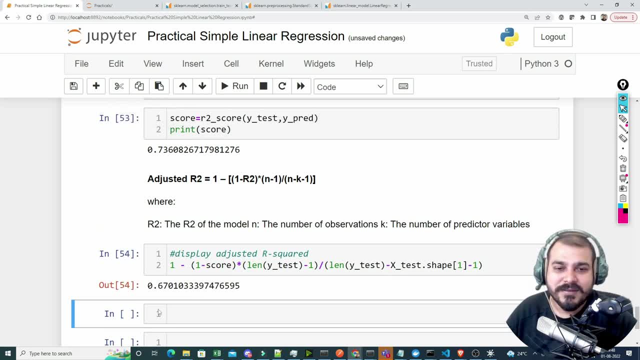 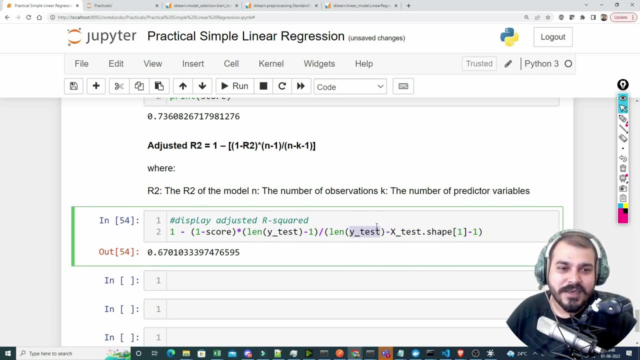 or a big change in the score. So if I probably go and see, it is like somewhere around 0.50,. OK, So I've just applied this formula where I've written 1 minus score, length of y-test minus 1, y-test is basically giving you the number of observation and all. 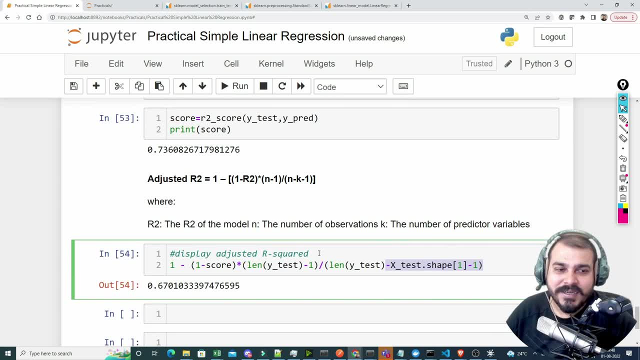 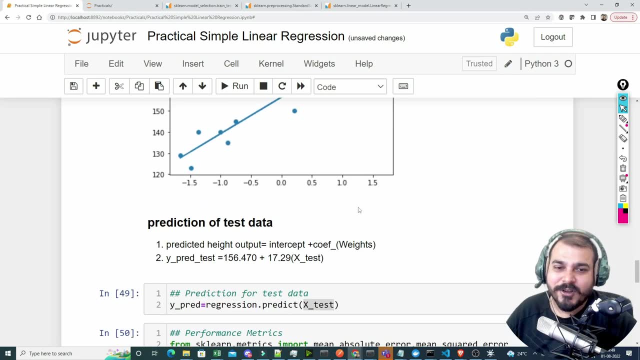 And this is the x-test and this is the other thing, right? So yes, I think I've covered all the most of the things over here. We have also seen that. OK, I've got 0.73, which is good. 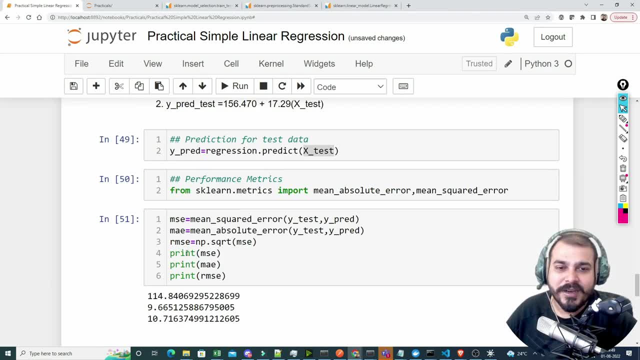 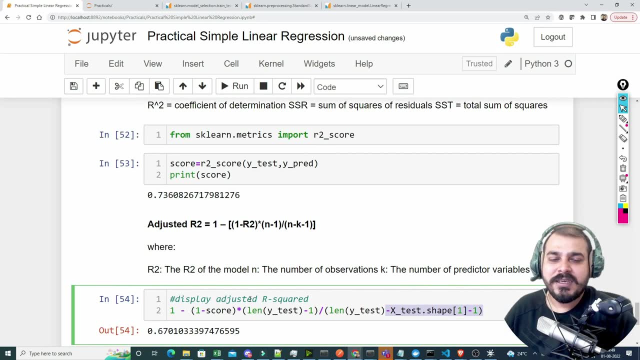 I've also seen all the performance metrics like mean squared error, mean absolute error, root mean squared error. This is absolutely fine. We have done some kind of visualization, analysis and all. Now let's try to see one thing. OK, Let's try to do the same thing with OLS technique. OLS: technique of linear regression. 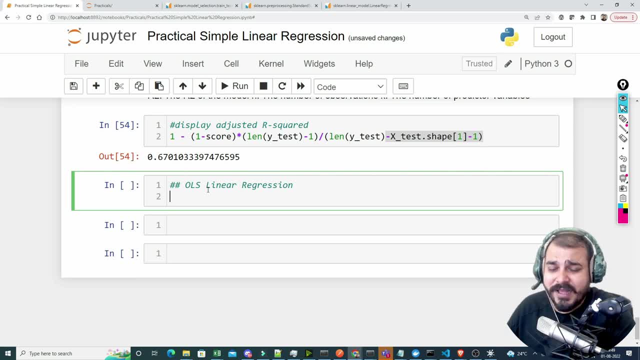 So can we get the same, because that formula that I derived right, can we get the same output that we are looking for. you know, In order to implement OLS, linear regression, I will say: import statsmodelsAPI as SM. OK, and I'm going to execute it. 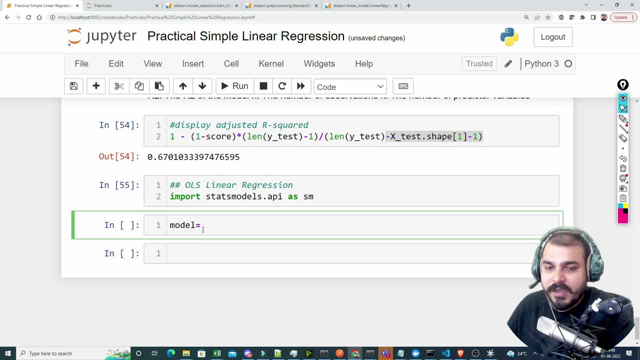 And now I'll just use my model- is equal to this model. will this API that I'm actually using right? This library that I'm using this has a library which is called as OLS, And you know, in OLS, all we need to give is with respect to your training data. 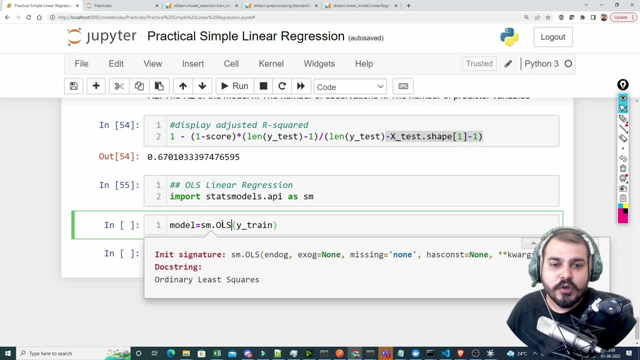 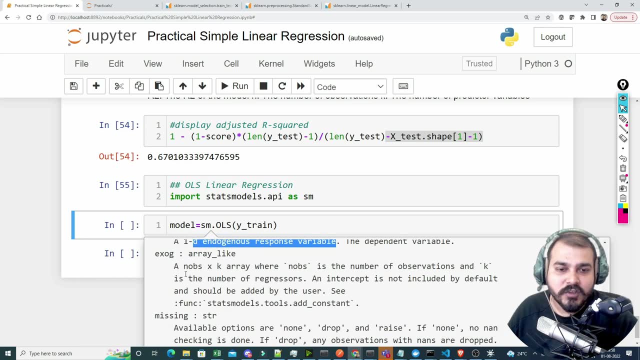 So if you probably go and see over here OLS, here you have something called as NDOG and EXOG, right? NDOG basically means 1D indigenous response variable, that is my output variable. EXOG basically means my true input variable, right? 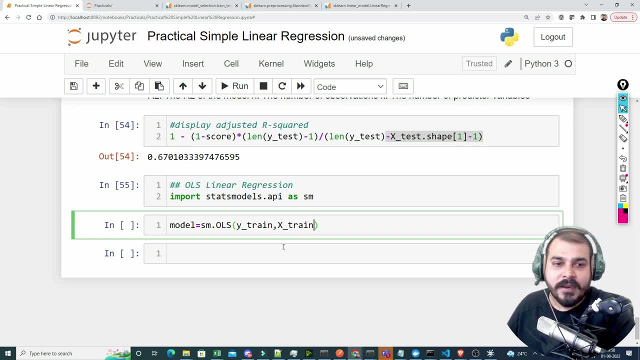 So here I'm basically going to give my xTrain and then I'm just going to do dot fit on this, like how we did for linear regression. Once I do this, I will get my model and all I have to do for prediction. 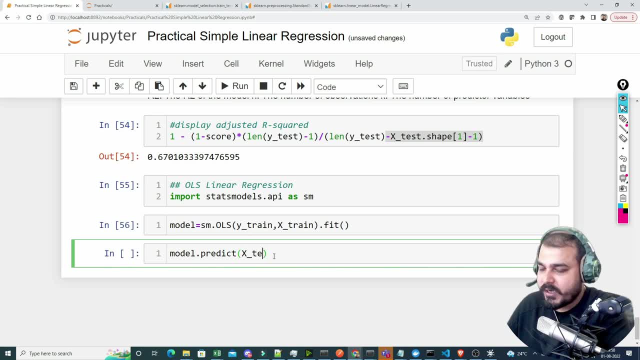 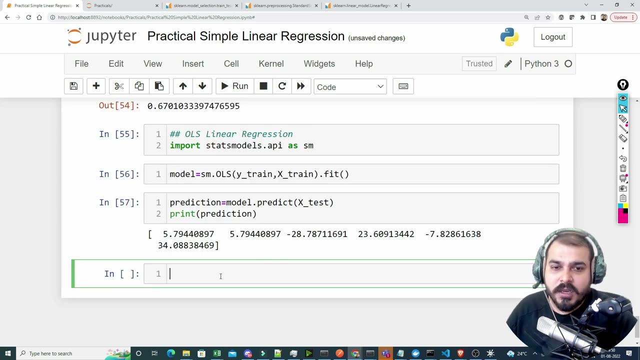 I will do model dot predict or X underscore test And this will basically give my prediction value right, This will give my prediction value. So if I probably execute this print prediction, you will be able to see the prediction also Perfect. So these are my predictions. 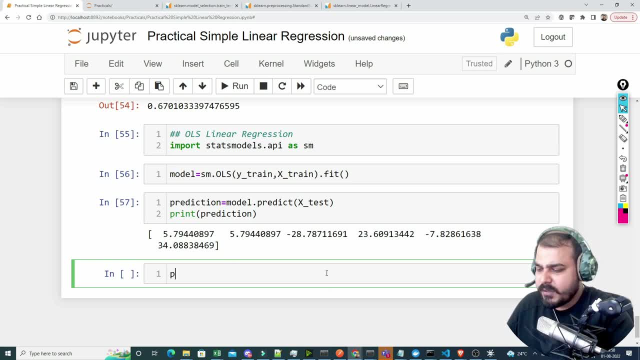 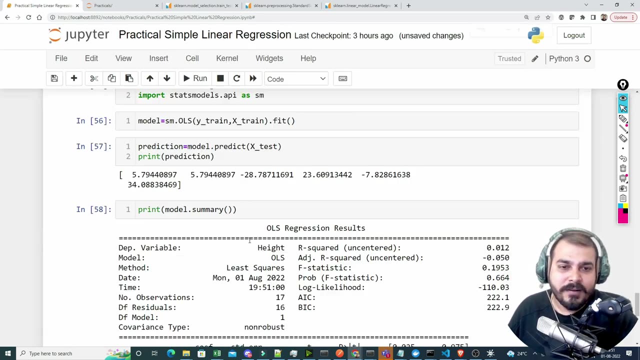 Now let's do one thing. OK, I'm just going to print my model summary over here, OK, In OLS, and see whether I'm getting the same thing what I did with the help of linear regression using gradient descent. So again, I'm printing this now here. I'll just zoom out. 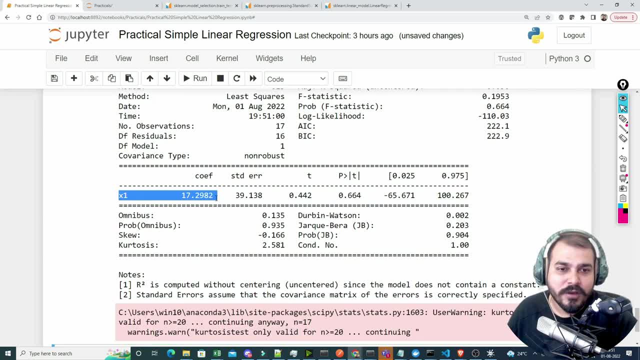 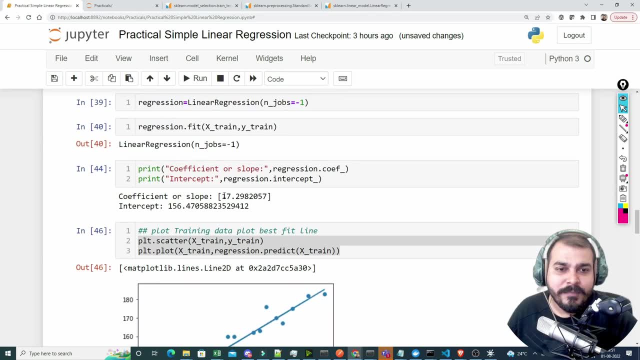 Here you can see that there is one feature x1 and it is having a coefficient of seven point two nine. Now is this matching with this or not? We'll try to see So if you go over here. here also, I'm getting coefficient as seven point two nine eight. 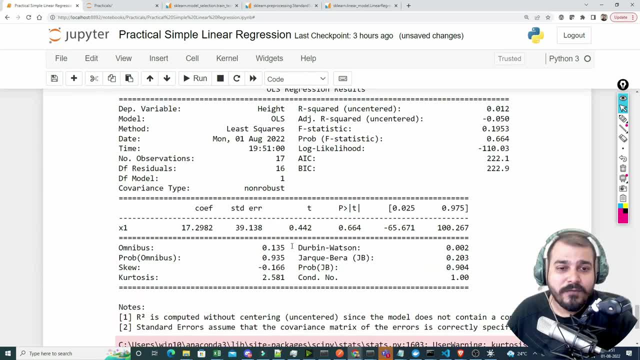 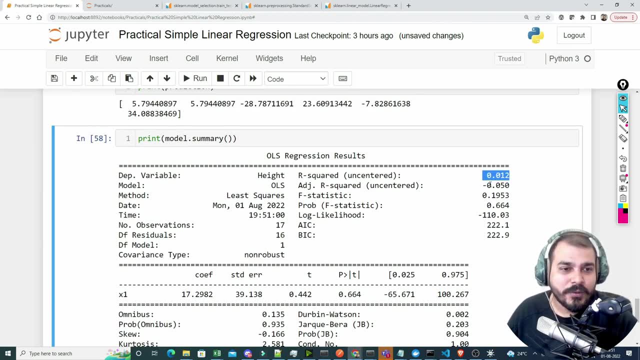 which is quite amazing. Now you can see the proof that, with the help of OLS also, I'm getting the same coefficient. and yes, there are some more parameters over here. right, They are like R squared value- adjusted R squared value, right. 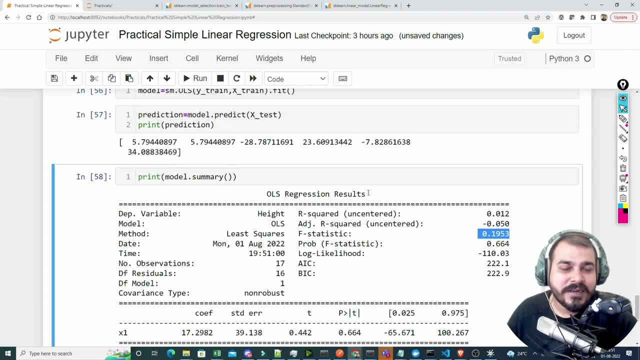 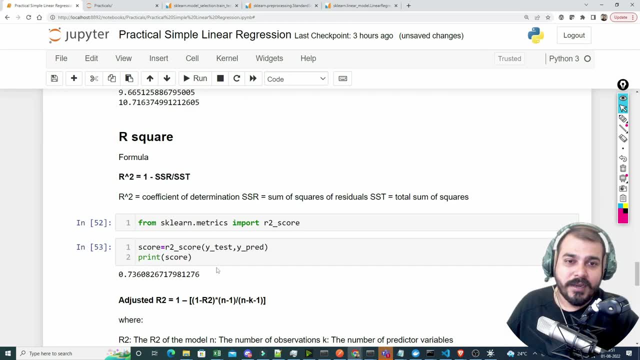 Statistics value, And this is specifically for uncentered centered data. It is not there, right. So all these things here. you can basically see that, But at the end of the day, we are getting a coefficient which is seventeen point two nine, which is approximately equal to this. 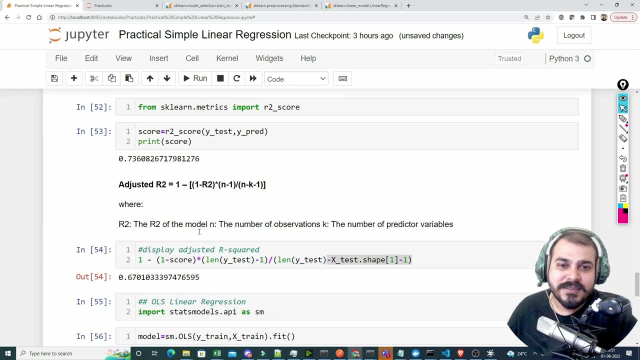 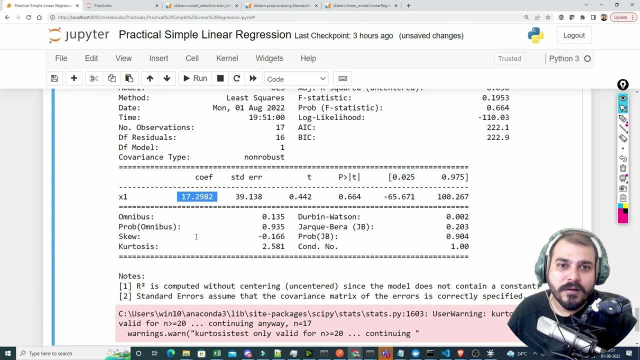 particular coefficient that we got with linear regression OK. so this is the most important point with respect to this. That basically means with the help of OLS also, we are able to get some good values Right. Good good, because almost all OLS and this SKlearn works in the same strategy. 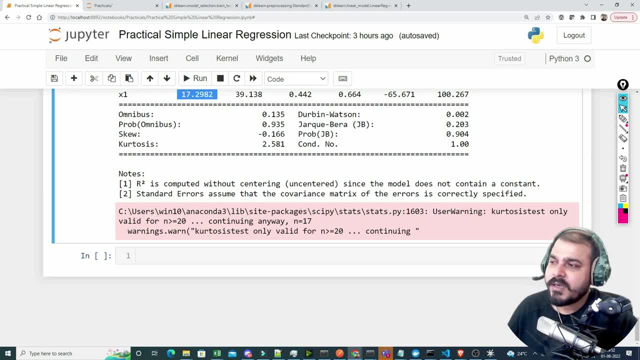 OK, now till here. we have discussed about so many things right now: What, how to do the prediction for the new data. So this is super, super important: Prediction for new data Right now. let's say that I get a new weight. 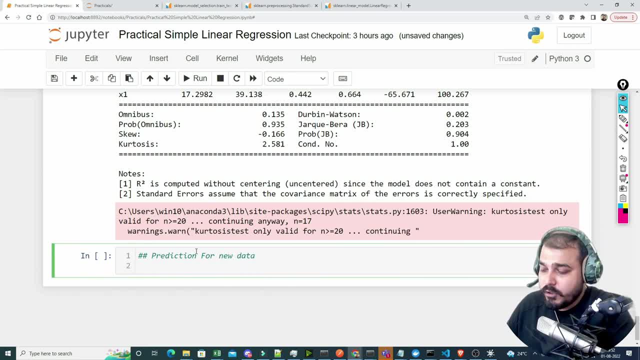 OK, let's say my weight value over here, And in order to do the prediction, I will write regression dot, predict and my new weight value, my new weight value. Always make sure this you are providing in two dimension again. Right, So it should be. let's say I want to predict it for seventy two weight. 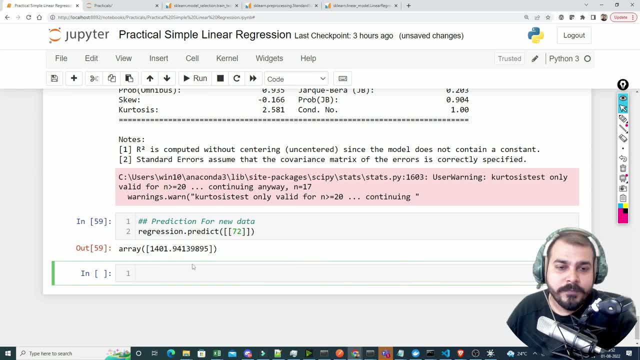 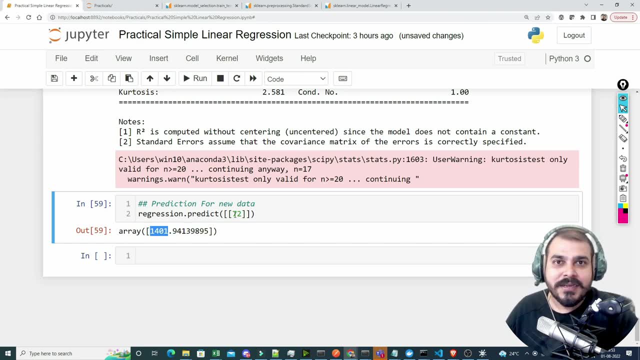 What should be my output. So here you'll be able to see the output. Now, guys, here you can see that, after prediction to showing one four zero one, Oh my God, This basically means that a person who is having a weight of seventy two 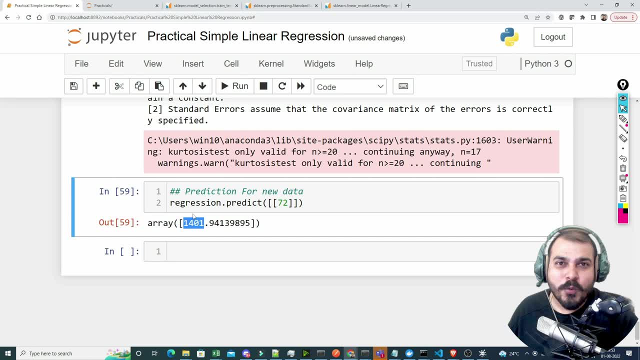 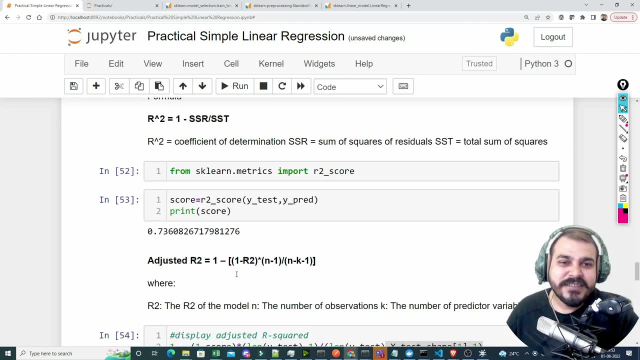 is getting a height of fourteen zero one centimeters. So what mistake did we do? You know why it is basically giving this kind of output? The answer is very simple, guys: We missed a very important step, which is called as standardization. 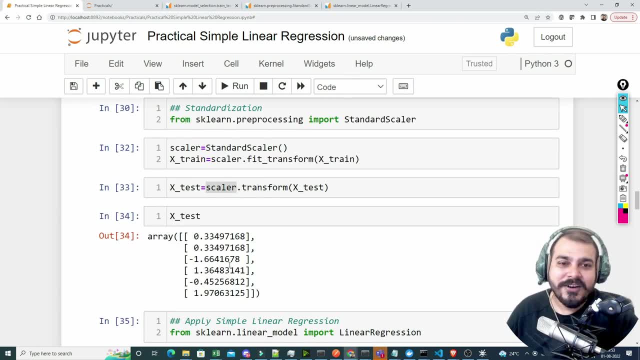 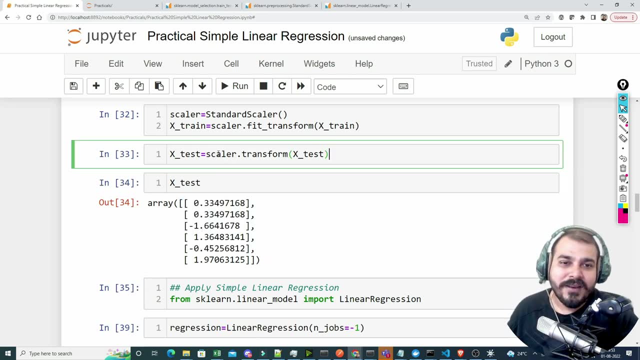 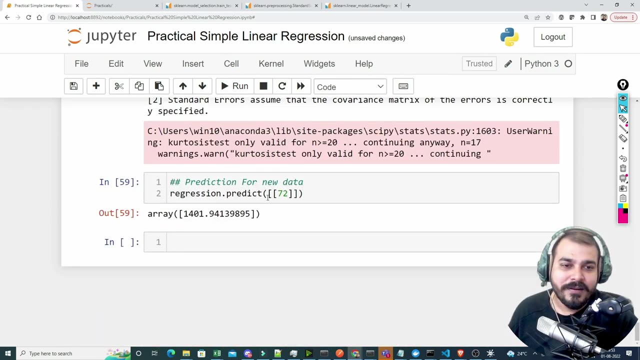 See, we did this Standardization Right, And right now my data points are not, you know, standardized down or normalized in this particular range, Right? So what do we do? We will again use scalar dot transform. So here I will just copy this and I will write over here: simple scalar dot. 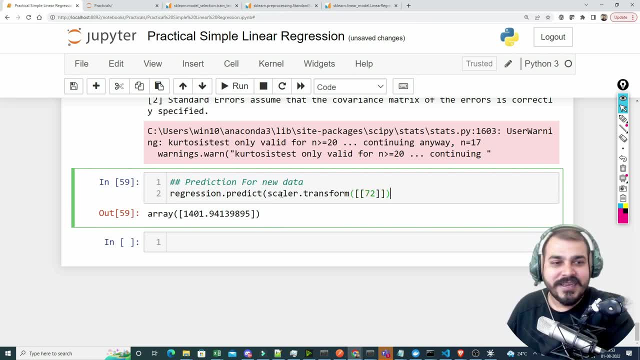 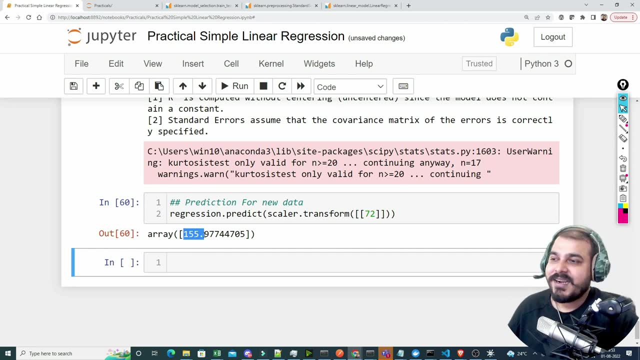 transform and I will give this value inside, this Now. once I give this value inside, Then you will be able to see I will be getting a good value. So now this is the correct output with respect to this particular data Right Now. just imagine, if you did not remember. 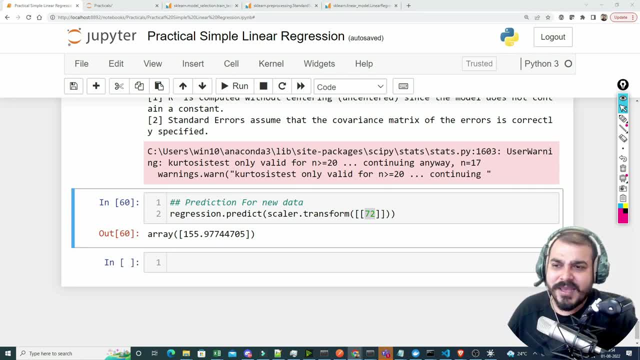 that scaling part, you would have worried, right, Krish. what happened? Why am I getting such a high value, Right? So always make sure that whenever you are doing some kind of predictions- OK, you have to make sure that this problem. 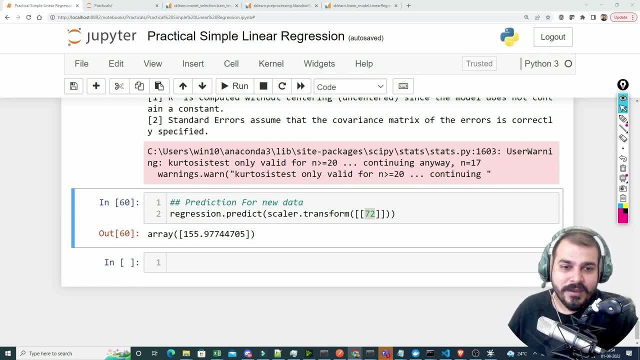 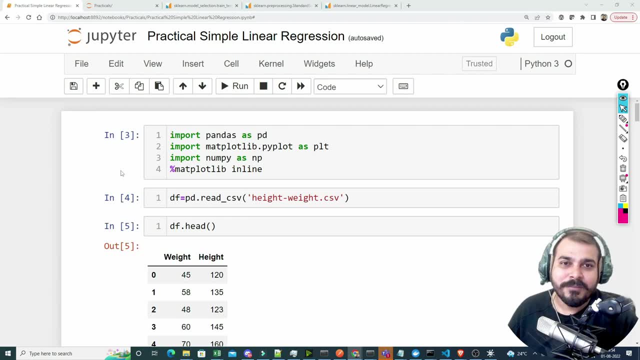 this scaling transformation needs to be always done. OK, so this is super, super important Right Now. this was all about this. you know the entire linear regression model. This is a simple linear regression model where we took a simple data set. 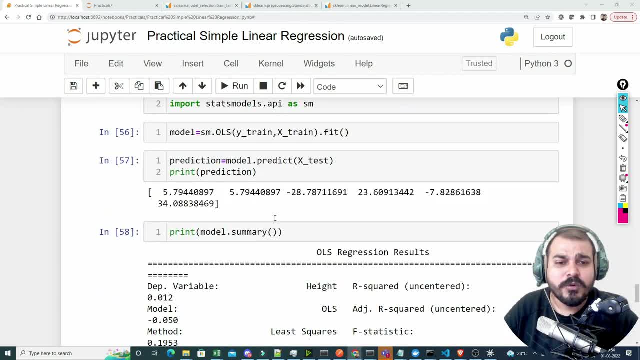 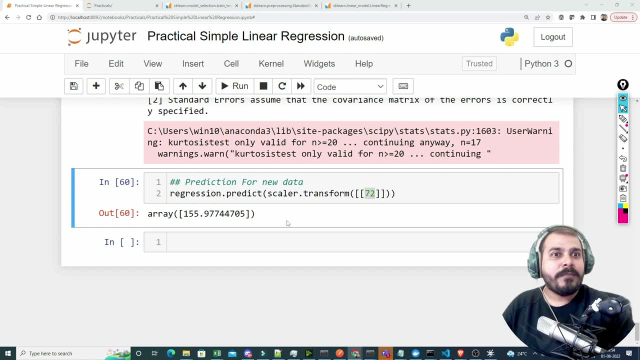 and we tried to see much and much more of information and we tried to do the prediction. So I hope you have understood this. In our next video, we are going to see a problem statement where we have multiple features and we'll try to implement multiple linear regression. 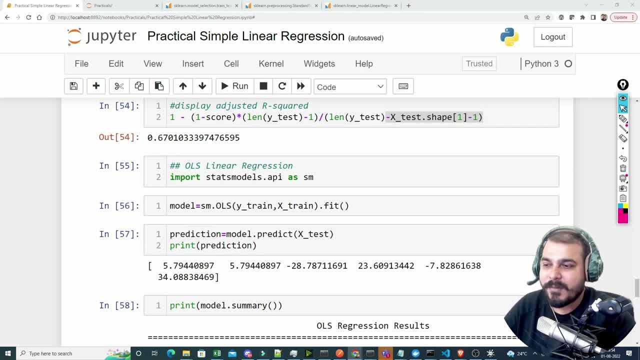 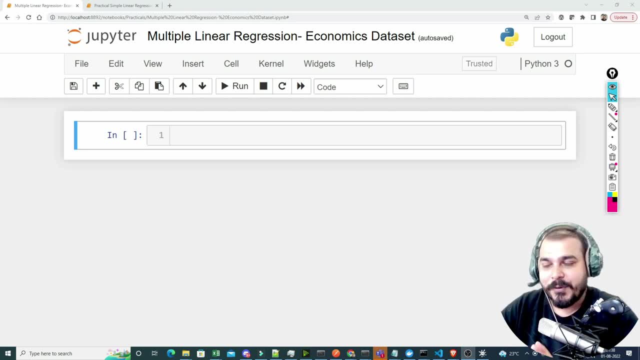 And we'll also try to see with this OLS whether we will be able to get the same output or not. So this is our second project And in this project we are going to solve a use case using multiple linear regression. Now, whenever I say multiple linear, 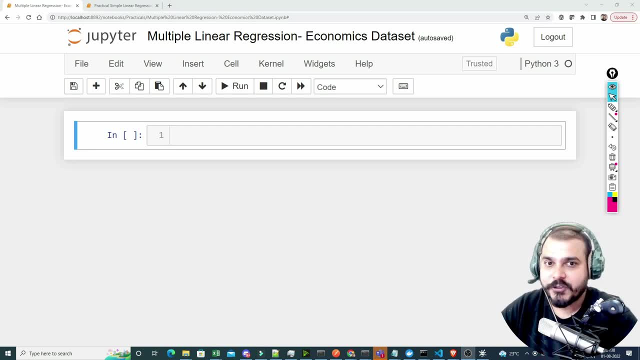 regression, that basically means I will have at least more than one independent features. OK, so for this I will just increase the complexity more when compared to the previous one, and the data set that we are going to use is something called as economic underscore index, dot, CSV. 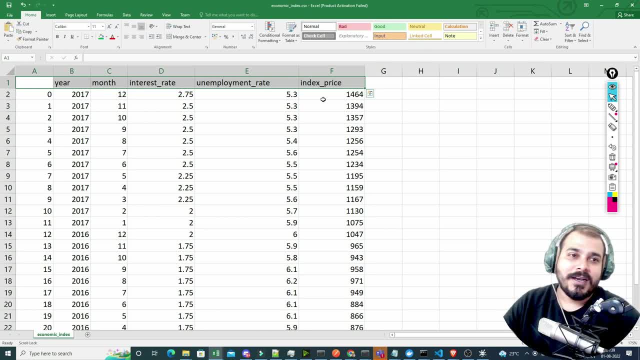 And again, this particular data set I have actually prepared by seeing some of the stats information- I'm not taking the complete data set, but at least 25 records from there And we'll understand how we can implement multiple linear regression on this particular data set. Let me talk more about this particular data set. 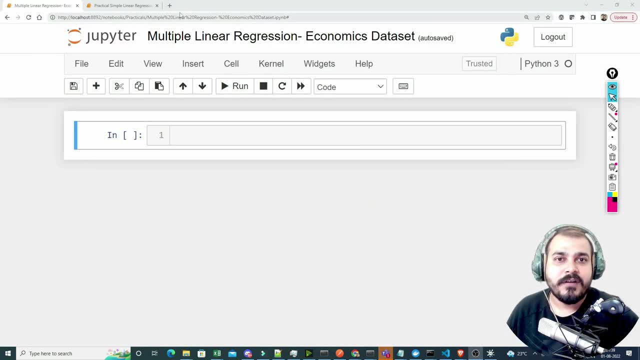 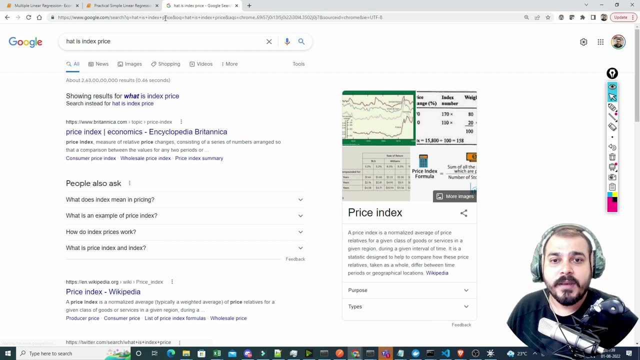 This data set is all about index price. Now, first of all, we'll try to understand what is index price. OK, so what is index price Now? here you'll be able to see. index price is a measure of relative price changes consisting of a series. 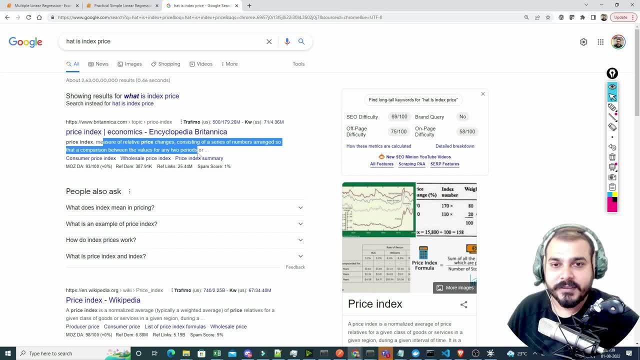 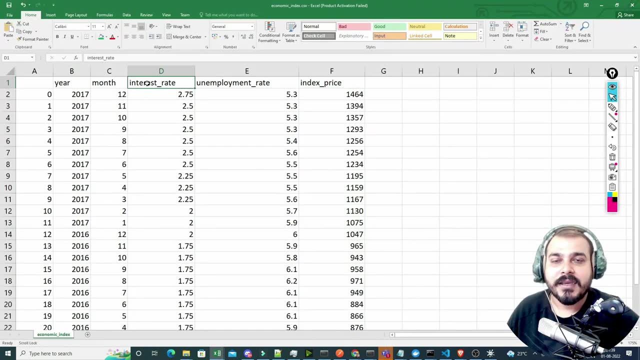 of number arranged so that the comparison within the value for any two periods. So to calculate this index price- and government uses this specific index price over here- we require two important things, That is, interest rate of the bank and the unemployment rate, And based on this, by applying some formula, we basically calculate the index price. 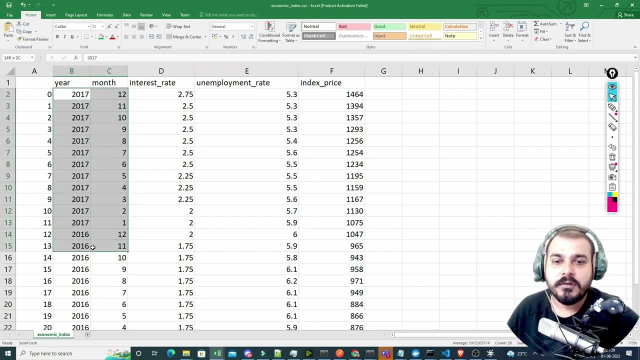 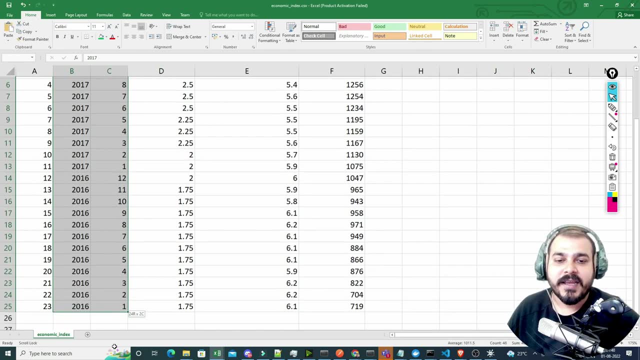 Now I have all these details based on month right, All 12 months, you can see two years data is there. That is the reason you can actually find out 24 records. So 12 years data is there. Now we need to create a model which will be taking these two important features. 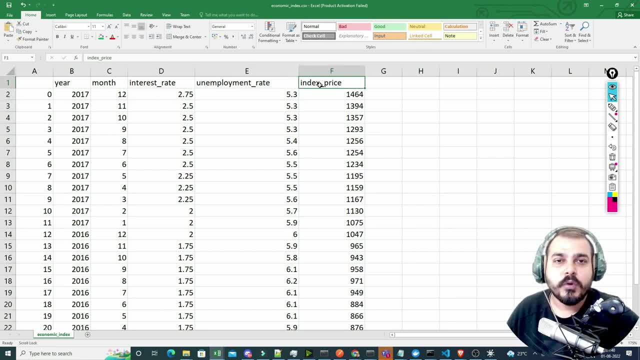 that is, interest rate and unemployment rate, and it should be able to give us the predicted output index underscore price. And that is what we are going to do. Why we say this has a multiple linear regression, Because here I specifically have two features. 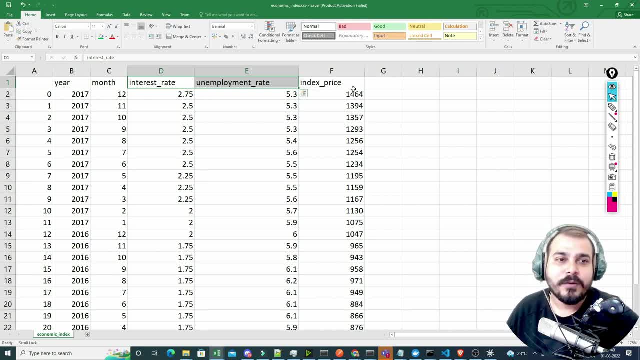 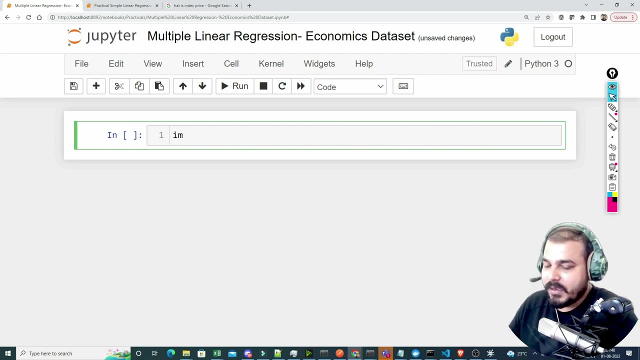 OK, in the previous example we just had one independent feature and one output feature, But here we have two independent features and one output feature. OK, so let's go ahead and let's try to solve this problem Now. first of all, as usual, what I'm actually going to do over here is that import pandas are speedy. 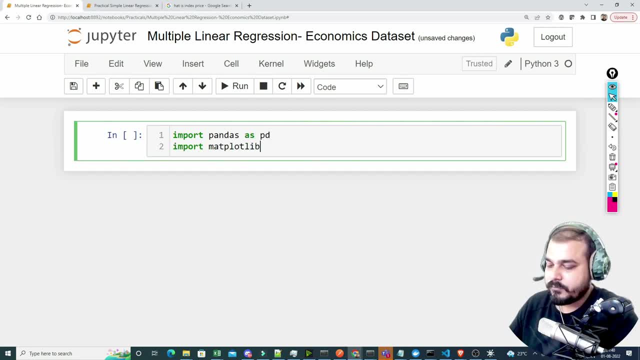 So same step: import matplotlibpyplot as plt, Then import numpy as np, because this, all things, has been already done. So I'm just going to quickly complete this, so that I hope everybody knows how to do this. Now we will try to read the data set. 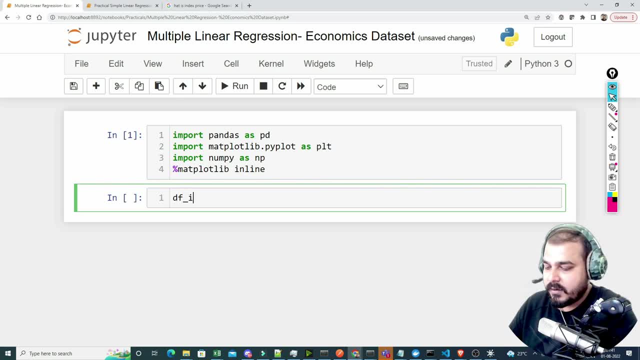 So here I'm just taking the specific data set and I'll say df underscore index. OK, And I'm just going to read This data set. let's say I'm going to write: read underscore csv. Read underscore csv. and here I'm basically going to take pd dot- read underscore csv. 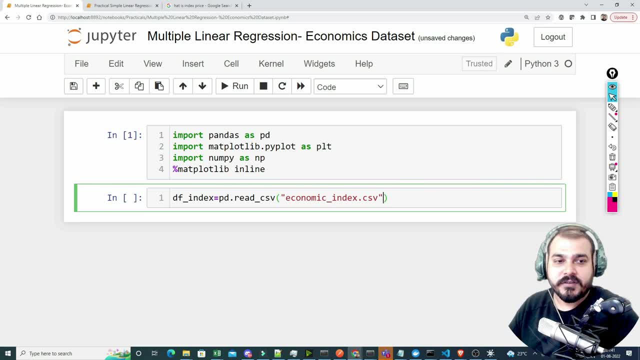 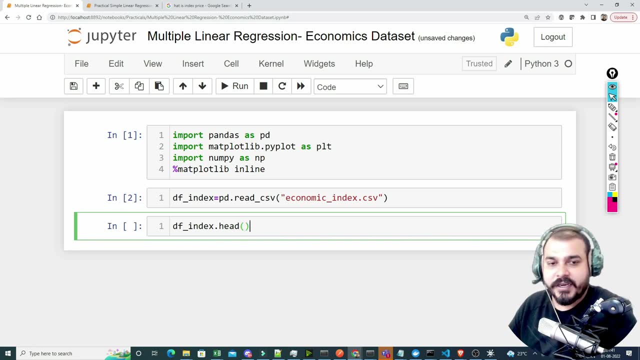 And here I'm going to basically take economic index dot csv. Right now, if I write df underscore, index dot head, So I basically have my two years data. Very simple Now over here, the first thing that you will be able to see, right. 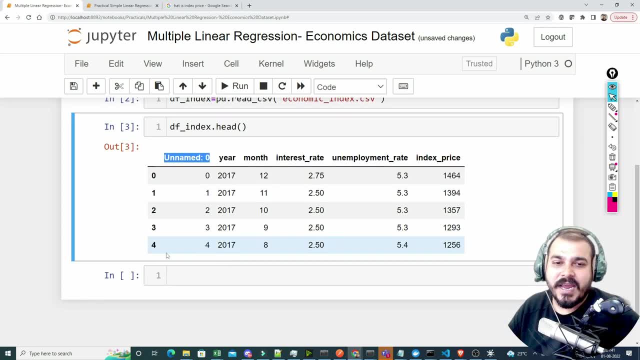 You have this extra column that is getting created, So first of all, I will just drop this column in order to drop this unnecessary column. Let's drop unnecessary column, And here unnecessary column basically means I can also consider year and month, because I don't require this right based on interest rate and employment rate. 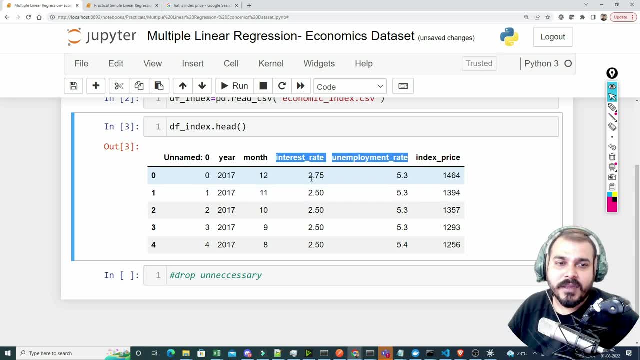 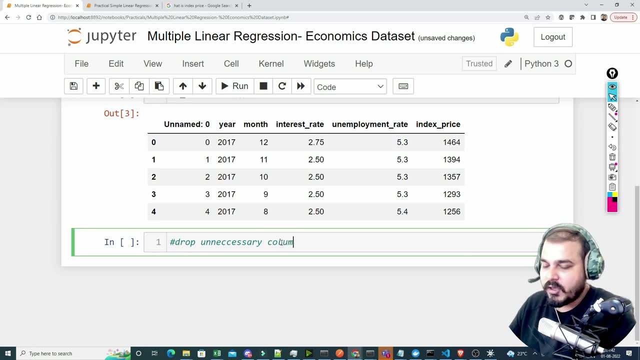 I need to be able to predict the index price, and whatever year or whatever month. if these values are given, we should be able to predict the index underscore price. OK, so let's drop unnecessary columns. So here, first of all, I'll use df dot drop. 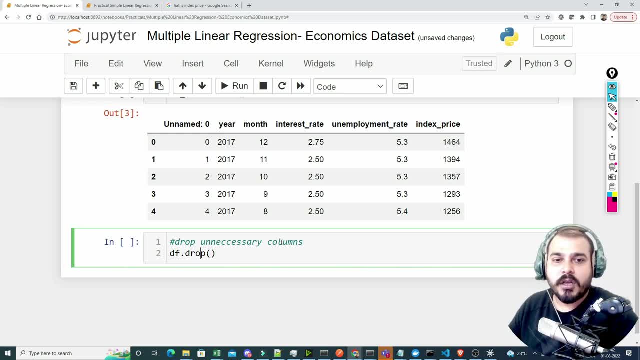 And always make sure that whenever you're trying to drop a column, you have to use one important parameter. OK, so let me just go ahead and write df, underscore, index, dot drop, And let me press shift tab Here. you just need to provide the labels and your access value. 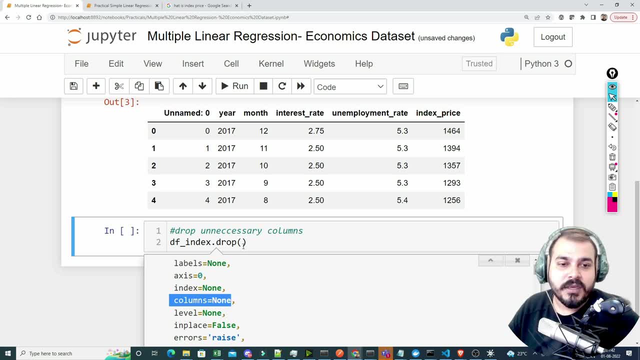 You can also provide index or columns. OK, so here first of all columns, So columns. here I can definitely provide something like, let's say, in the list It will be unnamed, Unnamed, or I'll just copy the same thing. 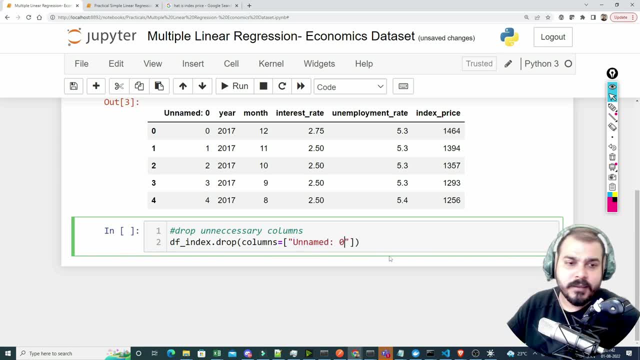 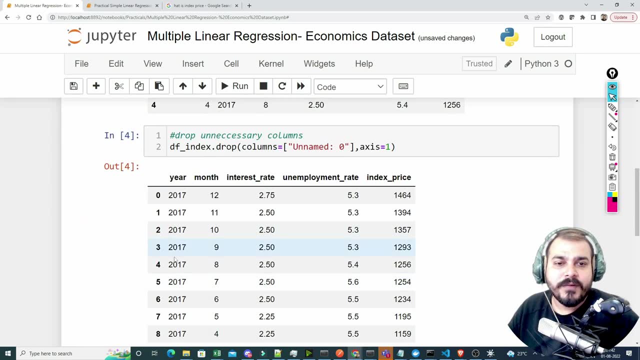 OK, And here I will add: access is equal to one. So if I execute this here, you can see that this unnamed column will get dropped Right And this will be the remaining data that I'll have, But I also have to drop year and month. 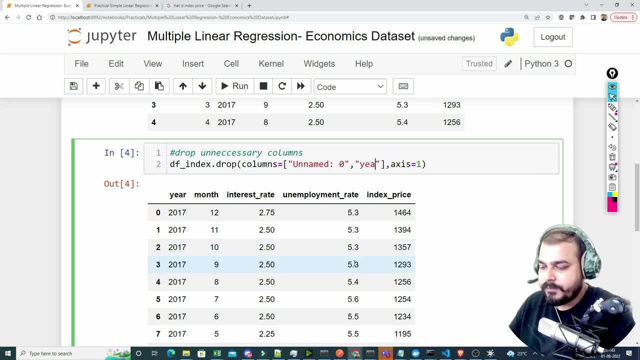 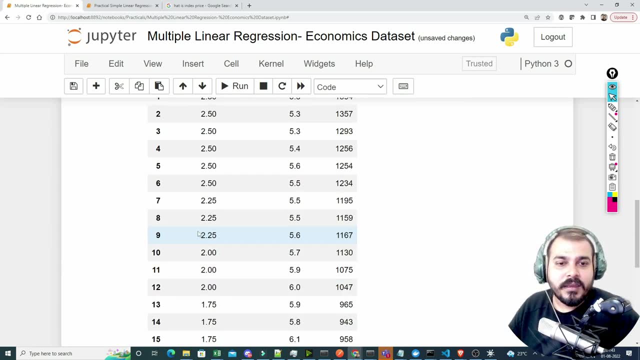 So what I'll do in this list, I will add here, And I will also add my month. So once I do this here, you'll be able to see that It is getting deleted. it's working perfectly fine now, when you're. 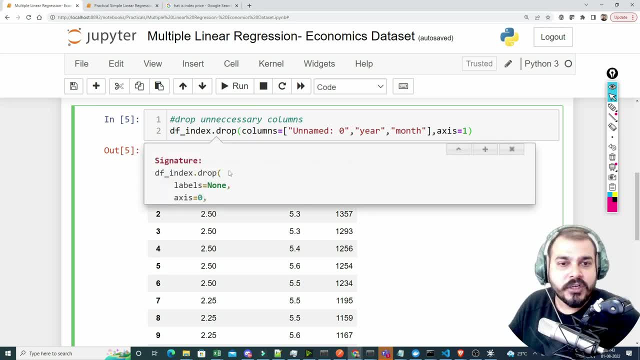 sure about this, then there'll be one more feature inside this, one more that will be in place is equal to right. here, when you do in place, In place is equal to true, That basically means you are actually dropping the column now, Right. 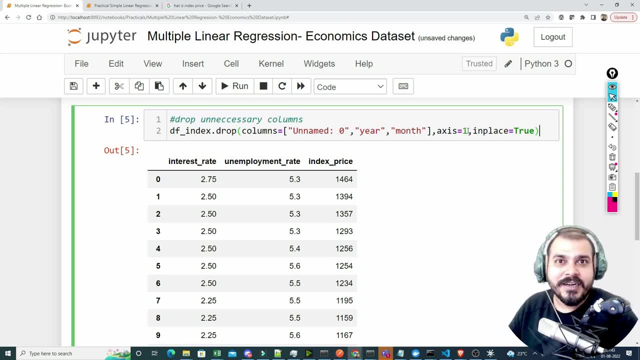 So, and once you drop the column, it will get updated in df underscore index. That is the main importance of in place underscore. true, That basically means, within this particular data set, you're dropping it and you're updating it. So now, if I go ahead and execute this, this will be my df underscore index, dot head. 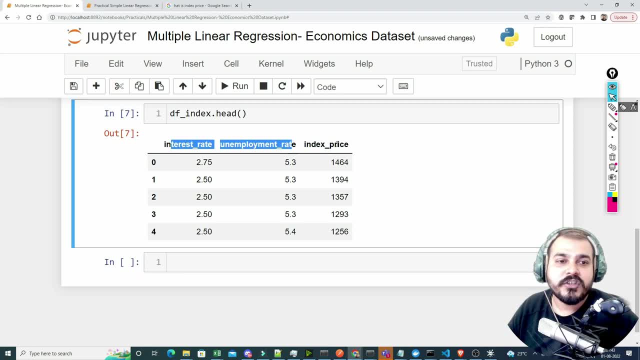 Now, here you can see, I have two features- independent features- and one dependent feature. Perfect. Now, first of all, let's go and see whether we have any null value. So in order to check the null value, I will write: df: dot is null, dot sum. 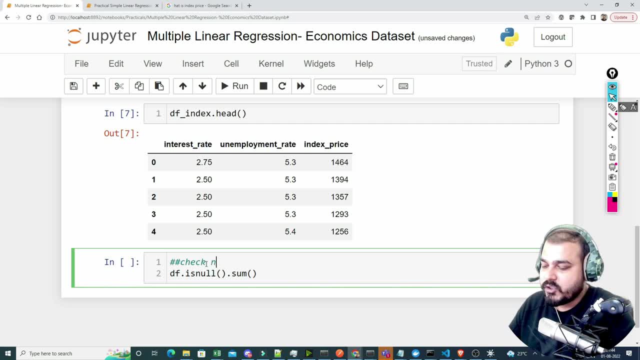 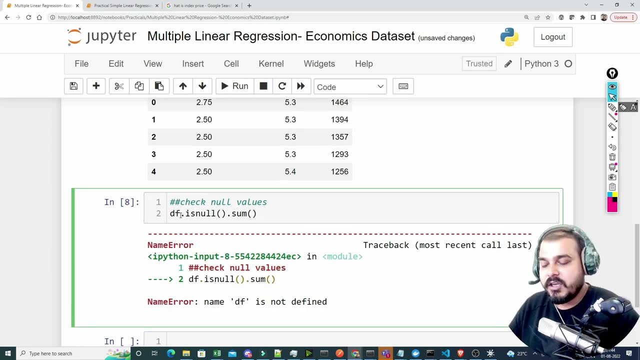 This is the common code to basically find out, Check null values. OK, And right now I'm not taking it, but as we go ahead we'll have some amazing problem statements. So let me go ahead and write it as df underscore index, because that is the habit, right. 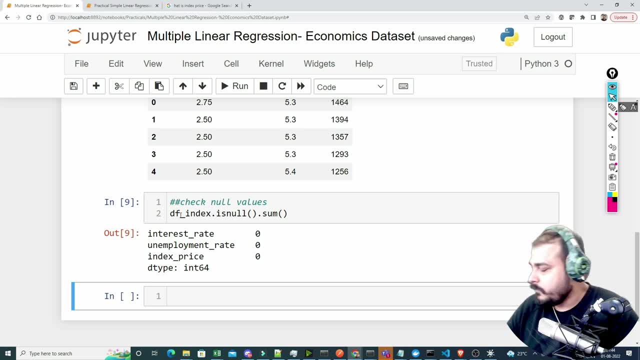 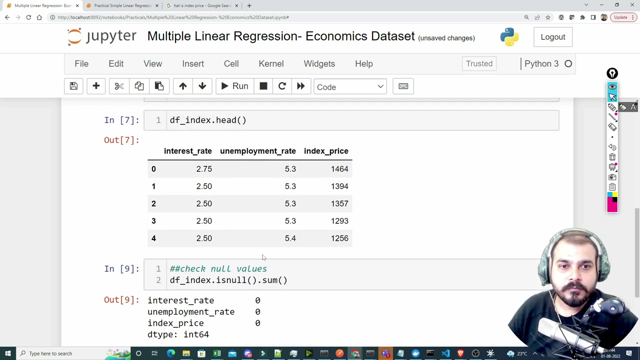 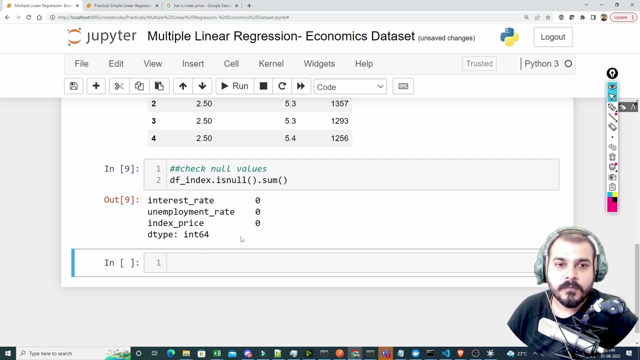 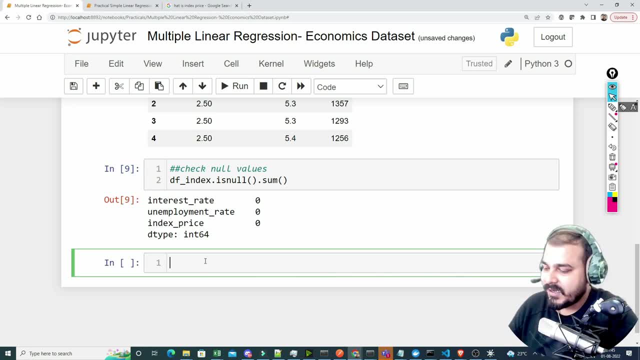 So, obviously, this particular dataset, what I'm actually first going to do is that let's do some visualization. OK, And this visualization that I specifically do: I use a library which is called as import seaborn, As SNS, and then here I'm just going to write SNS dot. 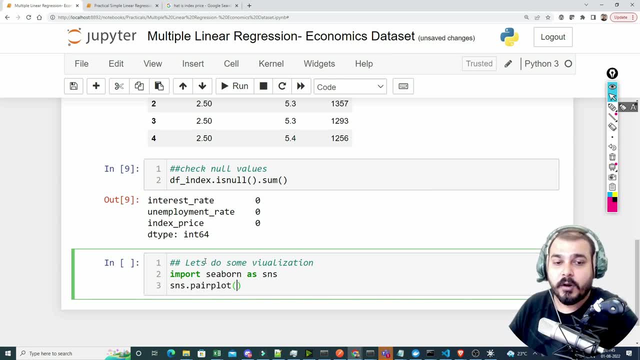 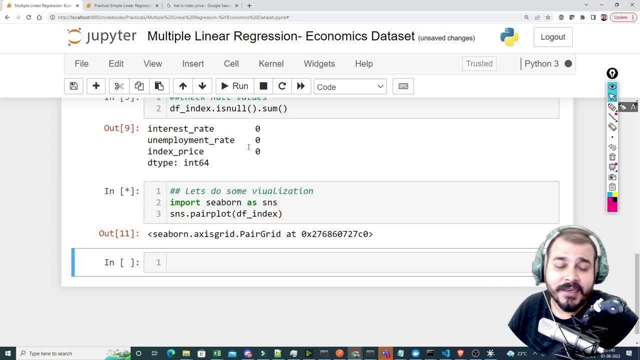 for that specific library function that I'm going to use is something called a spare plot, and if I give my df value here automatically- sorry, it should be df underscore index again. I'm making this mistake again and again, Not a problem. 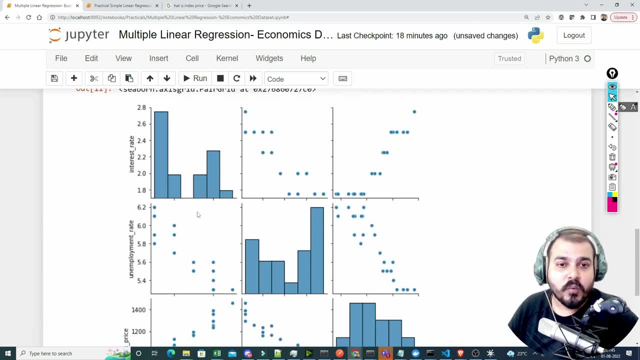 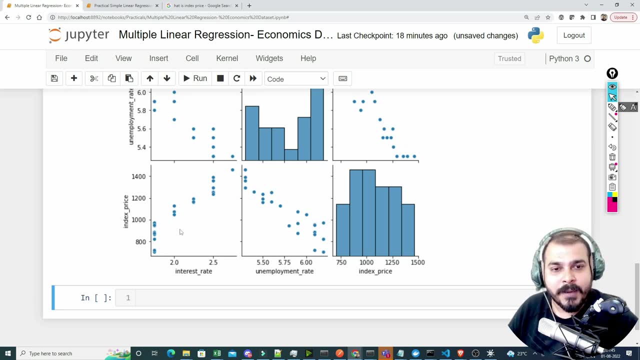 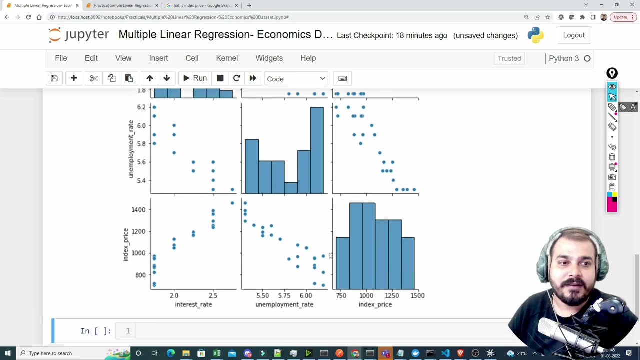 Now, if I probably go and see this df underscore index, here is what things you are actually getting. You can basically see with respect to index price and interest rate. you can see some some linear relationship is there with respect to index rate. you can see inverse relationship. is there right? 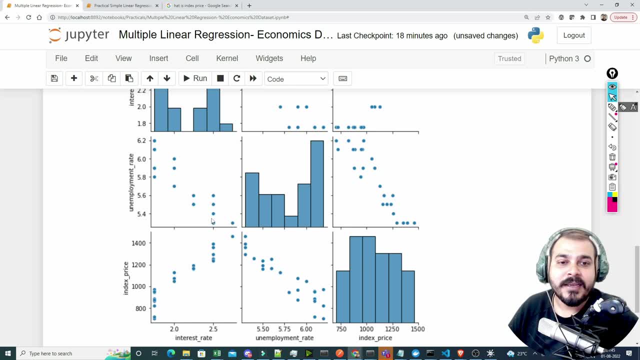 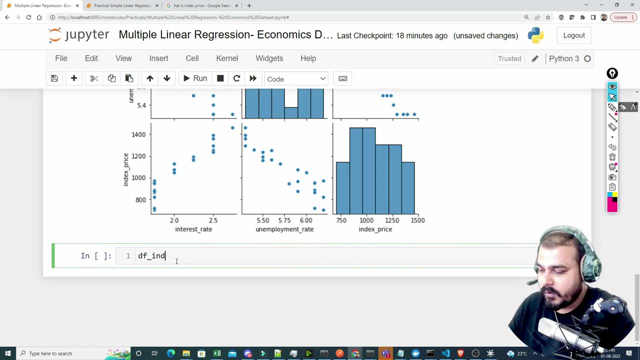 So again, if you check employment rate and interest rate, again here you are getting an inverse relationship. So if I probably go ahead and write df, dot, df, underscore, index, dot, CORR. So here what we are going to get is that we're going to get some negative values. 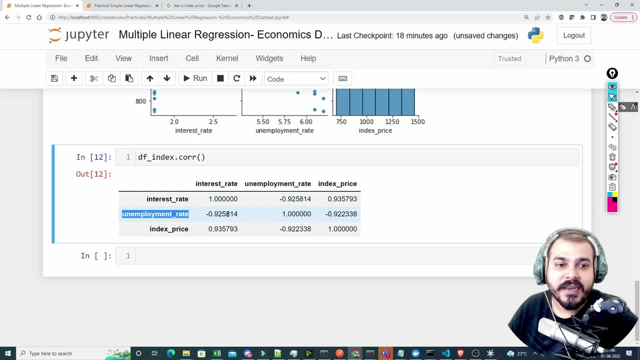 also because this interest rate and employment rate: here you're having a negative correlation. Similarly, with respect to this index price and unemployment rate, here you are having a negative correlation. But if I see, with respect to interest rate and index price, you have a positive correlation. 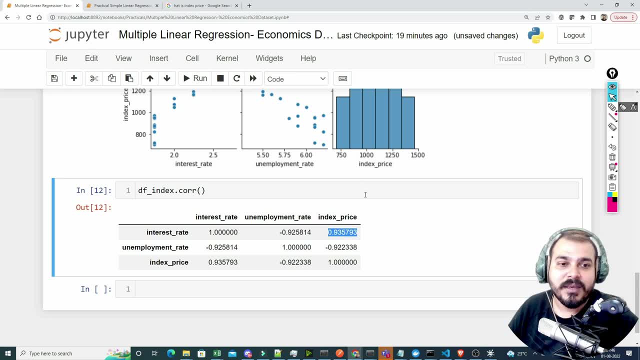 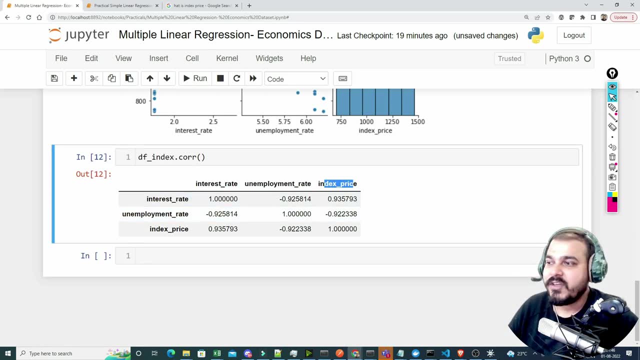 So that basically means, as the interest rate is increasing, your index price will keep on increasing. If your unemployment rate is increasing, your index price will be decreasing. Now we are going to use this two specific feature and try to implement some amazing you know. 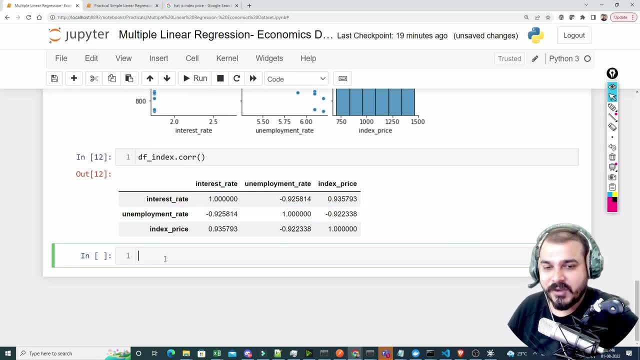 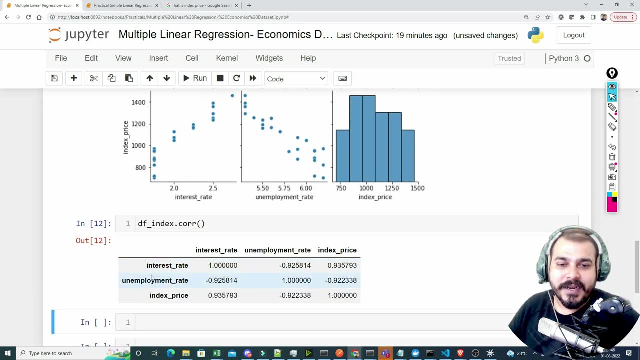 will basically create a machine learning algorithm using multiple linear regression. OK, now let's go ahead, and let me first of all make some cells. I'd also like to make sure that I visualize this data points right- unemployment rate, interest rate- properly. 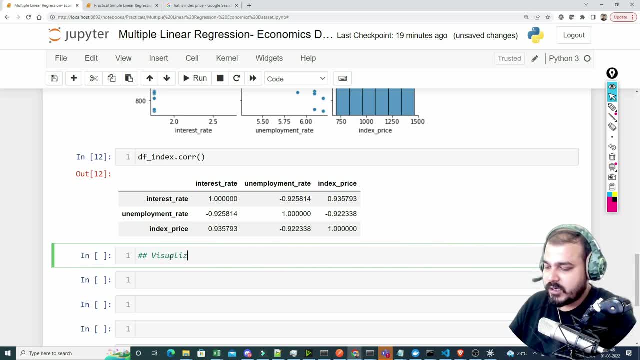 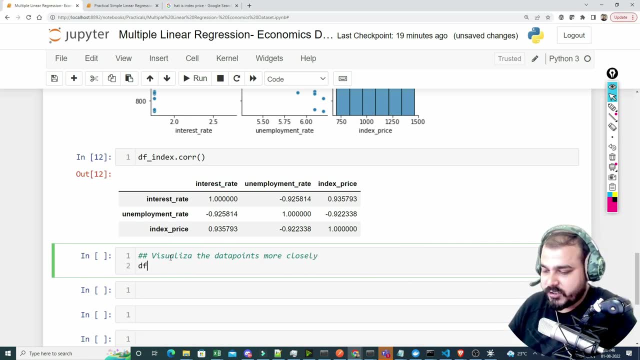 Right. So let's go ahead and visualize this more closely, visualize the data points more closely. OK, so here I'm going to just take df, underscore index. Or I can also use PLT, dot scatter plot, And here I will be using df of. let's say I will go from. 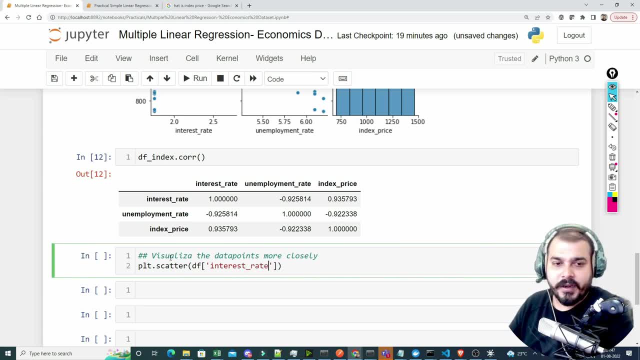 interest rate, Interest underscore rate along with. I really also want to see the correlationship between. OK here one more thing that we saw right: What is the correlation between unemployment and interest rates? So obviously, here you can see that it is an inverse one. and with respect to index price also, it is an inverse one. 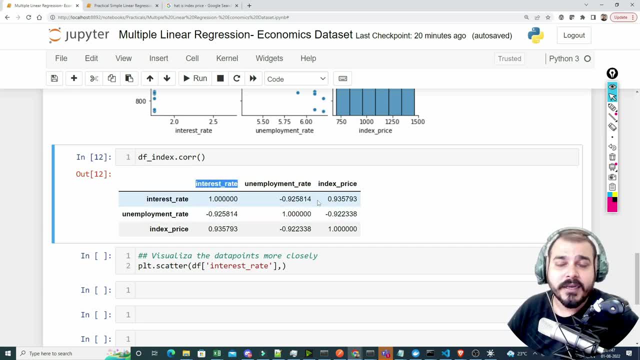 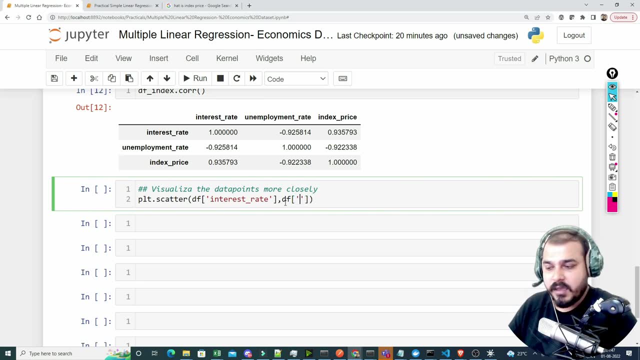 So obviously both these features will play an important role in predicting the output. OK, so now, if I go ahead and probably see the scattered plot, df of interest rate and df of unemployment rate- OK, so let's say unemployment underscore rate. OK, and here I will probably use a color. 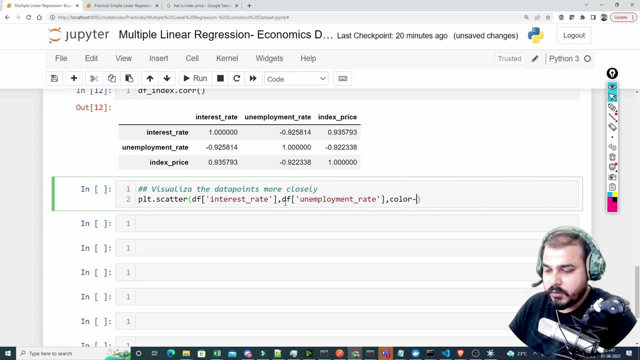 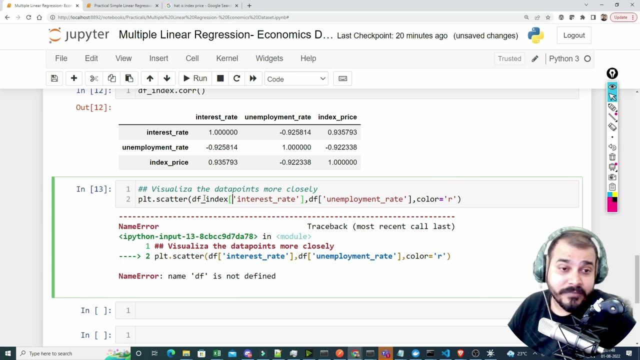 Let's say COLOR is equal to red points. OK, so here it will be R Now, if I probably execute it. so here you can see df underscore Index- again same mistake, but I don't want to edit this part now. 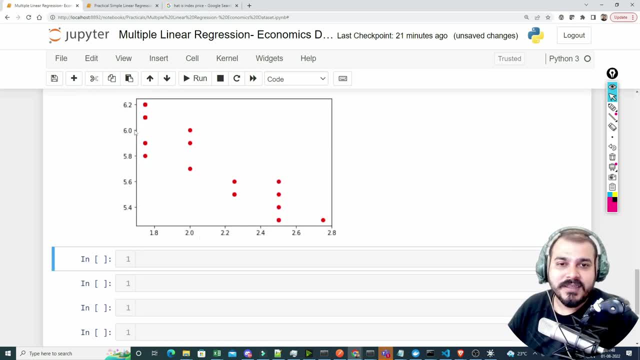 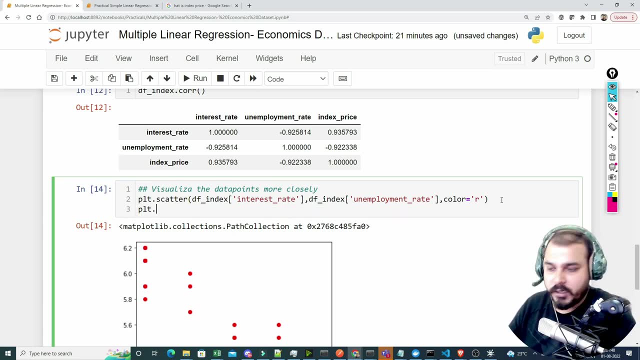 because it can happen with you. OK, So here obviously you can see that it is having an inverse relationship. OK, so obviously here I can also do PLT dot X label, And here I'm just going to write it as interest rate. 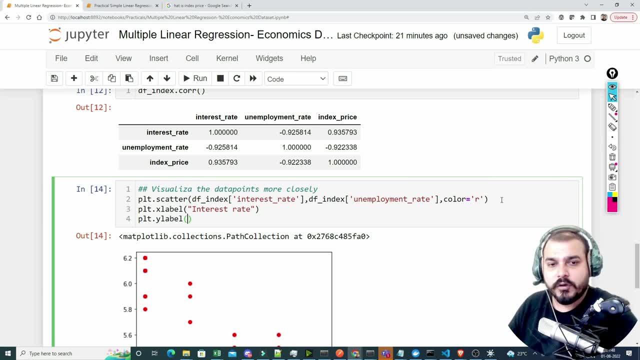 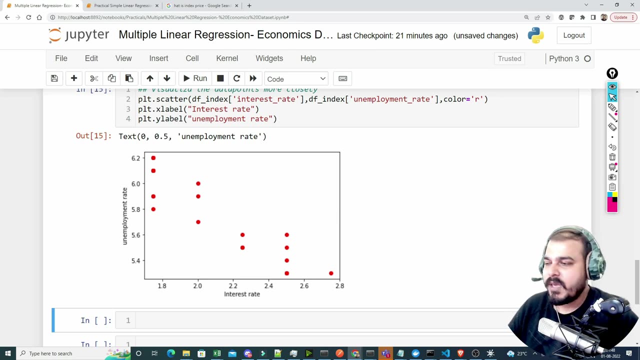 PLT dot Y label. Here I'm going to basically have Unemployment rate OK, and once I execute it here, you'll be able to see it Obviously. inverse relationship: the same diagram, we have got it in a bigger one. 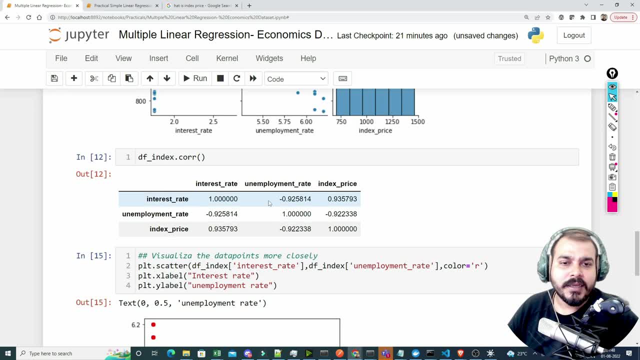 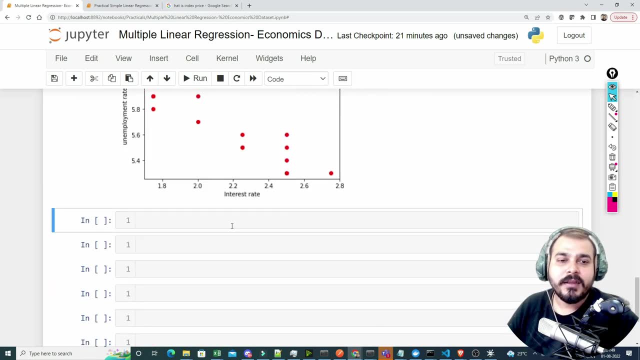 OK, now Do it for the next one, that is, interest rate and index price. Obviously, you'll get a positive correlation. This is perfectly fine. Now let's go ahead and implement. First of all, what I'm going to do is that get my independent. 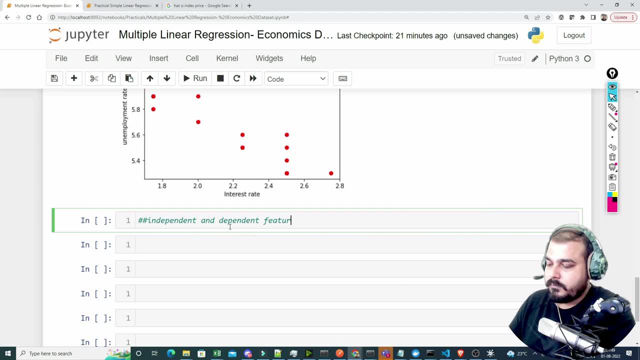 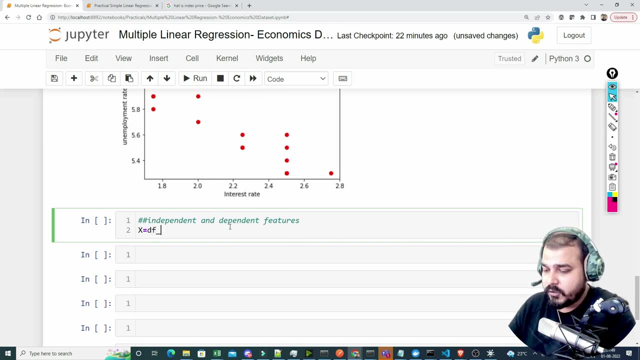 And dependent feature Right And when I get my independent and dependent features. first of all, I'll write: X is equal to DF underscore index. I know what all column I basically want, So I'm just going to write my column name. 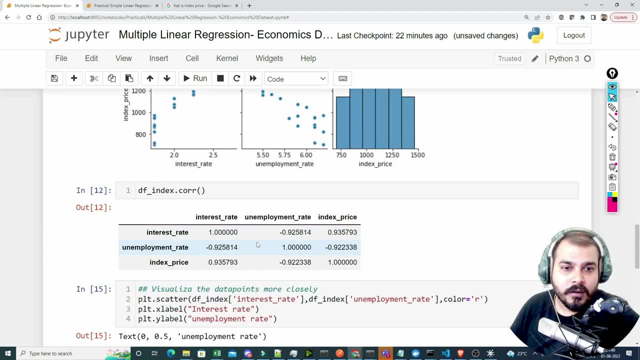 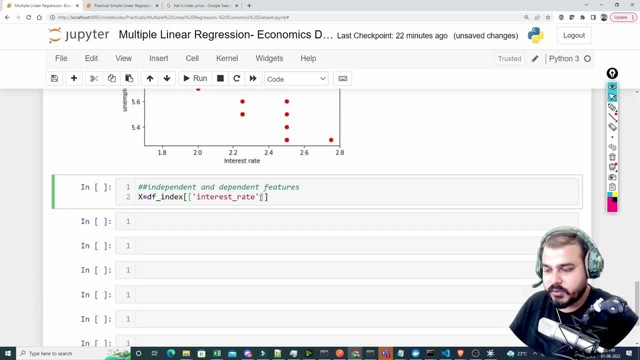 So first one is interest rate. Let's see, This will be my interest rate And this, the next column, will basically be my Unemployment rate. OK, I can also do in this particular way. Let me show you and another way. how do you, how you can basically do it. 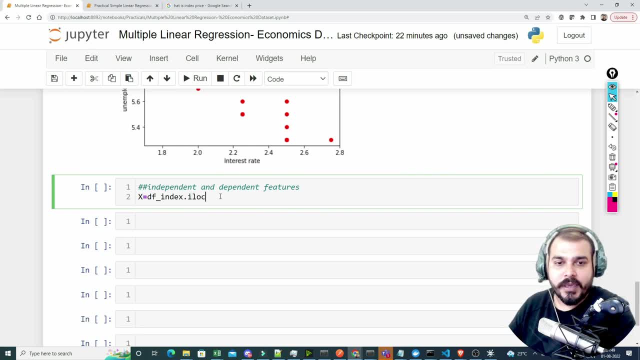 OK, so DF underscore index. I can also use ILOC. OK, and here ILOC first parameter says: take all the rows from all the rows, just remove the minus last row, And here you'll be able to get your X value. 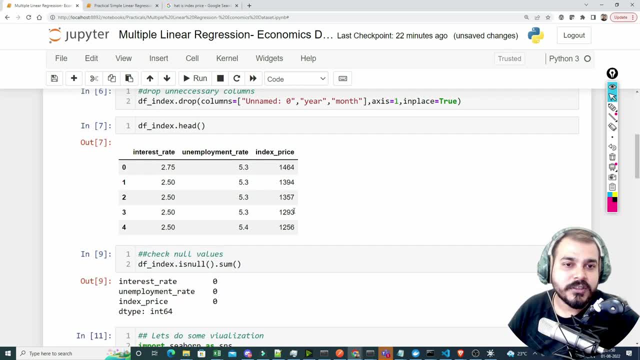 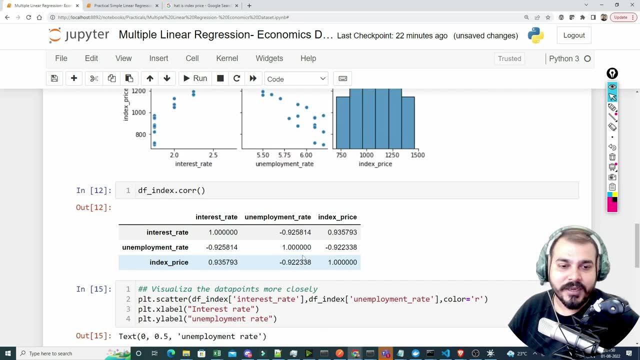 That basically means from all the features, just from all these features that you have. just remove the last feature, because index underscore price is your output feature and this is obviously a continuous value. So regression problem we are trying to solve OK. similarly for the Y variable. here you can write DF. 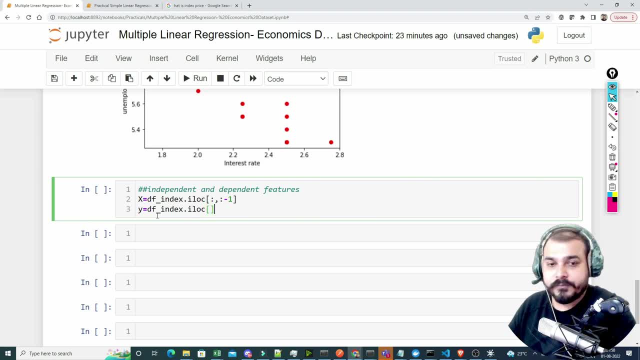 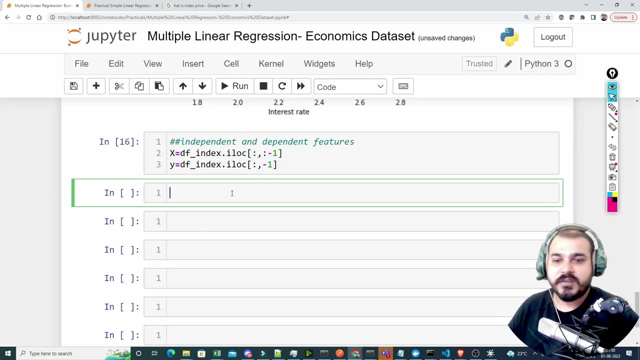 DF, underscore, index, dot, ILOC, and here colon, comma, colon Or minus one. I'm just saying that take the last column and put it in the Y value. OK, so this two way also you can basically do it. OK, so once I execute it here, you'll be able to see X. 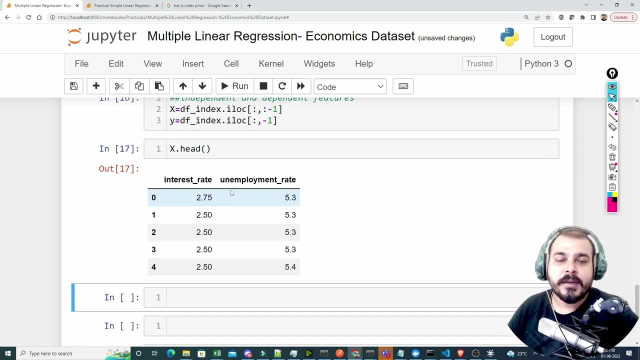 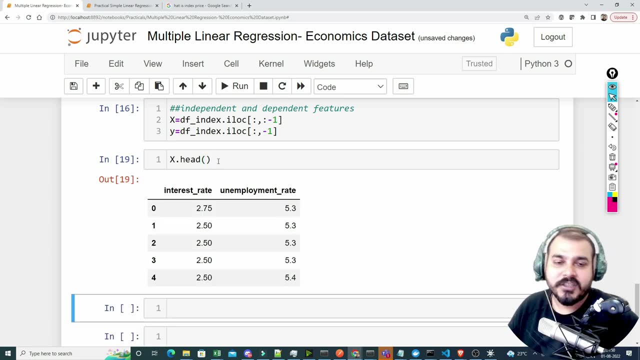 So let's go and see X dot head. Here you see your interest rate and unemployment rate. And similarly, if you probably go and see Y, here you'll be also able to see. Anyhow this will give you a tuple, So I'll not suggest you to go and display your data like that. 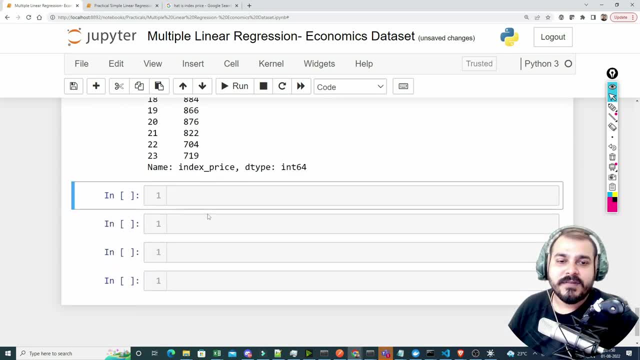 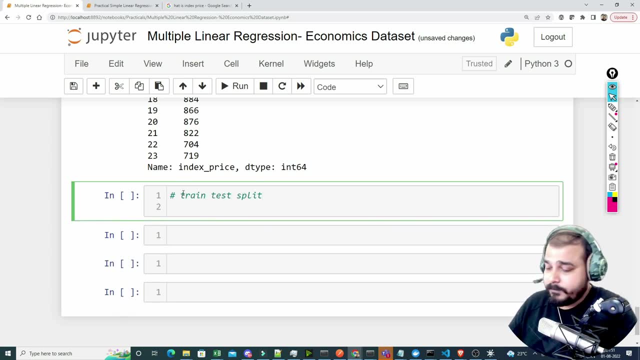 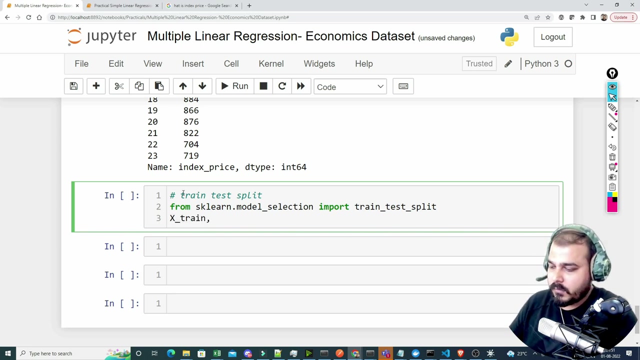 Here is perfect. Now the next step is very simple. We will do the train test split, as already explained. Train test split OK from a scale on dot model selection. I'm just going to import Train test split, OK, and then you have X train comma. 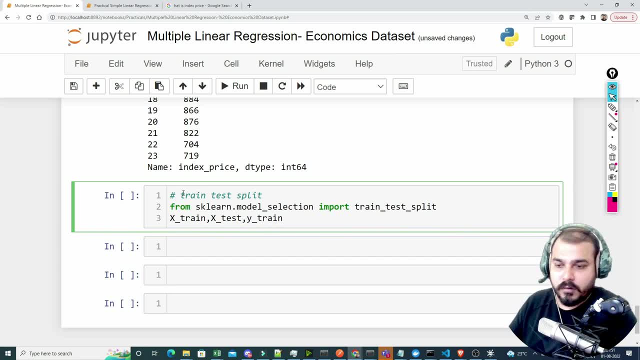 X test comma Y: train comma Y: underscore test. OK, And then here I'm just going to use my train test split. I'm just getting bored a little bit, So let me go ahead and copy some of the code from here. 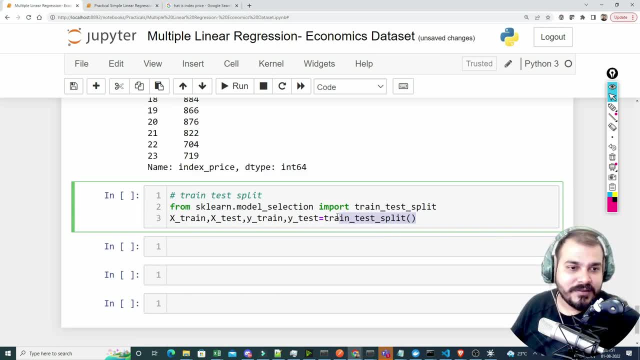 So this is my train test split. Let's say I'm doing 25 percent, So I'm just going to paste it over here. OK, So here I've given X, Y, Test size 0.25 and random state underscore 42.. 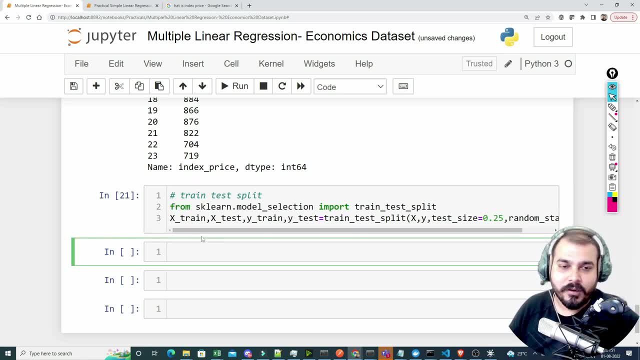 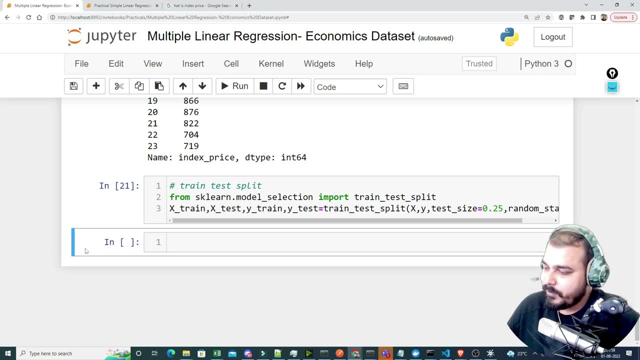 So once I execute it here, you will be able to see your X train, Y train, and all right. Now, guys, I'm also going to introduce you all to a new kind of plot in Seaborn, which will basically be very 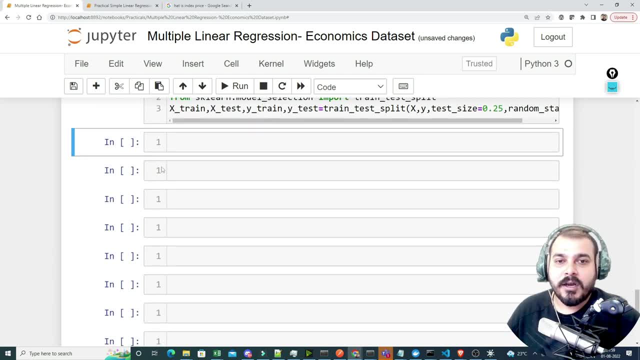 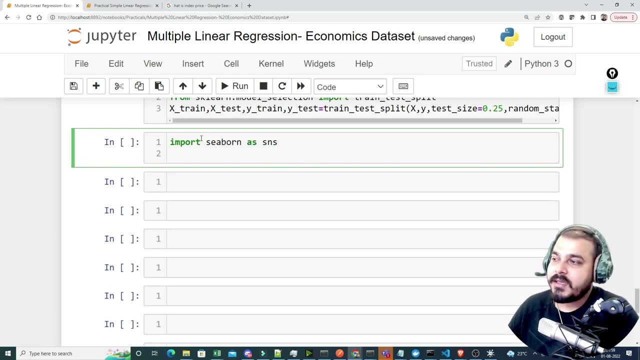 very helpful when you are actually working with this kind of data. Now let me go ahead and show it to you. First of all, let me import Seaborn as SNS. Now in Seaborn, you have something called as REG plot. 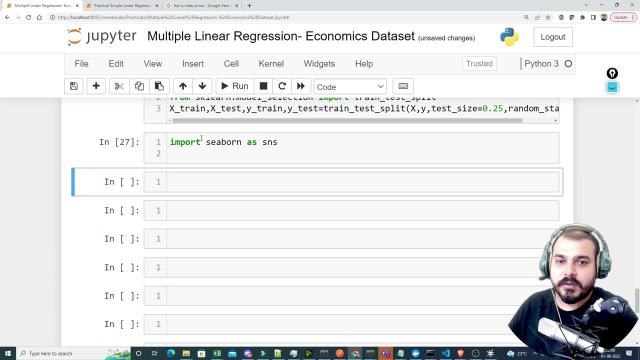 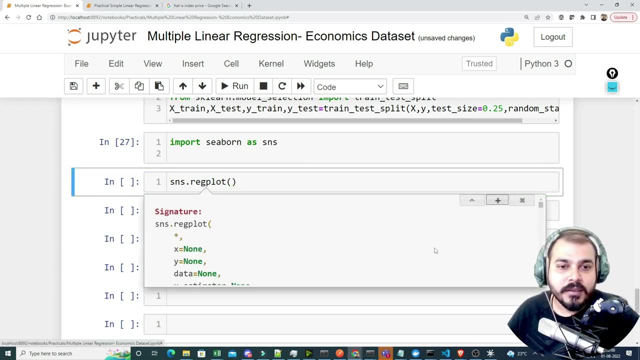 OK, and if you probably want to see this plot, I'll just execute this. OK, and let me copy this one over here. and let me just write shift tab Now here in this particular plot. this plot is all about this plot. 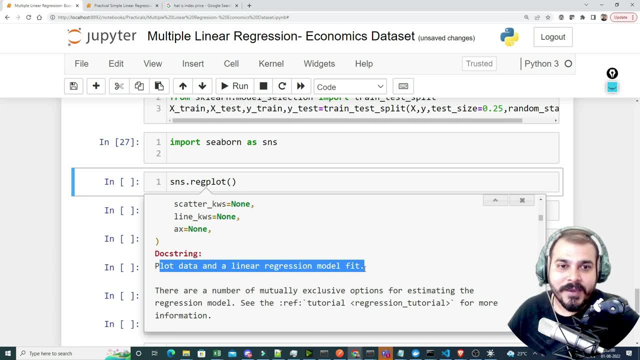 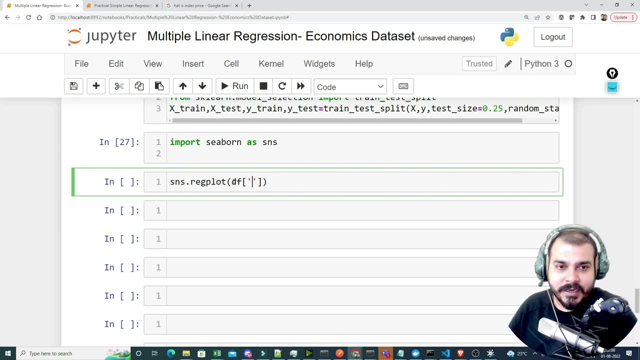 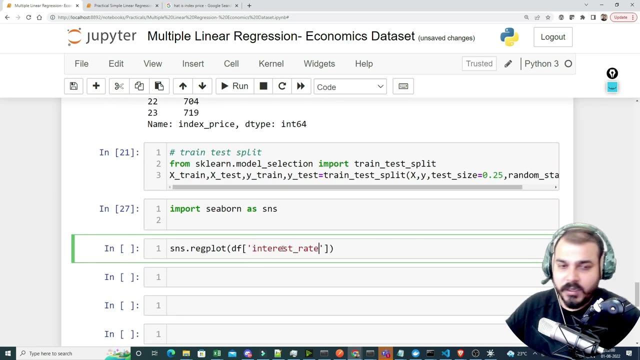 It plots data and a linear regression model fit OK. so let's say, if I'm using DF of DF of, let's say, in my X axis, I'm just going to put one of the features which is like interest rate, And my another feature over here will be DF of the index price. 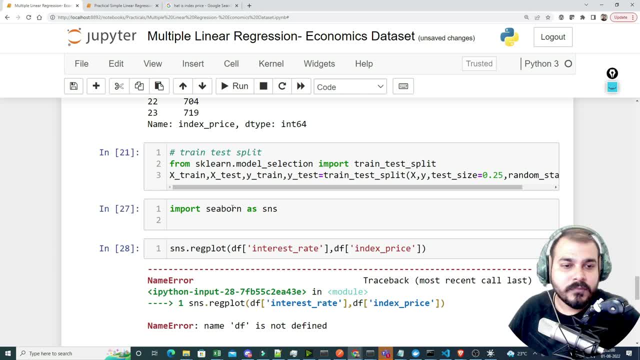 OK. so if I just try to plot this, OK, so it should be DF underscore index. OK, my mistake again, not a problem, You should do mistakes. OK, DF underscore index. So once you plot this here, you'll be able to see with respect. 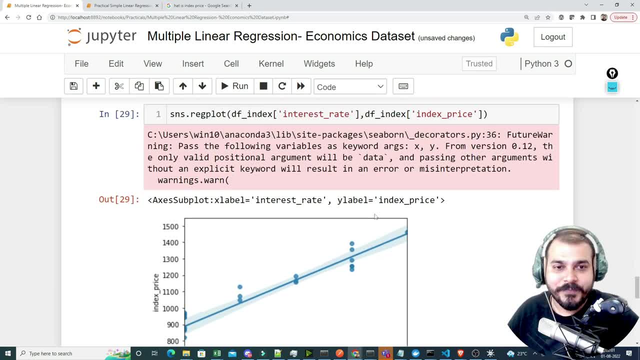 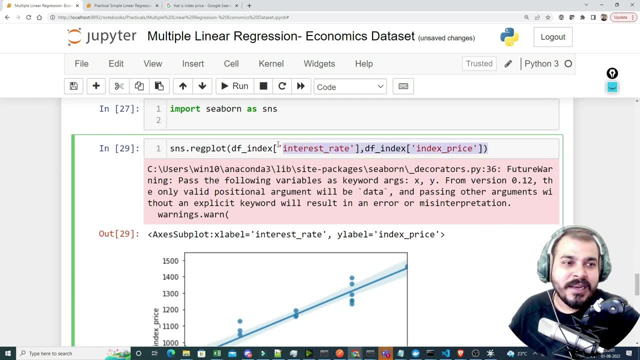 to this kind of data points. this is the regression line that will get created. So this gives you an amazing idea that, yes, the errors that probably are going to get is quite less OK. similarly, let's say that I'm going to copy the same thing and I'm just going 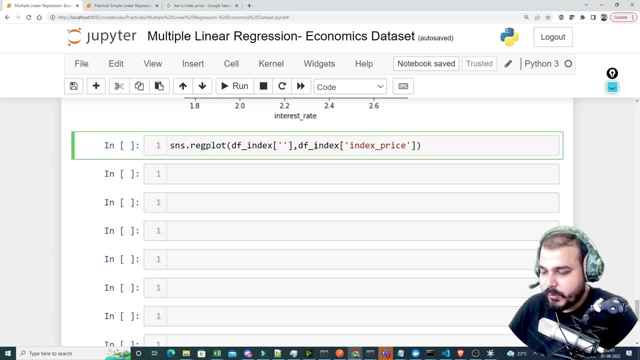 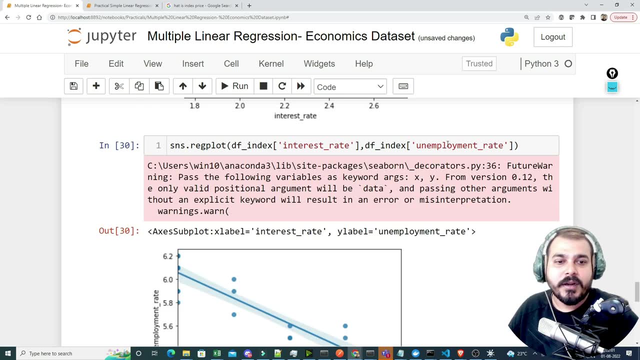 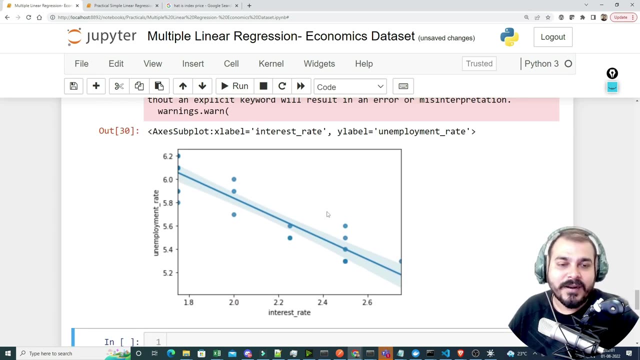 to plot this along with the interest rate, let's say the interest rate and the unemployment rate. So if I probably write unemployment rate and if I plot it here also, you'll be able to see that you are able to get an amazing regression line within this particular point. 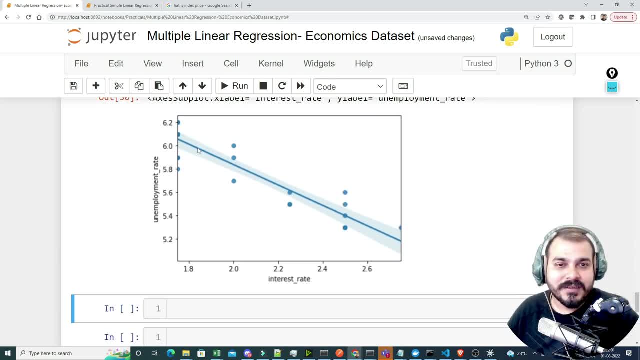 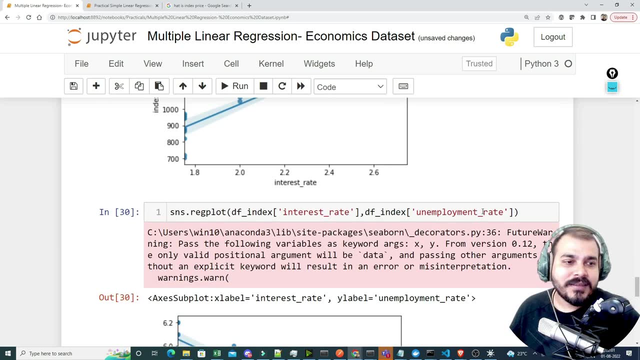 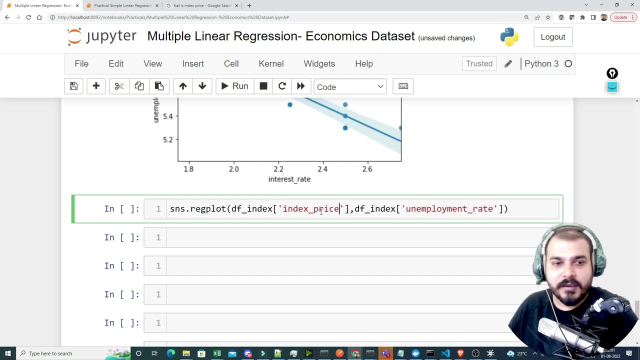 OK, And this way, and this, this shaded region, basically shows that, yes, we can hyperparameter tune this particular line to some level. OK, so, and similarly, if I probably try to plot this with index underscore price, here also you'll be seeing an inverse. 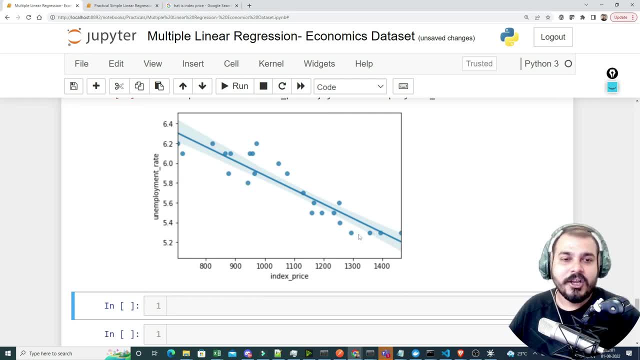 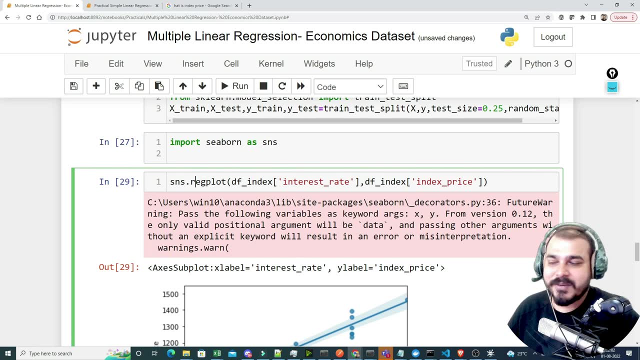 manner and with respect to that, here also you'll be able to see this kind of line. OK, so this was just an idea to give you every video and try to teach you something new, So I wanted to include this regression plot also. 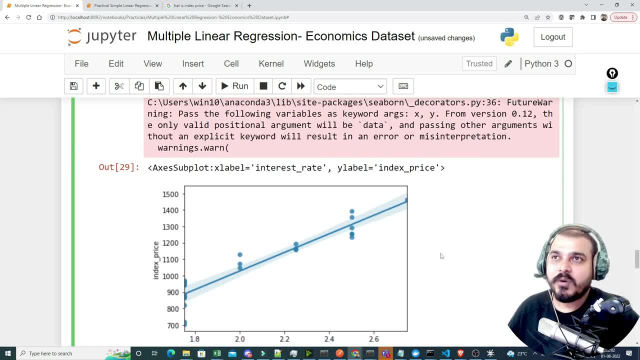 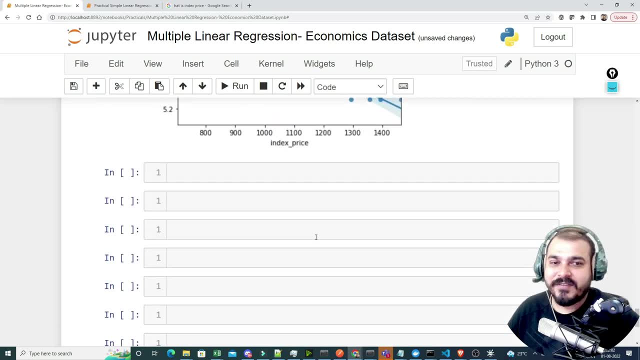 which will actually give you an idea. But again, you cannot do this for more than two features. You cannot basically create a 3D plot. It asks for only two features over X and Y. So with respect to that, you can definitely check it out. 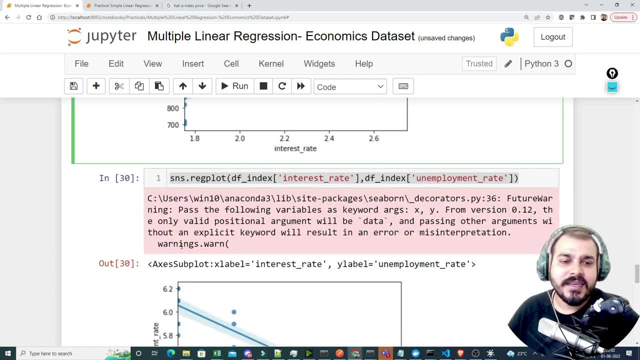 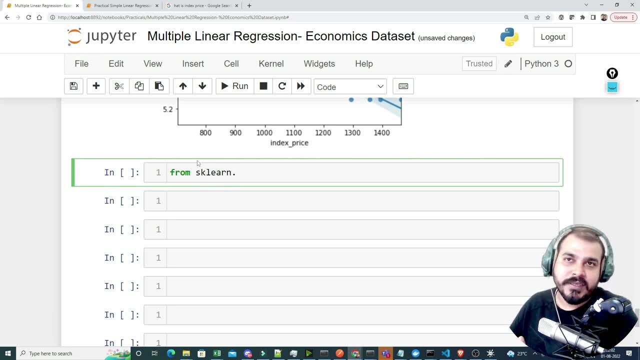 OK, now, since we have done our train test split, the next thing that we are going to do is that, obviously, standard scaling right. So I'm going to write from sklearn dot Now, see, I am not remembering where the standard scalar fall. 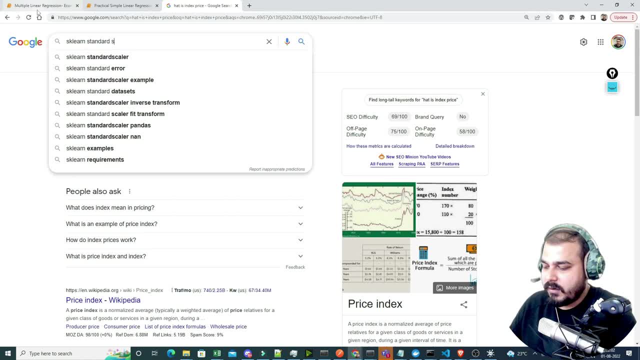 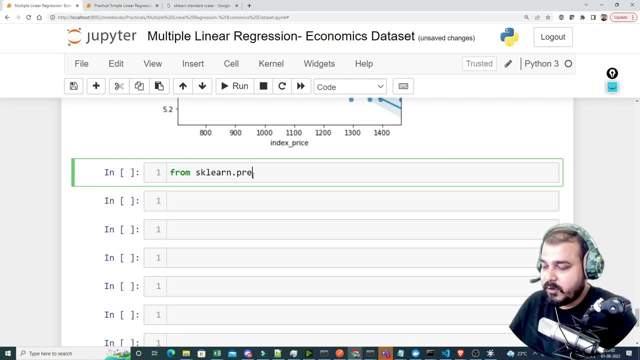 So I can go and search for it. sklearn, standard scalar- I'm actually not remember everything, guys, So it is present in processing. OK, right from sklearn dot preprocessing I'm going to import Standard scalar. OK, standard scalar. 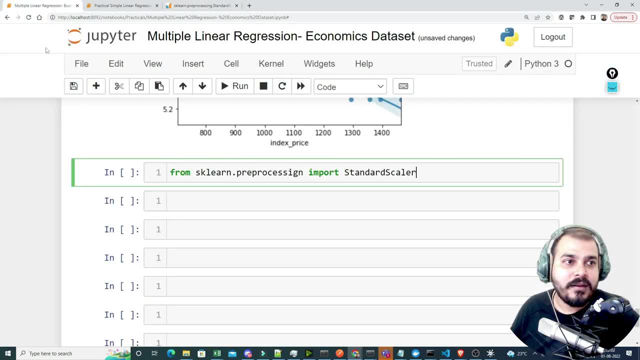 I think that is only the spelling. OK, standard, scalar. OK, perfect. So let me just go and import processing. This usually happens when you are doing the coding, because I'm not seeing any materials as such right now, because whatever comes in my mind, I'm basically. 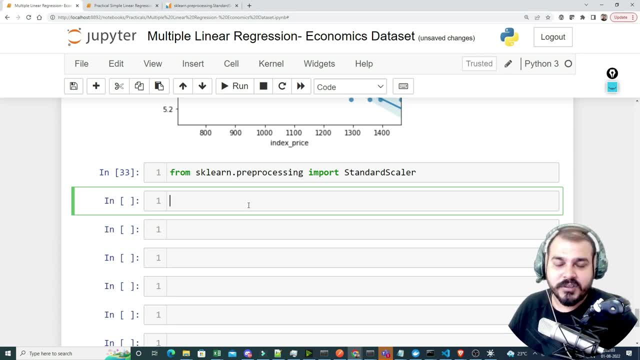 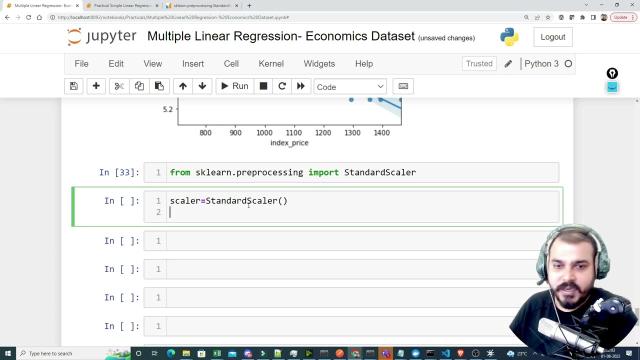 following the best methodologies as a developer, you know, So this will also help me to learn things better. So now what I'm actually going to do over here is that I'm going to create a scalar and I'm going to basically say standard scalar, standard scalar, and I'm going to initialize it. 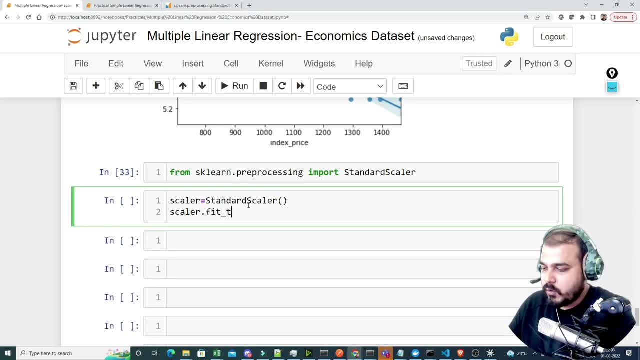 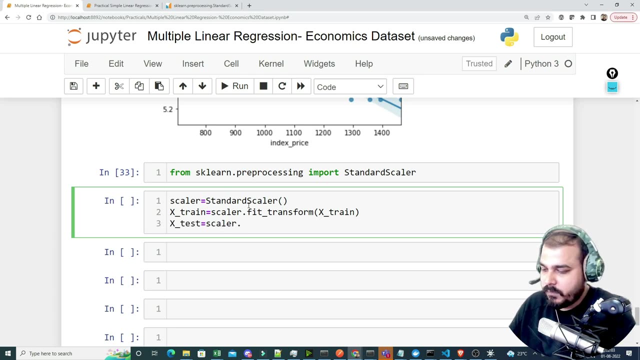 OK, then what we do? we write scalar dot fit underscore transform on my X underscore train data. Similarly, this will go in my X underscore train data And similarly, here you'll be able to see: X underscore test is equal to scalar dot. 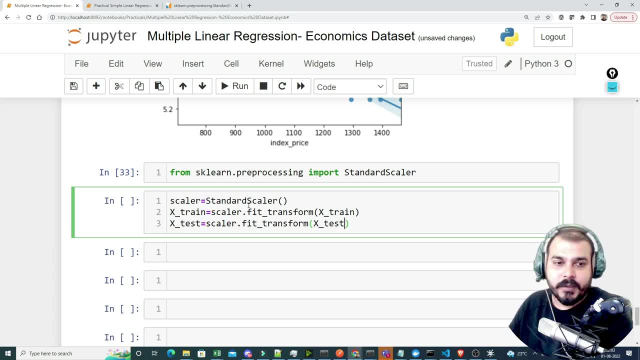 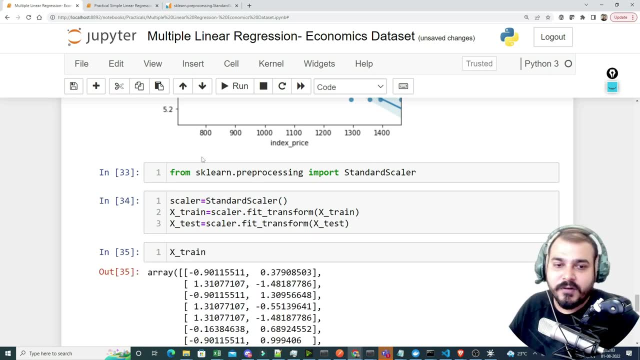 fit underscore transform on our X test data. OK, so this is my X train and X test. Perfect, We have got our X train. now. Let's see, We don't have to do it for the Y value. Now. see, here you have got two values right. 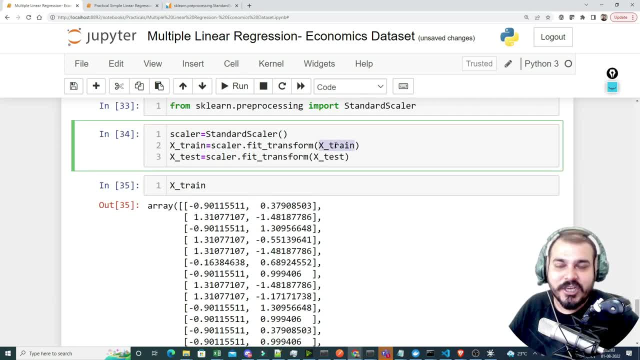 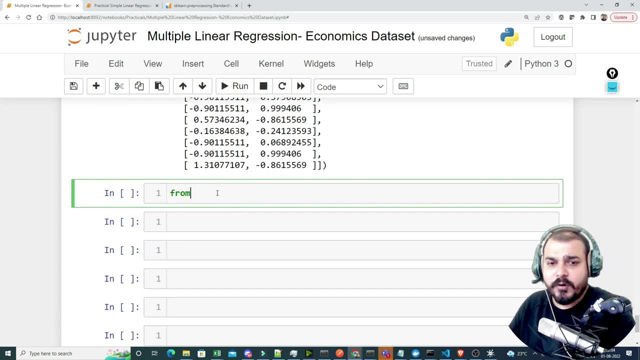 And when we do fit underscore transform, it converts this into a two dimensional array. So initially I had a data frame. It gets converted into a two dimensional, So this becomes. That's my input right now. The next step, what I'm actually going to do. 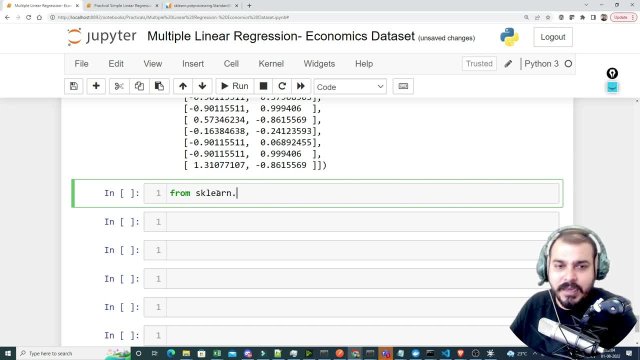 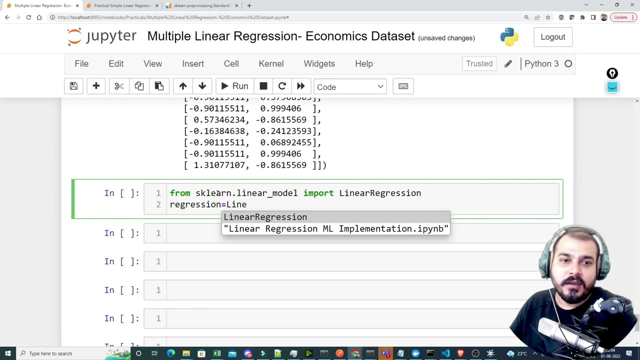 I'm just going to write from a scalar dot all linear model. OK, I'm going to import something called as linear Linear regression, OK, and this will basically be my regression, where I'm specifically writing linear regression. and this I've got executed. OK, then what I'm actually going to do: regression dot fit. 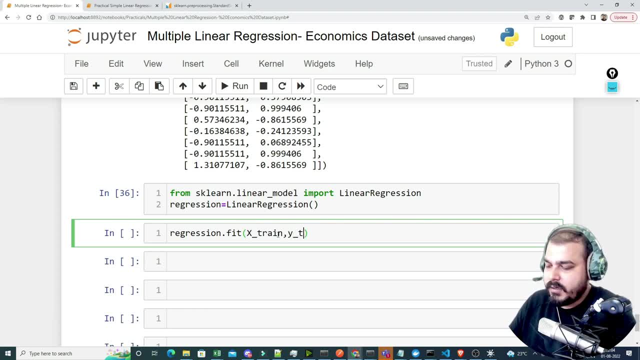 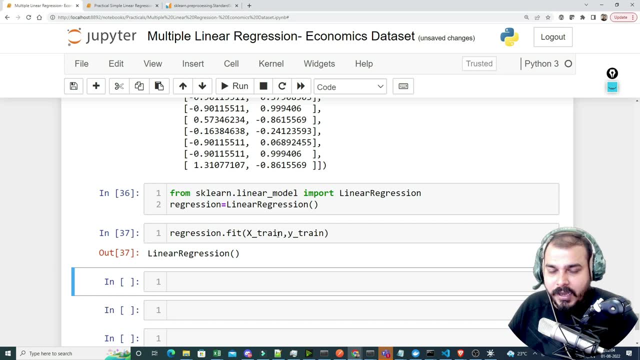 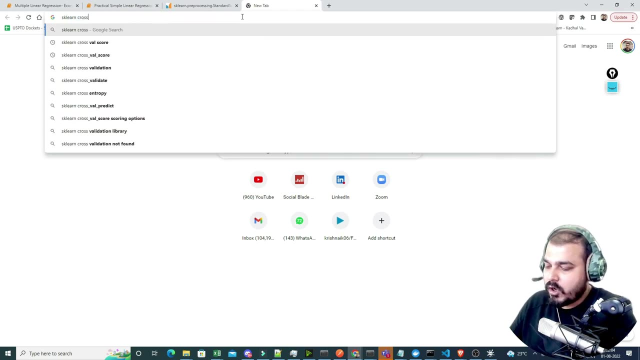 on my X train comma Y train data. OK, this is done. Now let me introduce you to something called a cross valve score also. OK, now this cross valve score will also give you some good results. OK, so let me just search for a scalar cross valve score. 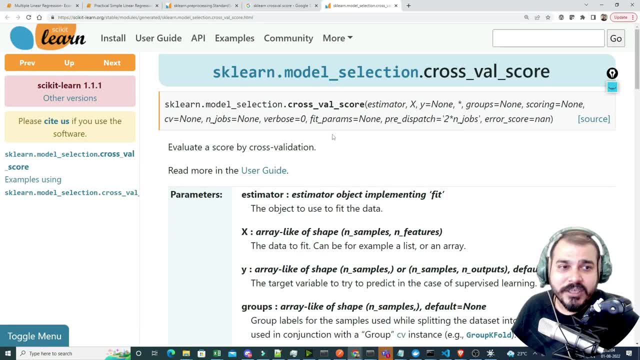 OK, now, as I said every video, I will try to teach you something new. OK, now, cross valve score is basically a cross validation method. OK, And then this is where I really want to talk about cross validation, And here all you have to do is that: give your model, give your X train, Y train. 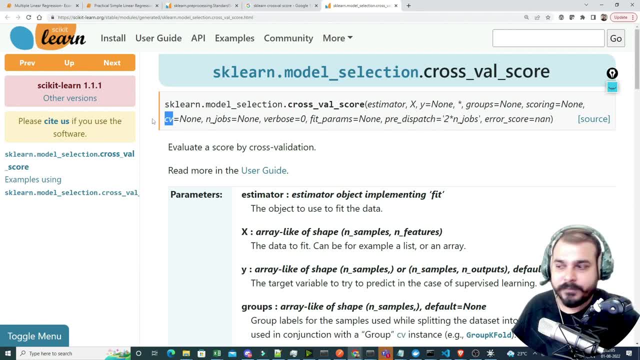 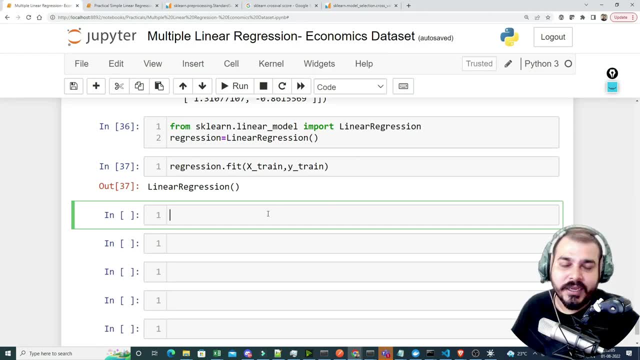 And this in turn will basically create a cross validation. Now, what does this basically mean? Let's say I'm going to write over here. OK, this is my regression. right, It has fitted to the X train and Y train. Let's say I import cross validation. 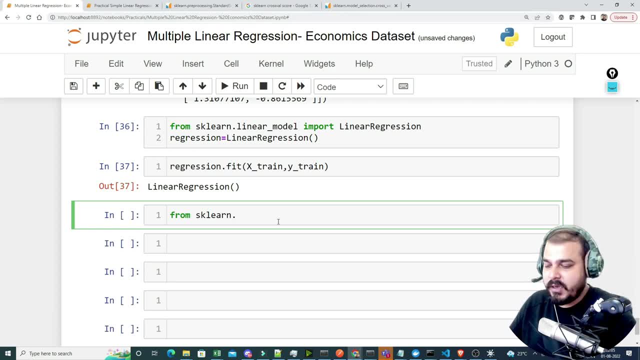 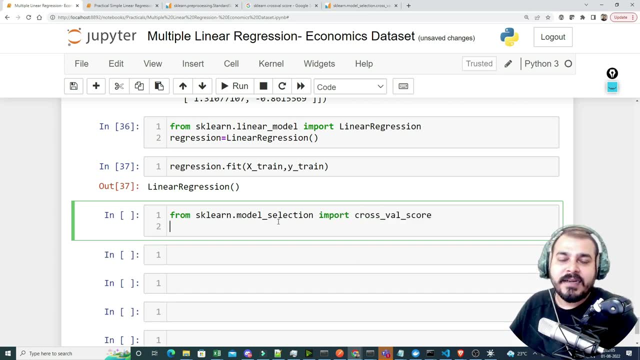 So if I say a scalar dot, let's see whether cross validation is falling. It falls in model selection And I'm going to import cross valve score. OK, now, inside this cross valve score, what I'm going to say is that, OK, fine. 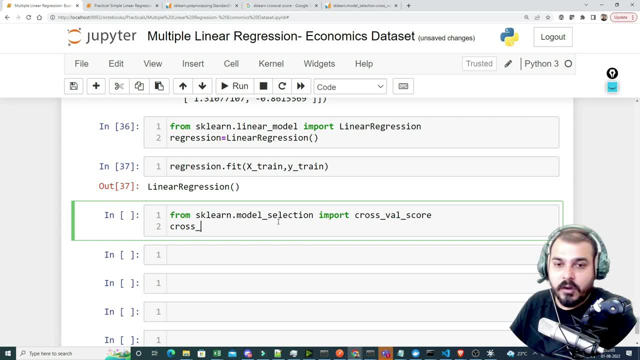 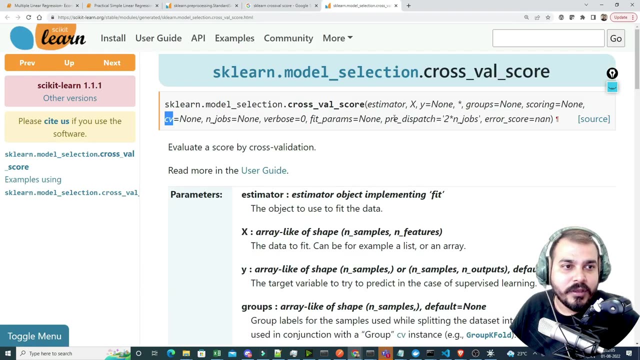 This will be my cross valve or cross, or let me say that this is my validation score. OK, This in turn. first of all, we will give this cross valve score over here, The data set that we are going to give. obviously, when I press shift tab, I have to give my estimator. 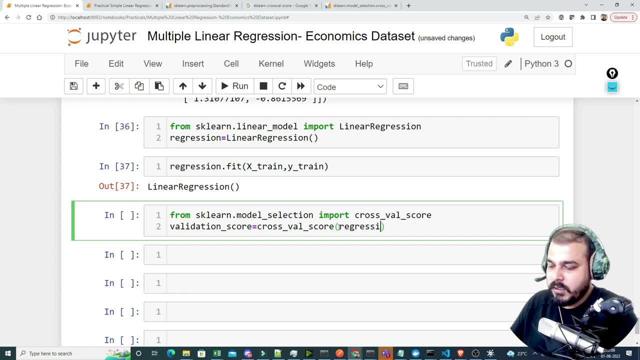 The estimator basically means my model. OK, so here I have got my model. And then in the next parameter, if I probably go and see I have to give my X and Y value, OK, so here obviously I will give my X train comma, Y underscore train. 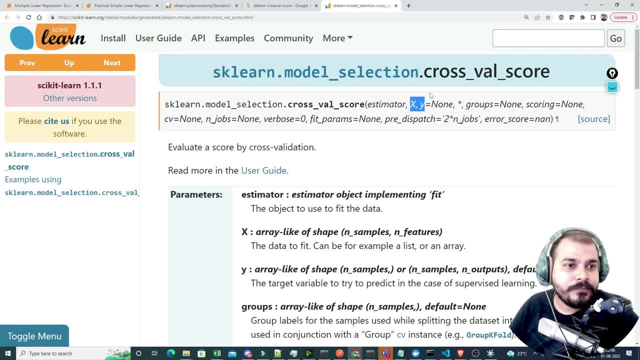 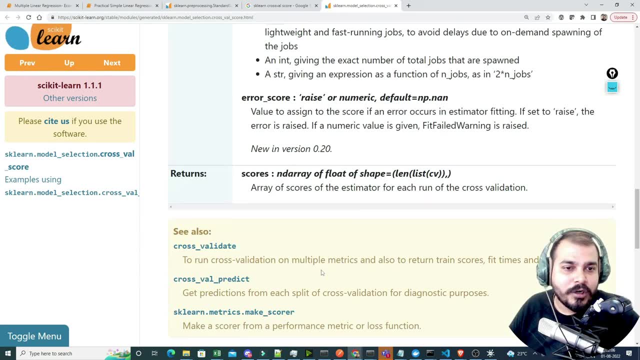 Perfect. The next parameter that I will probably give over here, if I see there is something called a scoring scoring parameter. Now, in this particular case, let's see what should be the scoring parameter. OK, so if you probably go, 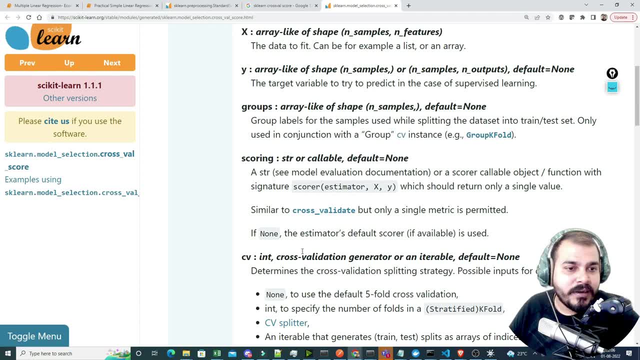 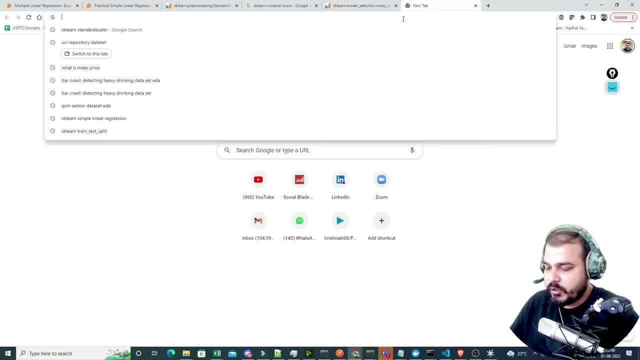 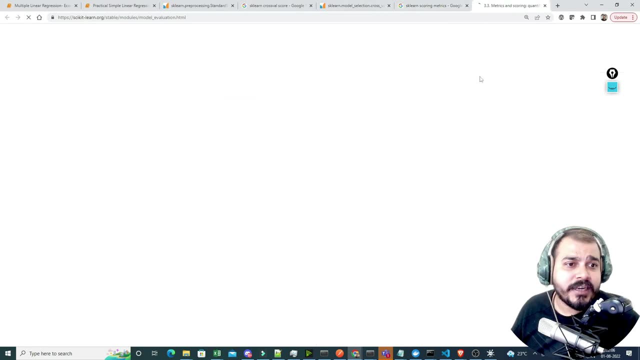 and see over here. similar to cross validate, but only a single metric is used. So if I probably see a scoring parameter in that, let's say I'm just going to search for a scalar scoring metrics. OK, now inside this, if I go and check it out, 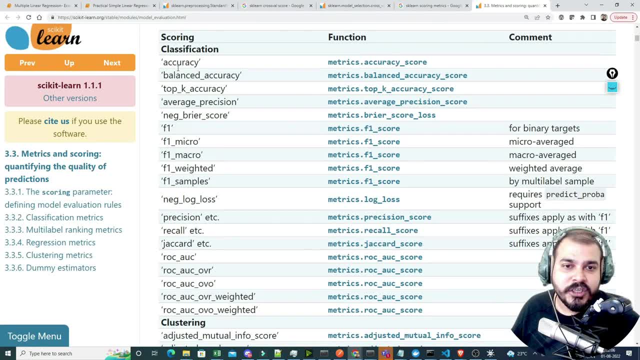 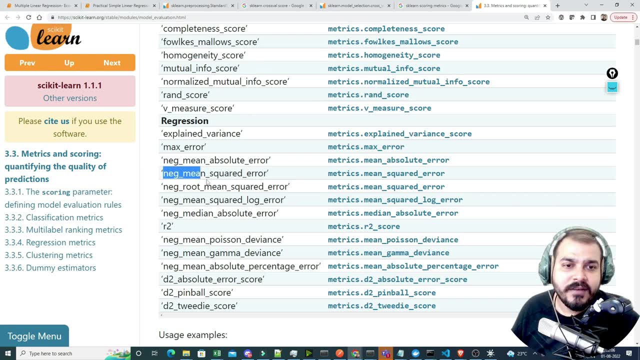 how many different types of scoring parameter are there? So, for classification, you have this many. for clustering, You have this many. for regression, You have this many. So let's say that I am just going to consider negative mean squared error. OK, negative mean squared error basically means I'm just going to get 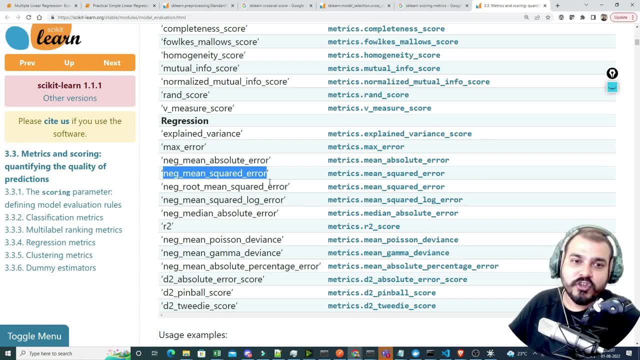 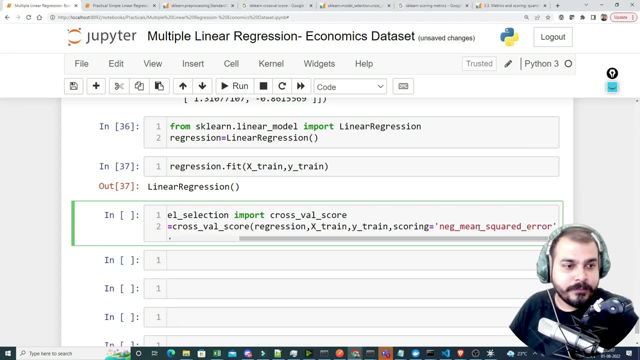 the mean squared error, but in a negative manner. OK, so I'm just going to copy this and put it over here. OK, this will be my scoring parameter. OK, so here I'm just going to paste it. Perfect, Now, this is done. 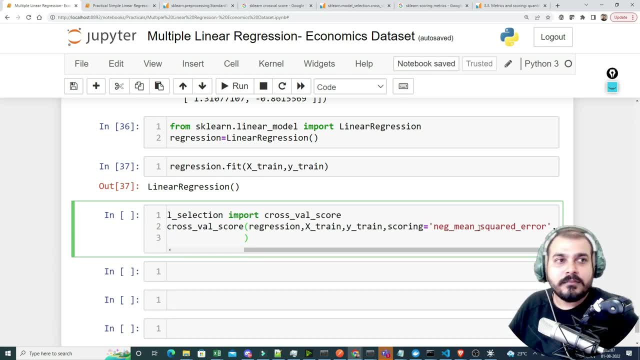 Now my next parameter, what I'm actually going to do if you go over here. the next parameter that is present with respect to cross val score is cross validation. Now, this is super important. If I see, my CV is five OK. 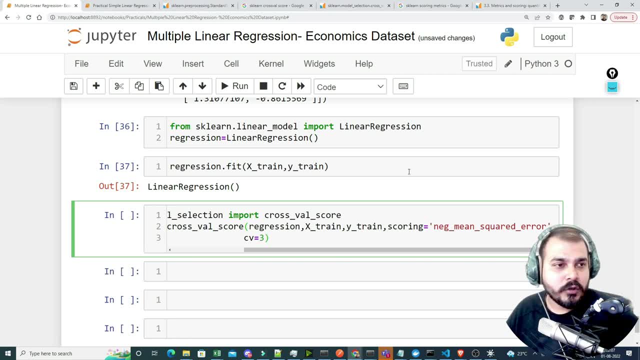 What does this basically mean? Well, let's say, I'm just going to make CV is equal to three. Let's say: If I have thousand records, total records, OK, OK now, initially, let's say: I made this as train test split. 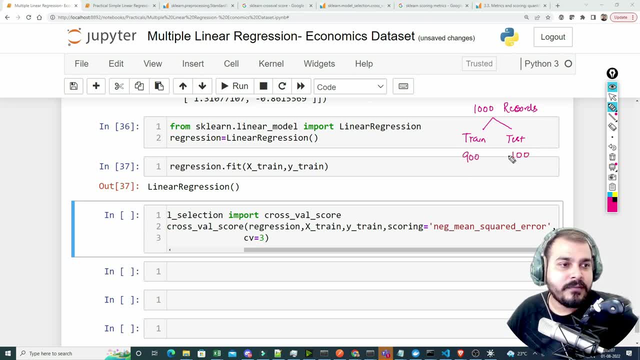 OK, let's say, in train I have nine hundred records and test I have 100 records. This data, I'm never going to use it, Right? I will just be using this data Now. this data will only be used when we need to test our model with the new data. 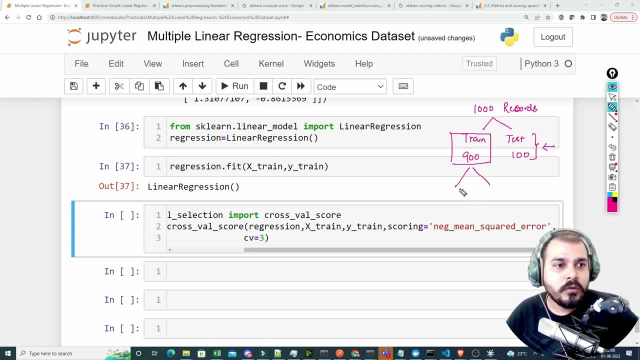 But further to hyperparameter, tune my model or to make my model better. you know I can split the strain data into train and validation. Now, when I split this data into train and validation, what will happen is that, let's say, I will split this based. 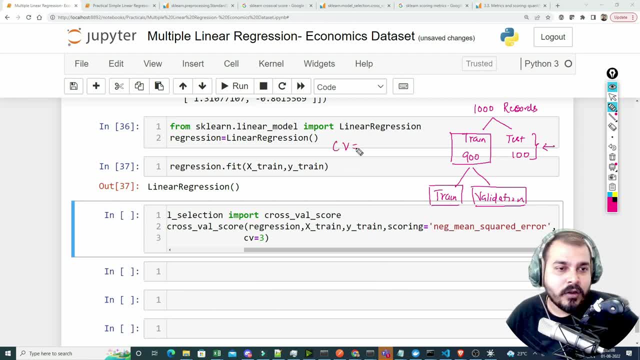 on some mechanism. what mechanism? I will say: let's go ahead and take cross validation as five. Now what will happen If I divide nine hundred by five? this basically indicates that what is the value that I'm going to get? Five ones are five, eights are 180.. Right? 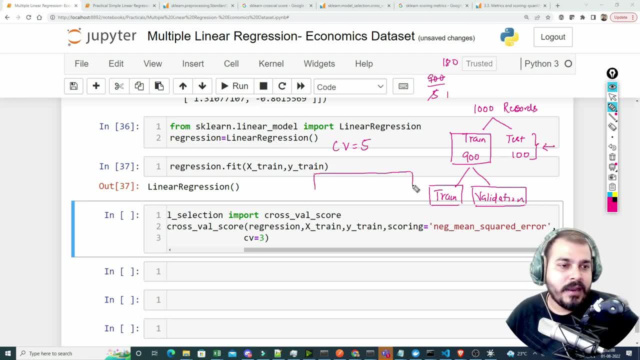 So this basically means in my first experiment, when I am taking my entire data set, the first 180 records will be my test data and remaining all will be my train data. Then in the second experiment, that is, cross validation is equal to two. 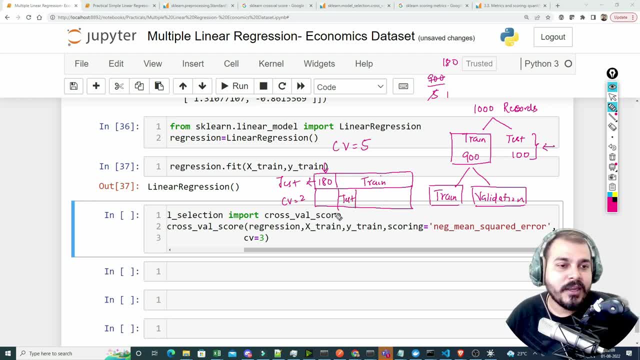 The next 180 record will be my test data and remaining all will be the training data. Similarly, I'll go, with respect to cross validation five The next- Sorry, Let me just do control Z- The next 180 record will be my test and remaining all will be the train. 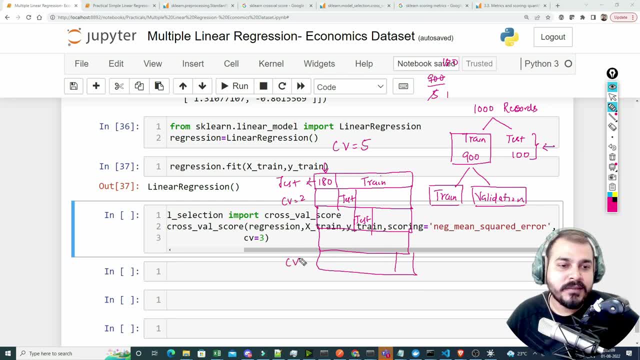 Similarly, I'll go like this And at the end of the day, we'll be able to see, at cross validation five. The last 180 records will be my train test and remaining all will be my train data. OK, now, as you know that, 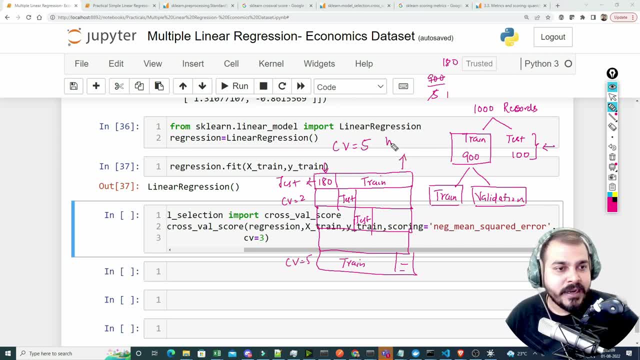 With this cross validation score, for every cross validation we will be getting a MSE. From where did this MSE come? This came from this particular scoring parameter. OK, so here we are going to use negative mean squared. That basically means, whatever MSE I'm getting, it will be a negative value. 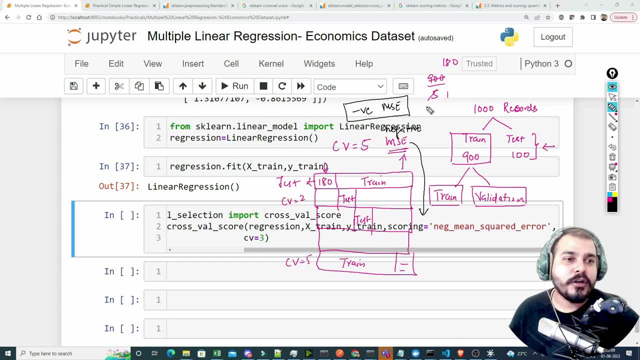 OK, negative value. So this is what we are going to do And again, our target is that it should be. the more this value comes towards zero, the more better the specific model is. So here, with the help of cross validation, I will be getting five different accuracies. 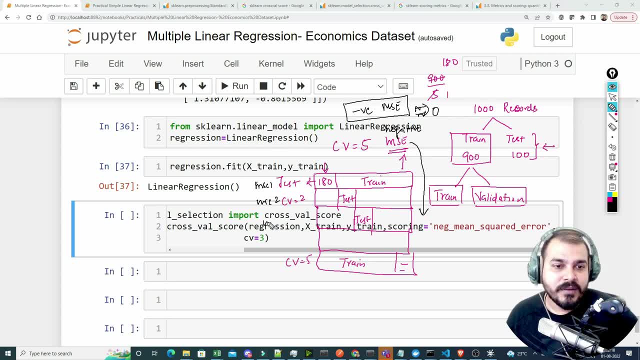 This will be my MSE one, MSE two, MSE three, MSE four, MSE five, And then I can probably take the average of all this and probably print it over here. OK, so this is what we are going to do over here. 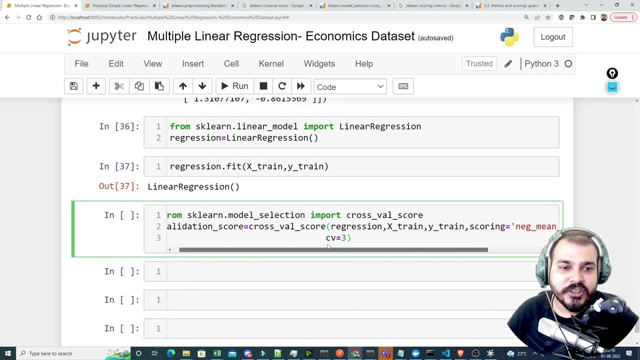 So let me just go and show it to you. Right now- I've just taken cross- validation is equal to five. That basically means I'm going to get three validation scores. OK, so let me just execute it. And this has got executed. 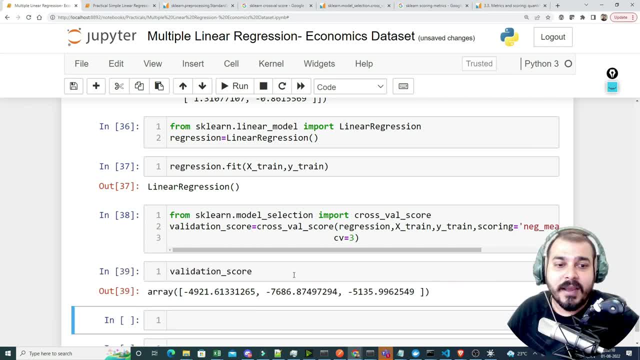 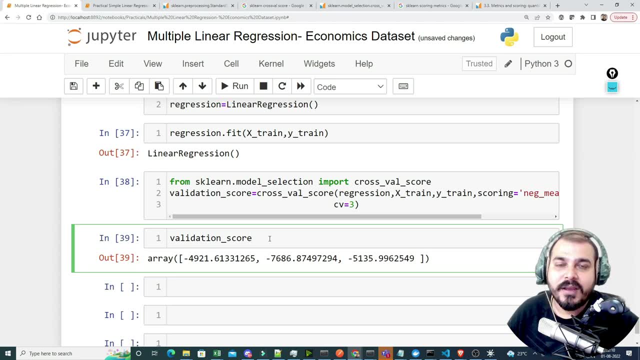 Let me go and probably see my validation underscore score. Here I'm getting three MSE values mean squared error values. And now, if I probably do the average of this, how do I find out the average of this? You can basically do npmean right, npmean. 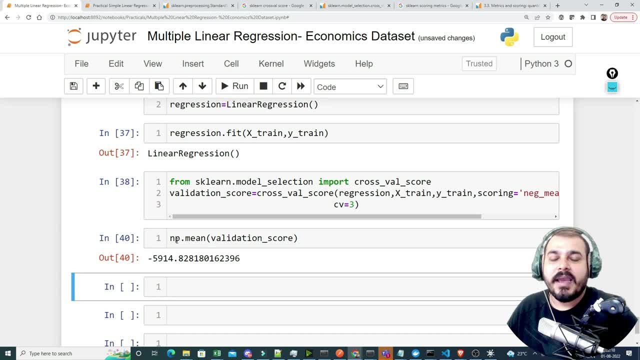 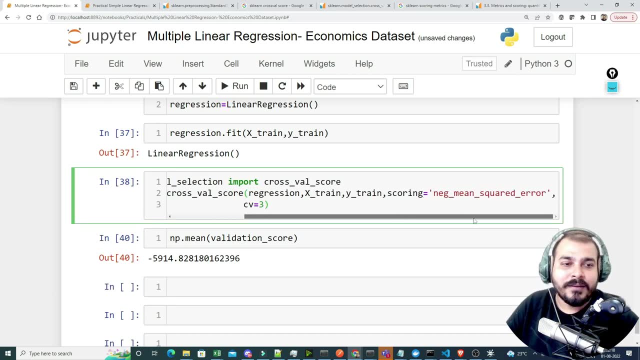 So by this way you'll be able to get the mean MSE. OK, so this is basically my mean validation score by performing all my basically cross validation on this particular data set. OK, but again, this is just to check or to do additional step of cross validation. 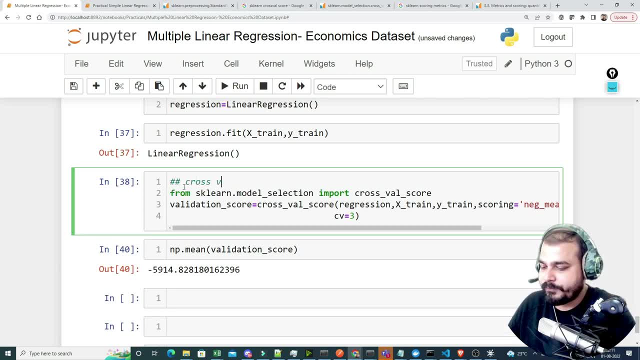 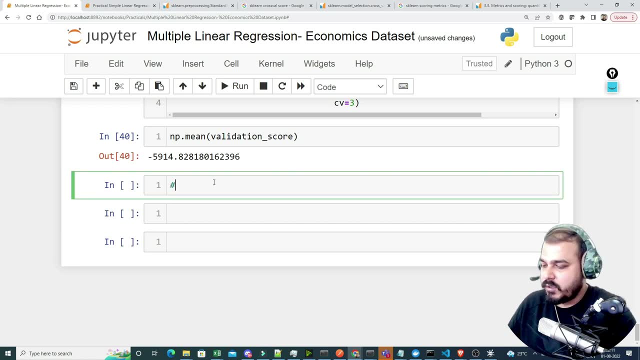 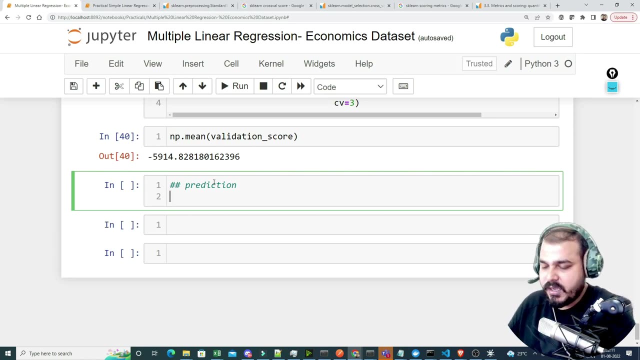 So here, this is how you have to basically do the cross validation. OK, with the model that we have created. But now let's go and do the prediction. So now I will do the prediction. OK, now, before we do the prediction, I also want to make some assumptions. 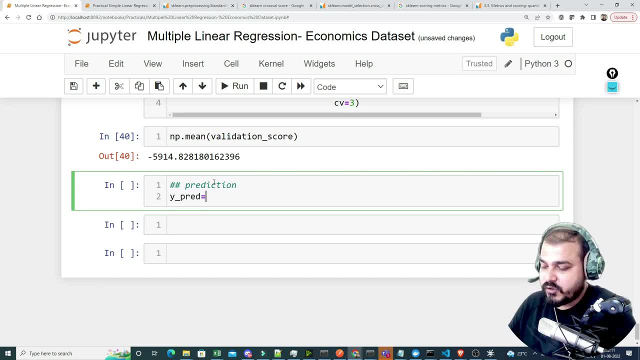 OK, and this assumption is super important. But before that let me do the prediction. So here I will be using the regression dot predict, and here I'm just going to give my X underscore test data And this will basically be my Y pred right. 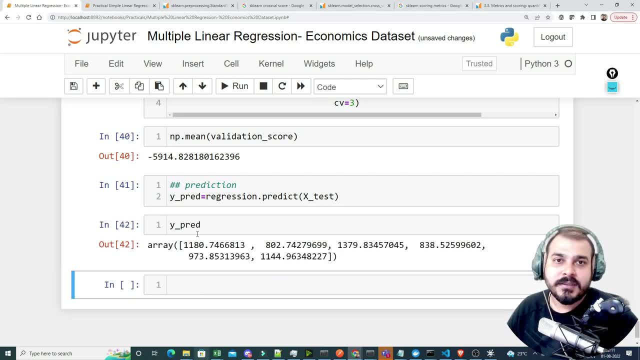 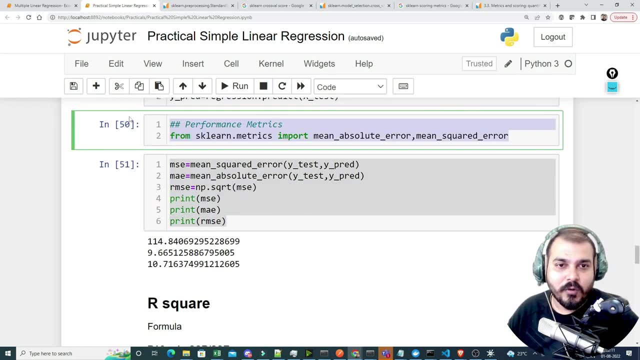 So Y underscore pred Perfect Now, after this, all the things that are common, right? So first thing, I'm just going to go ahead with this entire code, that is, performance metrics, and I'm just going to copy it over here. 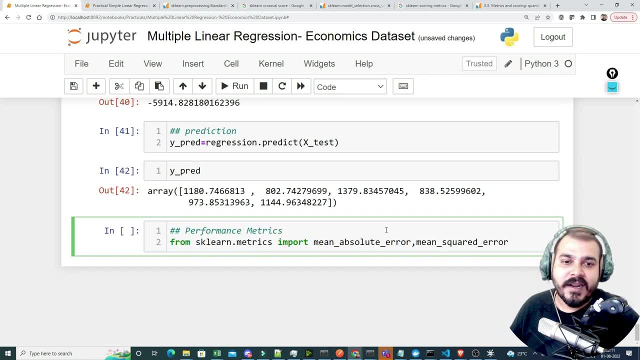 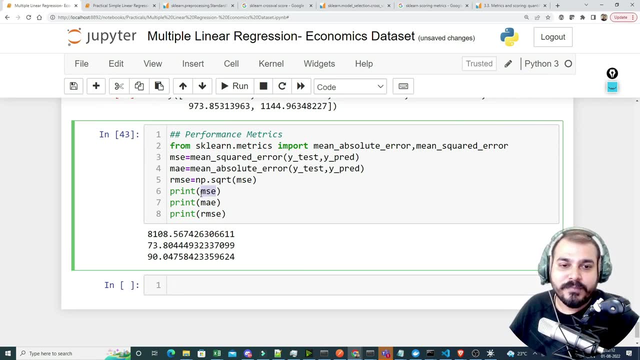 And similarly, I will go ahead and copy this, where I'll be finding the mean squared error and all, And here I this is where I've actually printed. So this is my mean squared error with respect to the prediction data And this is my mean absolute error with respect to the prediction data and RMSE. 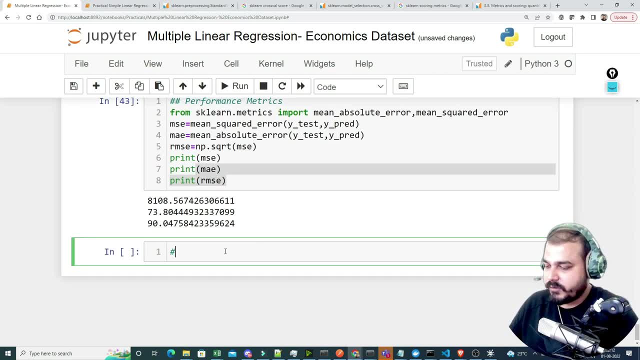 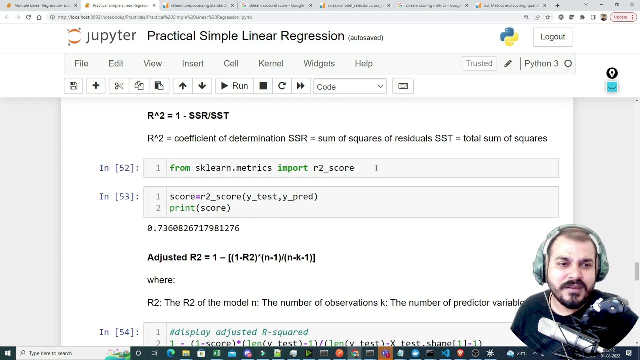 This is fine. right Now, let's start with some assumptions, Assumptions. but before this, let me also print the R-square and adjusted R-square Right. So here is my code. See, guys, I'm just doing along with you. 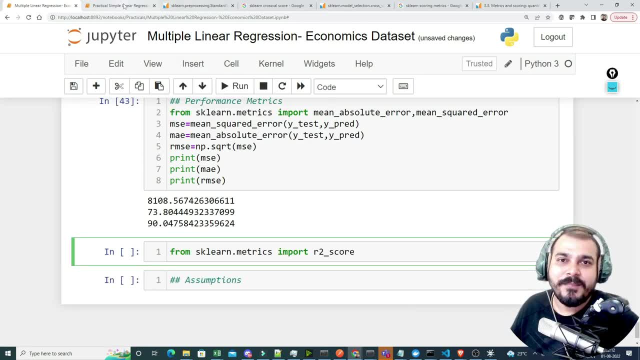 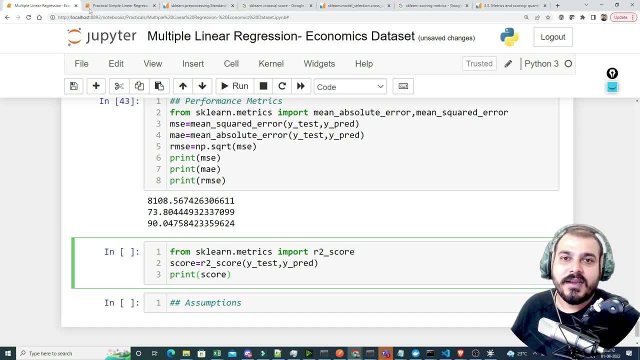 Please make sure that you also do it and you also practice. So this is my R-square And, similarly, I will go and copy this my print R-square And after that I will also go ahead and print this specific value, Right? So this is my adjusted R-square, right? 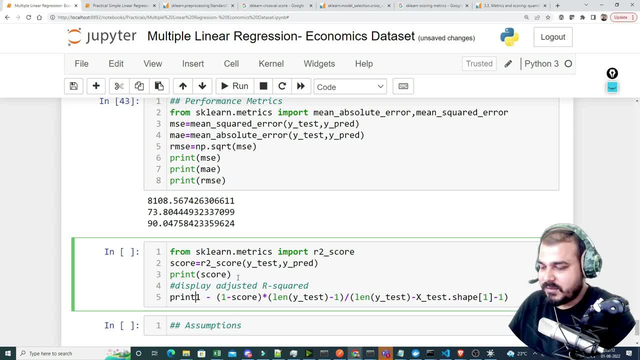 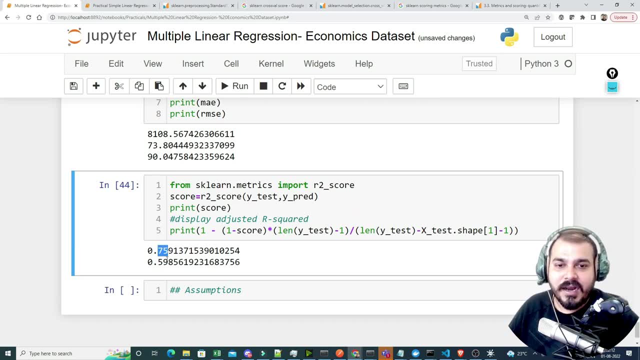 So here This part also, I'm going to print it. Now let's execute here you can see 75 percent I'm actually getting it as R-square and 59 percent I'm getting. is that adjusted R-square? OK, And obviously adjusted R-square will be later. 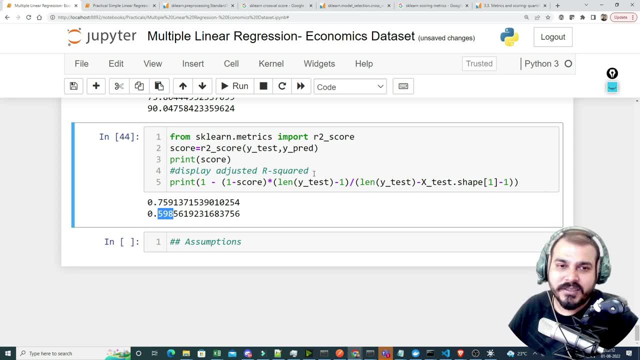 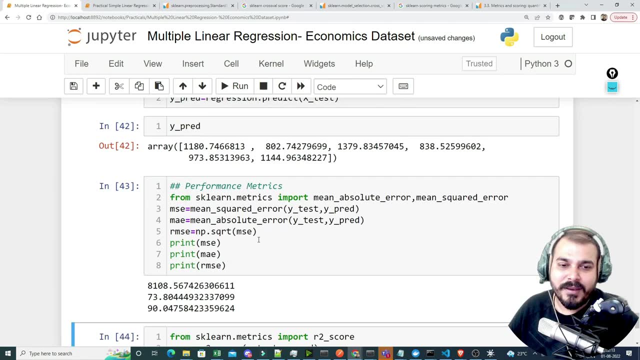 But I'm going to do a little bit less when compared to this. OK, But this is with respect to the test data, to just see that how my model is performing well or not. OK, But again, I just have small number of data points. 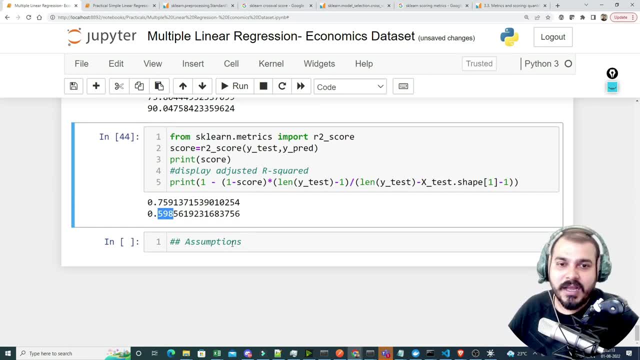 So I'm able to get this. If you have more data points, if you have more dimensions, at that point of time, you know we also have to check how the data is performing well or not. Now let's go ahead and let's learn something new. 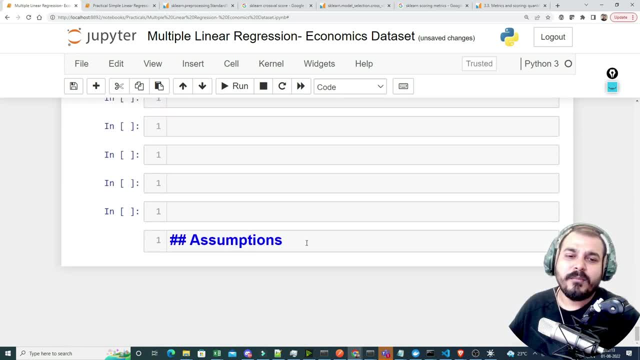 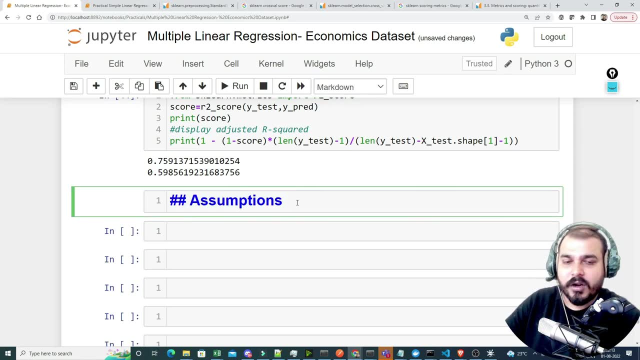 These are the assumptions like. finally, I should be able to find out whether my model is performing well or not, And by seeing these assumptions we can definitely come to a conclusion that my model will definitely perform well. So the first assumptions, after we do the prediction right. 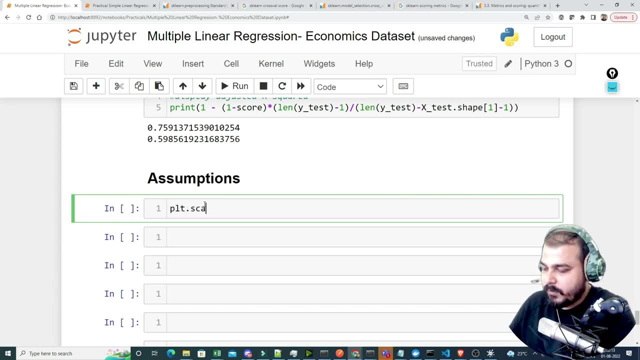 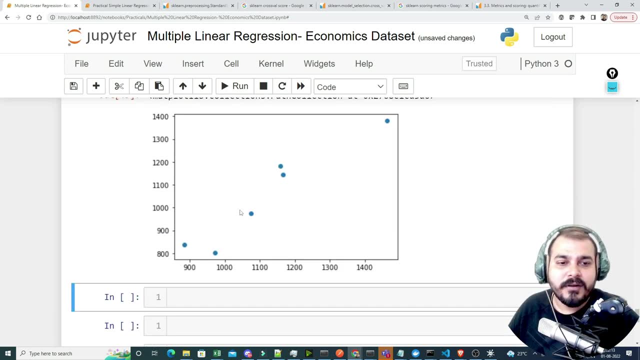 The first assumption is that I will just go ahead and plot my scatter plot And I will say here: I'm just going to give my y-test comma y-pred. Now, if I execute this here, you'll be able to see that they will be following some. 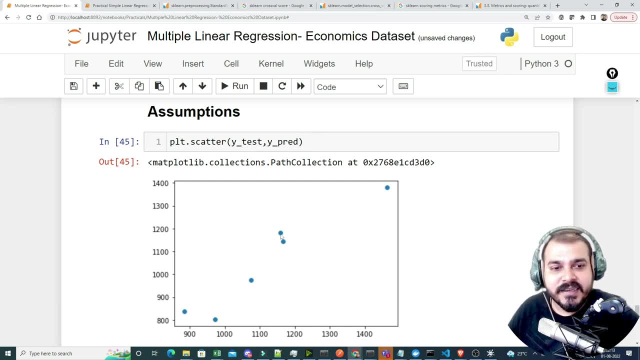 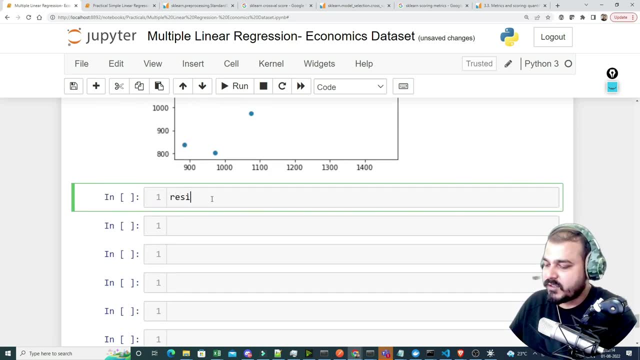 some relationship here between the y-test and y-pred. if there is a linear relationship, that basically means your model has performed well. OK, now the next thing that I'm going to do is that, with respect to residuals, let's go ahead and calculate the residuals or the errors between y-test and y-pred. 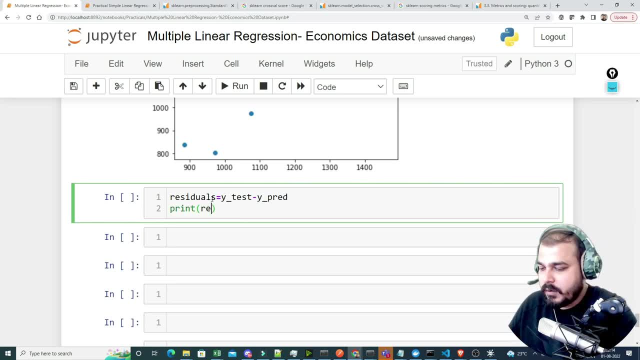 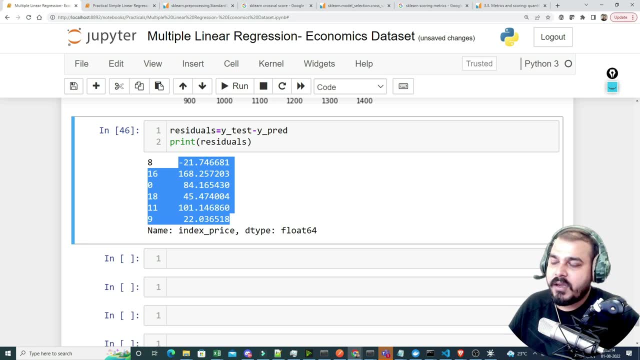 If I take up this residuals- OK, the residuals here- you'll be able to see I will be getting these errors right. These are my errors that I'm actually getting Now if I plot these residuals, if I plot these residuals with the help of this plot, 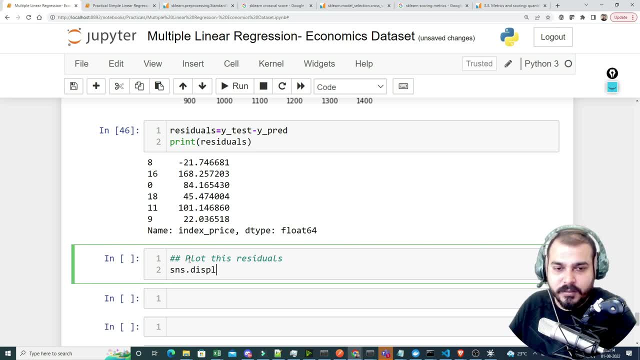 let's say, how do we write this plot? snhdisplot. it is basically present in cbomb And if I probably write residuals over here, and the kind of plot that I'm going to take is something called a KDE plot, that is, kernel density estimator. 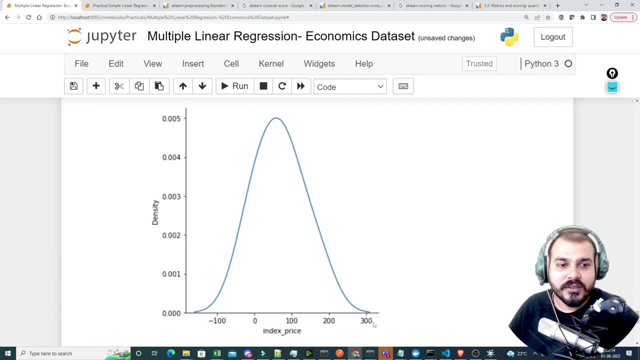 And if I execute it here, you'll be able to get something called as a linear normal distribution. So if this kind of curve is basically coming, that basically means yes, the model that you have created is good. OK, and one final thing. 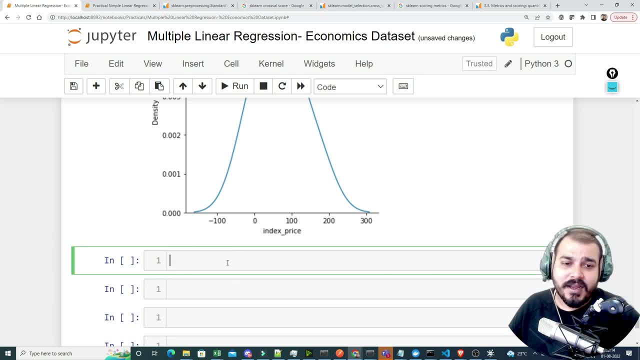 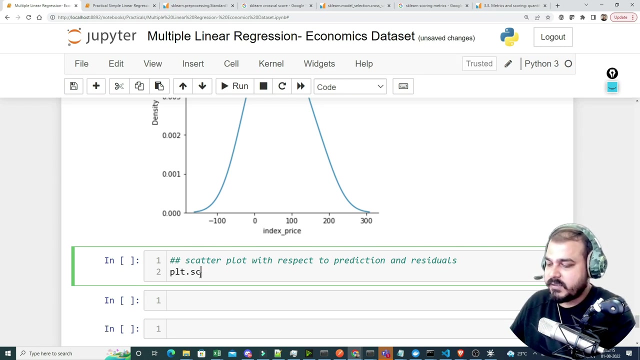 that we have to probably take with respect to assumptions is that let's create a scatter plot With respect to Predictions and residuals. So if I probably create this plot with residuals and predictions, you'll also be able to see some observation. OK, so what I'll write as a pltscatter with 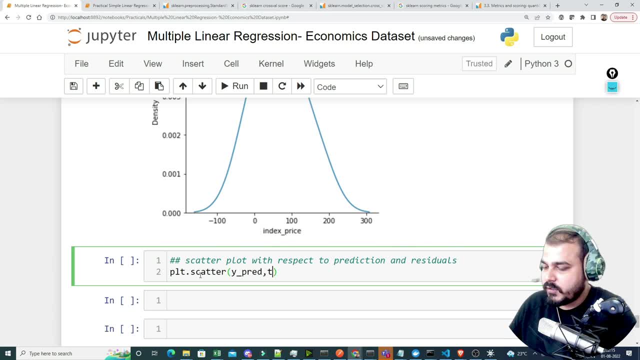 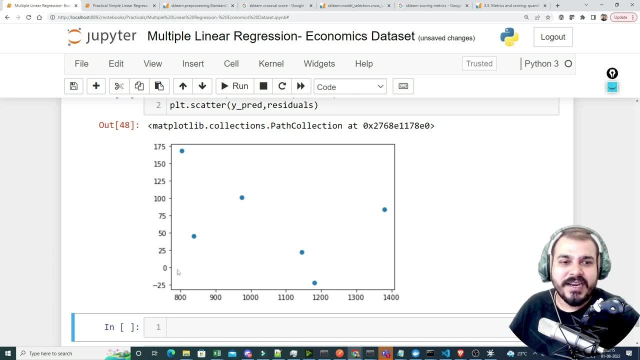 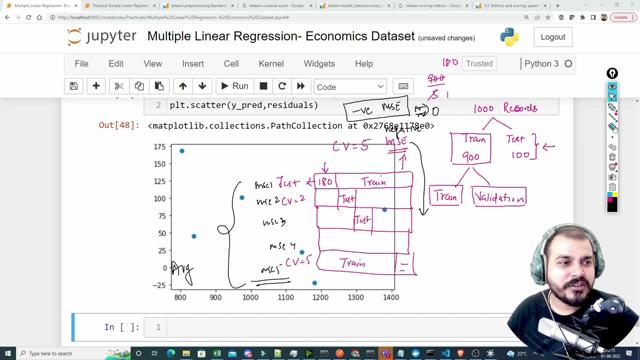 y-pred comma residuals. Here you'll be able to see That. Follow any pattern. see, this data is uniformly distributed. OK, now you may be thinking, Krish, the data is very less Now why you are saying it is uniformly distributed. 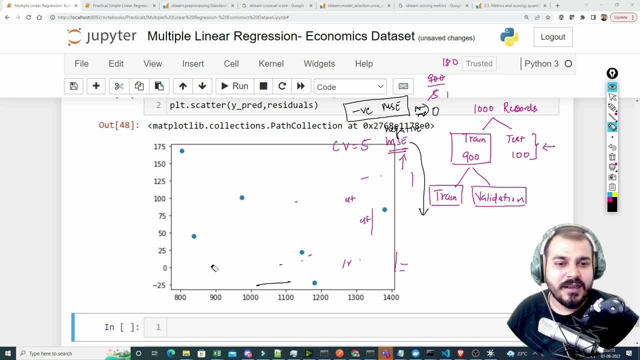 First of all, let me remove this. OK, everything will make sense. Uniformly distributed basically means data is distributed everywhere You know it does not follow any patterns as such. Here also, you cannot see any patterns When we'll be taking huge data. 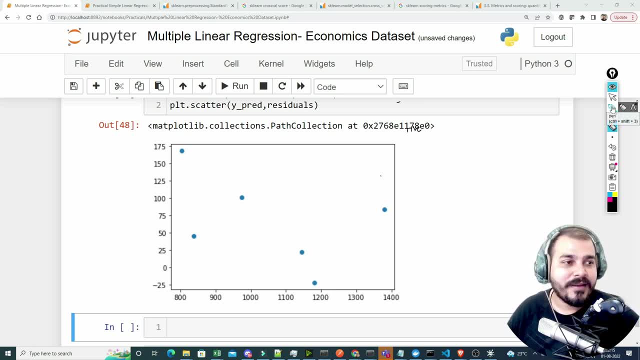 set. in going forward, you know we'll be doing some projects which will be having many data points. you'll be seeing that this data sets points will be something like this: So this is uniformly distributed. It does not follow some patterns. If I say some patterns, it may follow something like this: 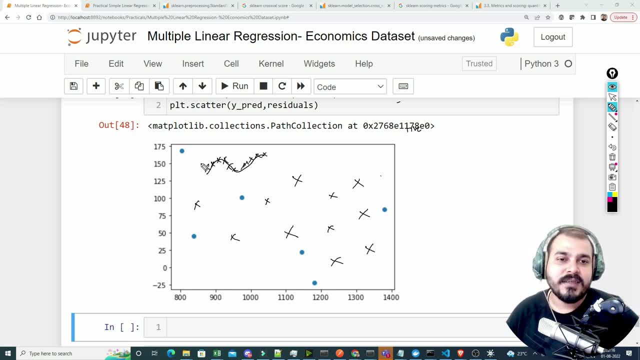 OK, it may follow this kind of pattern. If it follows this kind of pattern, that basically something is wrong. OK, something. But if it follows this uniform distribution, we can definitely come to a conclusion that there is no such problem as such. 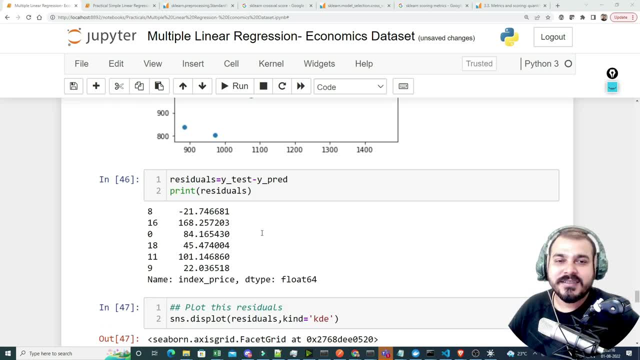 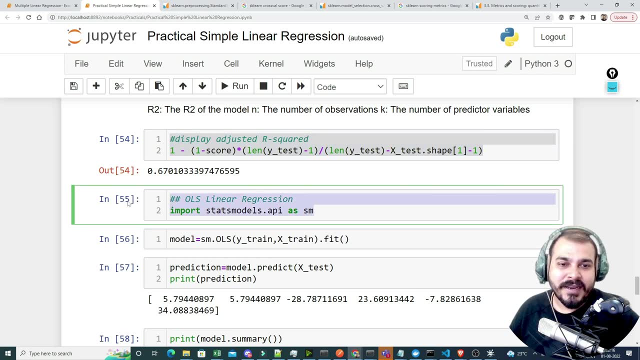 OK, so, yes, most of the thing we have covered in Now. final thing is that obviously we need to compute the OLS. that is ordinary least square. So again, I'm going to copy this entire thing, copy the Y-train and X-train part and do the fit. 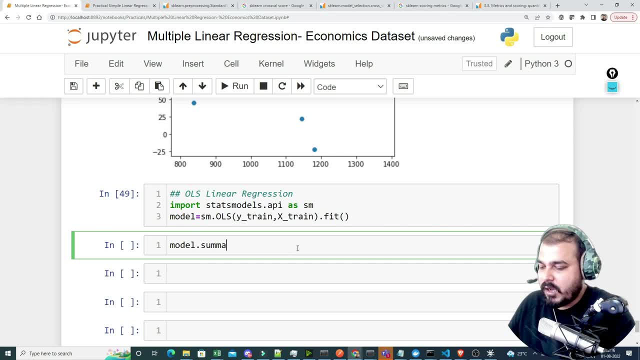 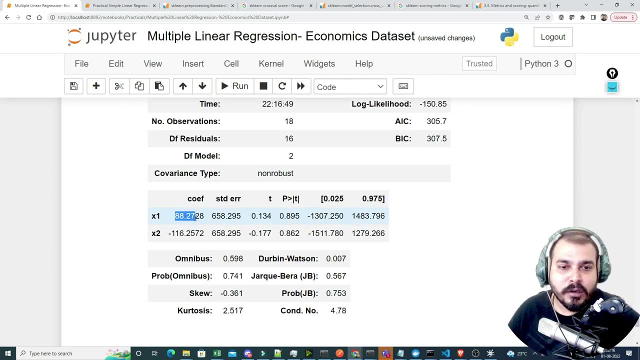 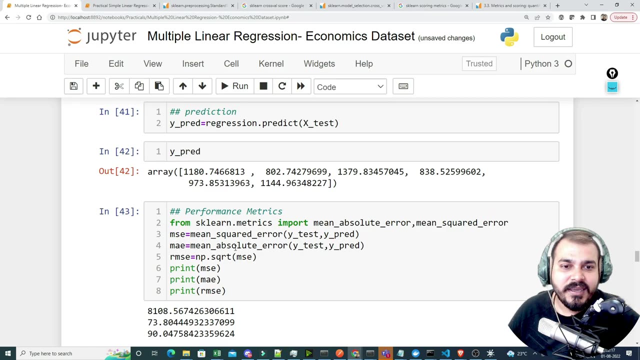 And once I execute it and if I see modelsummary now, our main thing is basically to check whether are we getting the coefficients almost similar. So coefficient over here is 88.2728 and 116.2572.. So are we getting that similar kind of coefficients?